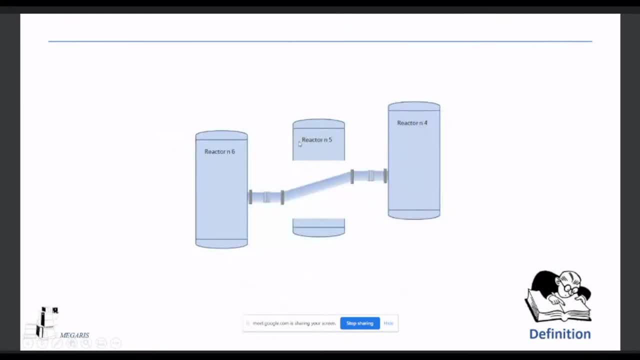 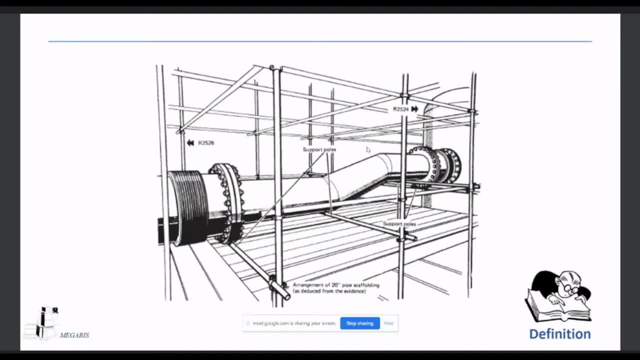 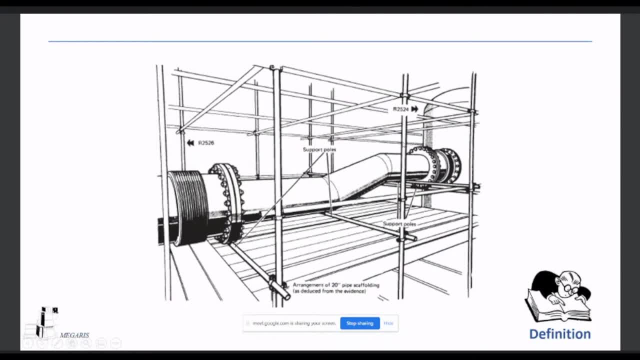 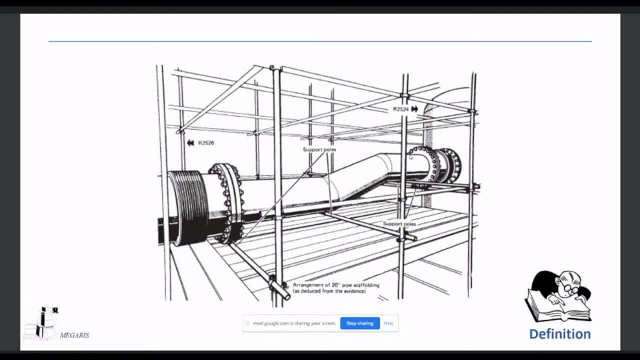 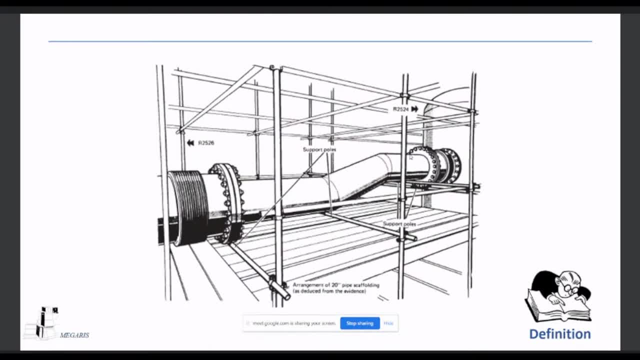 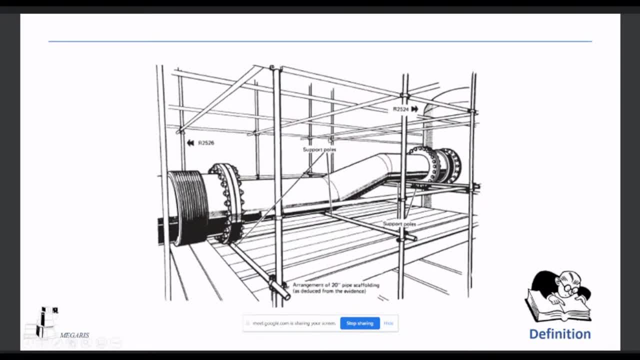 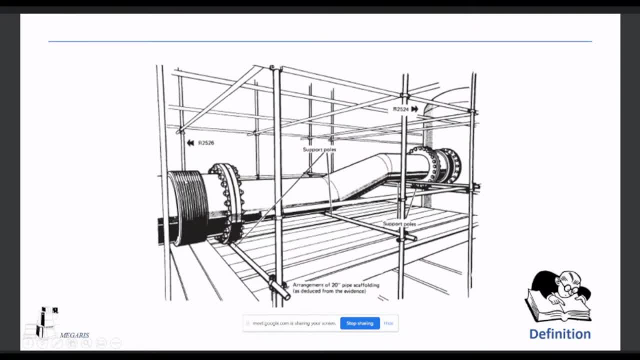 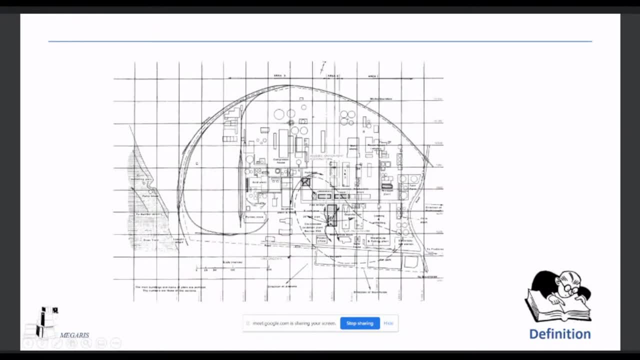 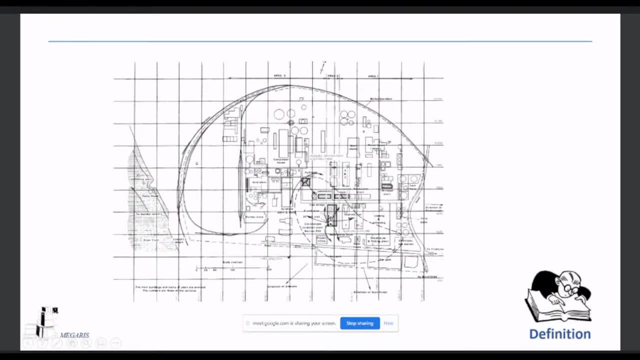 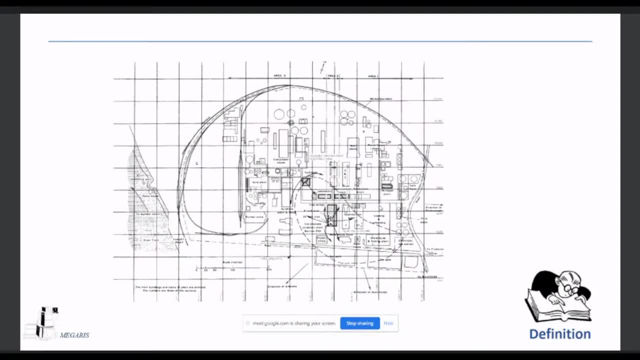 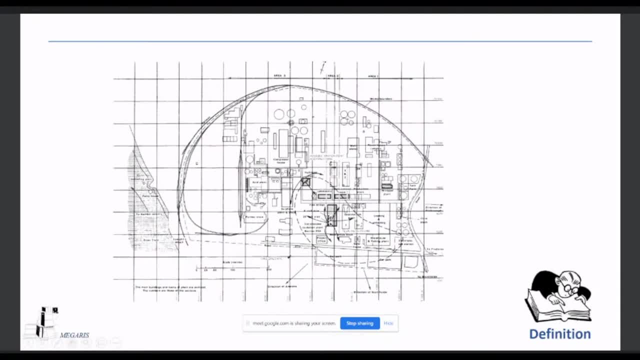 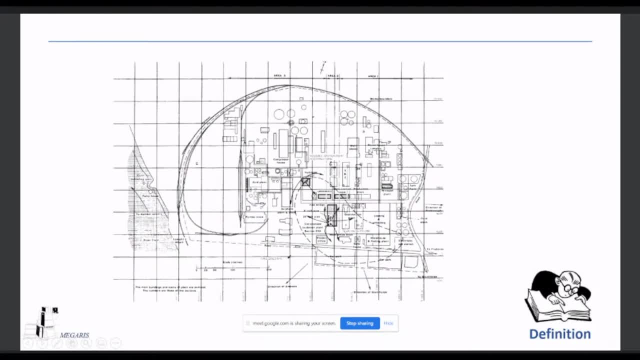 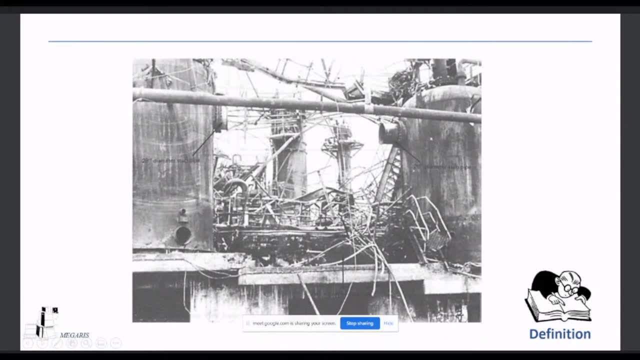 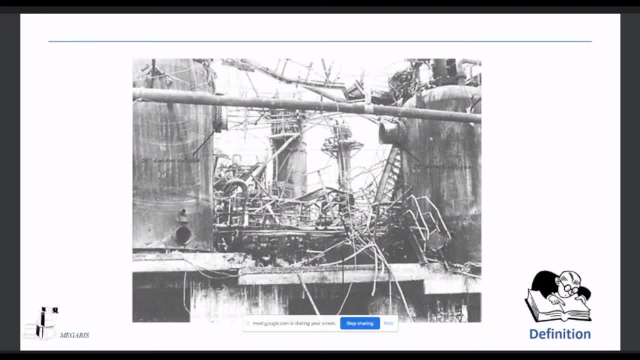 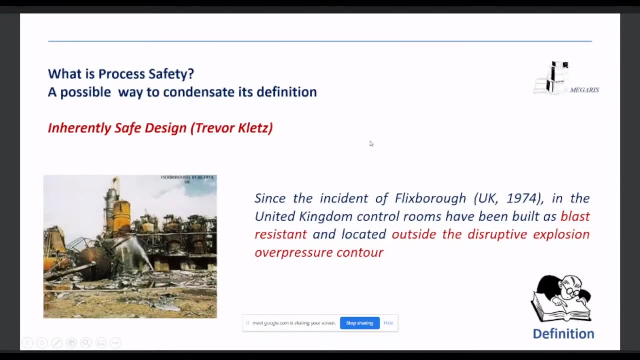 were just related to inorganic chemistry. So after two years, as you probably know, in Europe, in Italy, we had the Seveso incident and after that we had some regulations that were essentially introduced in the international regulation Since the incident of Vicksboro in the United Kingdom. 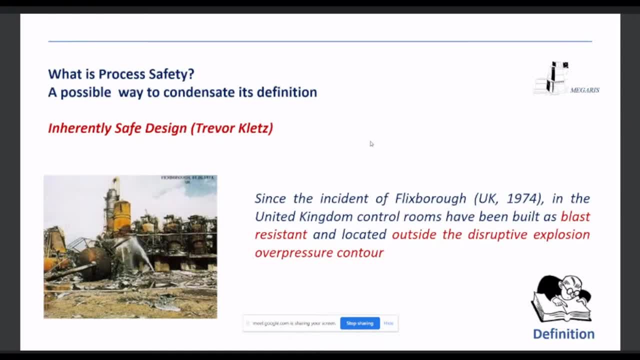 control rooms have been built as blast-resistant and located outside the disruptive explosion over pressure control. We- probably in the UK we- anticipated the introduction of severe and serious rules like this Probably, Probably, much, much earlier than in the rest of Europe. 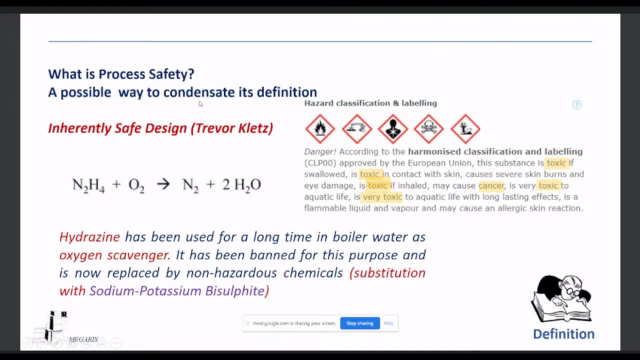 Okay, So what, practically speaking, what do we mean with inherently safe design Until 15,, 20 years ago, in order to reduce oxygen concentration in the boiled water? so you know boiled water, we have a blood arm, So we have to feed the boiled water with new, essentially new, demi-water. 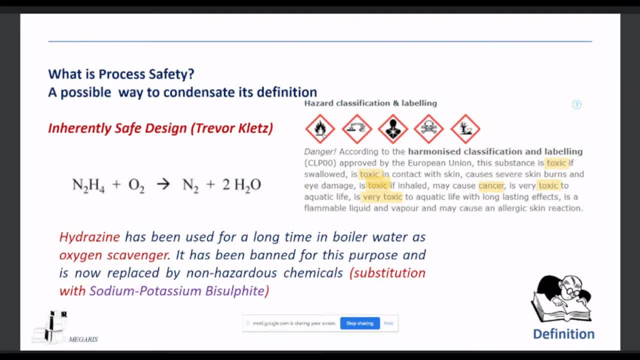 And you know that oxygen is essentially just a corrosion promoter, So we have to keep the oxygen concentration. Until 20 years ago more or less- I remember because I worked as a process engineer in this field- hydrazine was added to water. 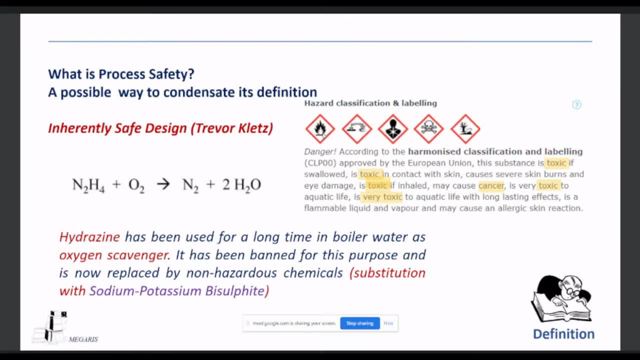 And I remember- I remember personally, but hydrazine was used for a long time in boiled water as an oxygen scavenger. It's been completely banned Because essentially, as you know, this is the CLP regulation that is in Europe, is the regulation that is used for classification, labeling and packaging. 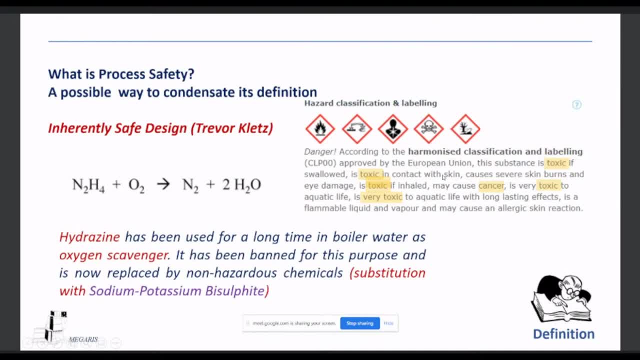 And it's toxic, it's toxic, it's toxic in contact with skin and so on. So this is essentially an example of one of the first pillar of the inherently safe design: replacement, substitution Today in order to essentially to achieve the same target. 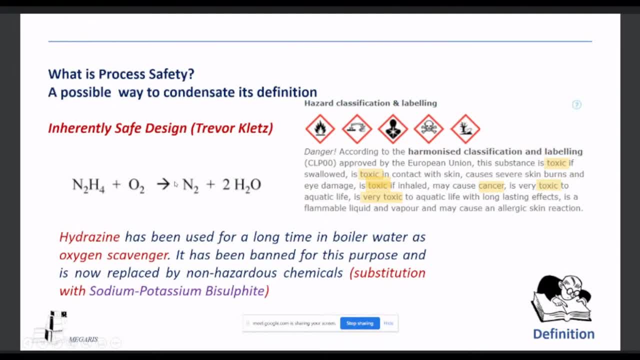 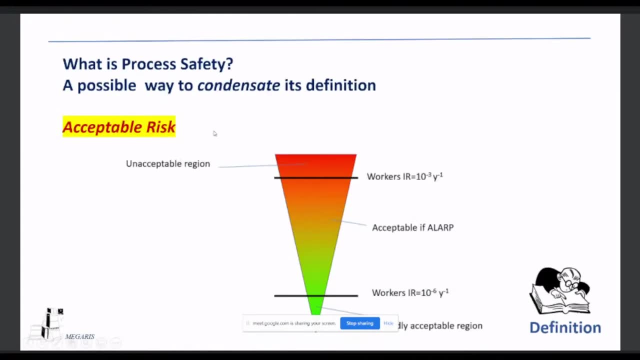 we add sodium or potassium pisophate, So it is inherently safe because there is no longer a toxic chemical in the water. This is a way to comply with inherently safe design rules by Trevor Prince. Okay, the second, the second, the second keyword to identify process safety is acceptable risk. 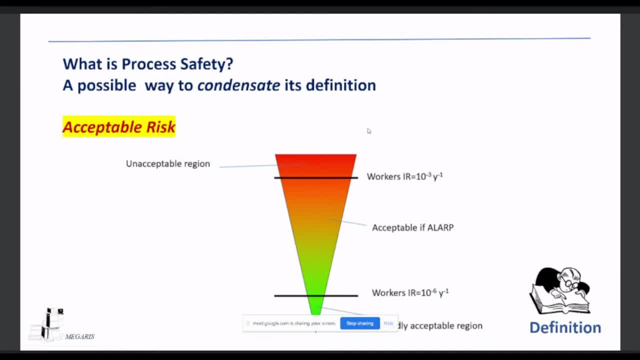 Okay, acceptable risk is not an easy, an immediate concept, because we know that unfortunately we have to pay something to risk we cannot reduce. there is no, essentially no risk zero in our, in our, in our project, in our design. So we have essentially to accept some risk. 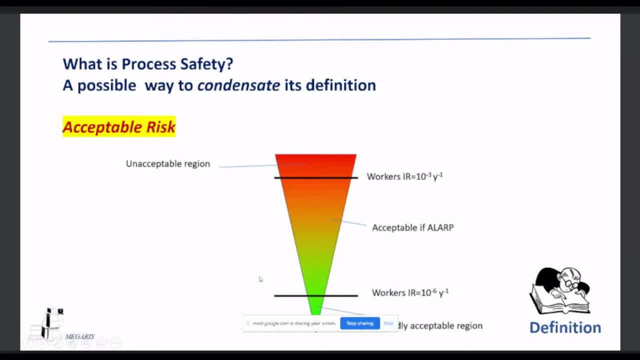 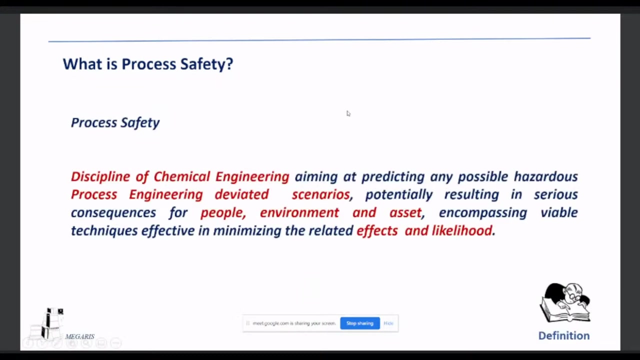 So acceptable, acceptable risk. we can see here the UK ALARP diagram that is internationally, internationally adapted and accepted as probably the most effective, just in order to to identify a validated acceptable risk criteria. So acceptable risk is a second Keyword. So just to conclude this first tile, this first, let's say, building block of the definition: 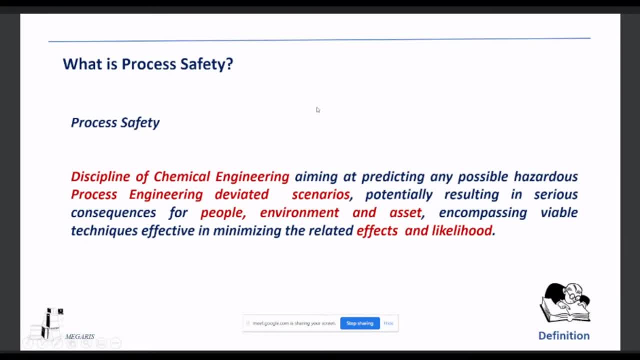 we can say that the process safety can be maybe identified as a discipline of chemical engineering or of course also other in other. but I'm a chemical engineer So I have a chance to how to promote chemical engineering. I may get predicting and possible. 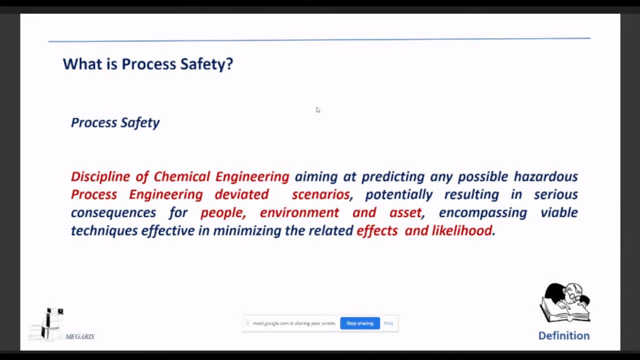 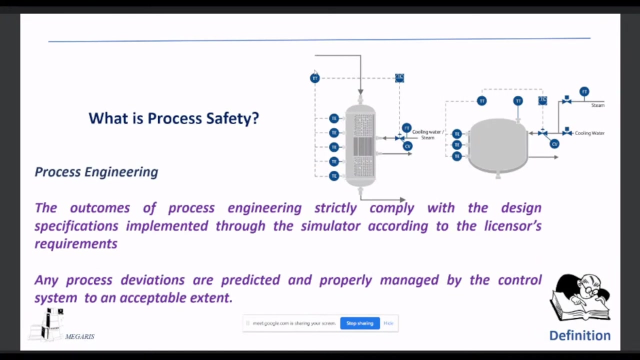 any possible hazardous process engineering deviating scenarios potentially resulting in serious consequences for people, environment and asset. encompassing, viable, technically effective in minimizing the related effects and the likelihood. I think this definition could work, maybe. Okay. why is the process safety different from other disciplines? 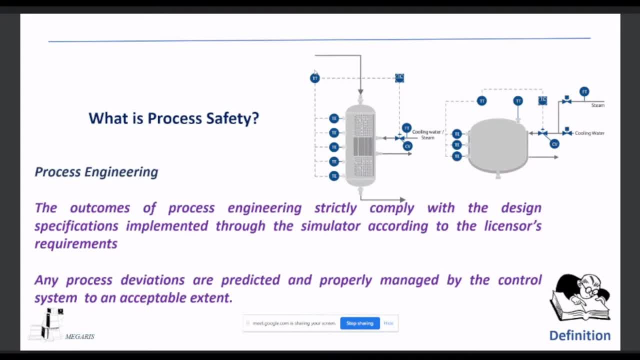 And what is the relationship between process safety and process engineering? Okay, in my experience- and I probably think you can, you can agree with me- I think process safety is somehow. I think process safety is somehow just a daughter of process engineering or a system. 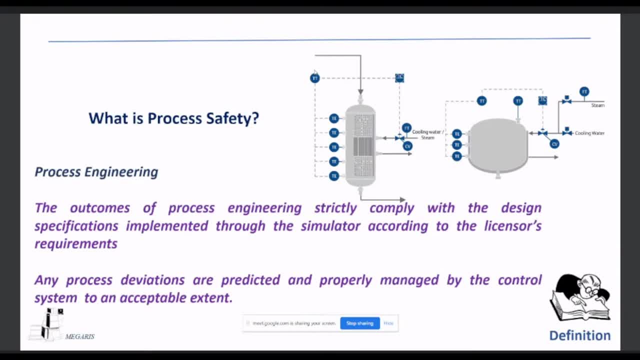 We know that outcomes of process engineering strictly comply with the design specification implemented through the simulator- no ISIS, for example. according to the license or requirements, Any process deviations are predicted and properly managed by the control system to an acceptable state. When you, when we essentially carry out an answer, study: okay, we can, we can discover that there are some deviations. 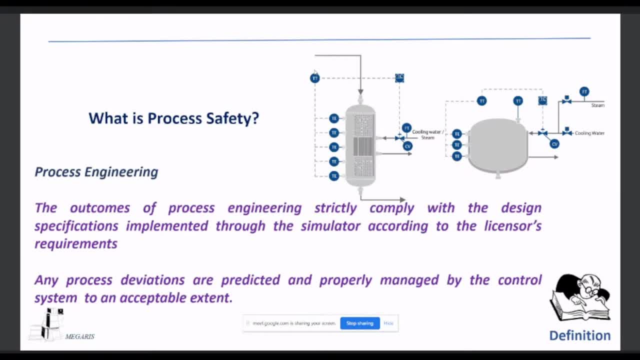 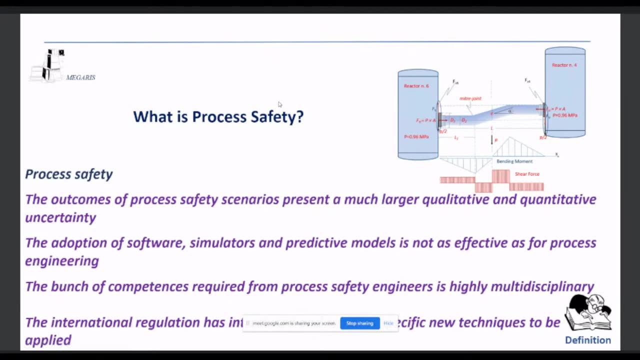 But in reality if we have just a Soletion column, it's not likely to You can have a huge departure from the design specification. This is process engineering, process safety. In my experience I can- I can recognize ultra process efficiency scenario presently much larger qualitative and quantitative uncertainty. 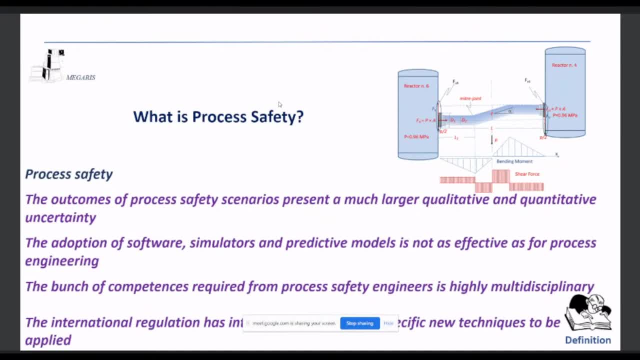 The adoption of software Simulator predictive model. any kind of additional tool is not as effective. as for process engineering, The benchmark competence is required for process process safety from process safety engineers is highly multidisciplinary and the international regulation is essentially a way just to to essentially require specific new techniques. 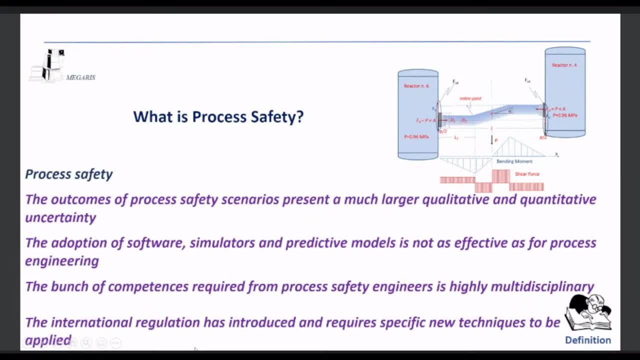 to be applied. international regulation is not secondary in the definition, because we have seen in the last i i would say from the seveso direct directive introduction that in reality, uh, probably the the contribution and the challenge of the international regulation and i would say the european regulation. we can, we could dedicate just a kind of specific discussion about the relationship. 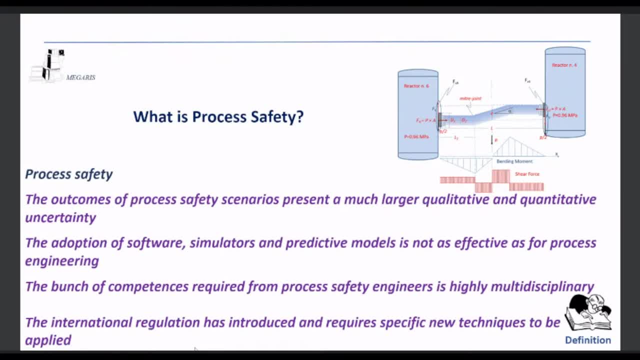 between the european and european. european regulation is is a strongly systemic, is holistic, whereas the american regulation has been predictive and and additional. okay, so atx, for example, we will discuss about it. so the international regulation has been a forcing, terrible, huge, uh, let's say, promoting factor for processing, so we can see that process safety is somehow. 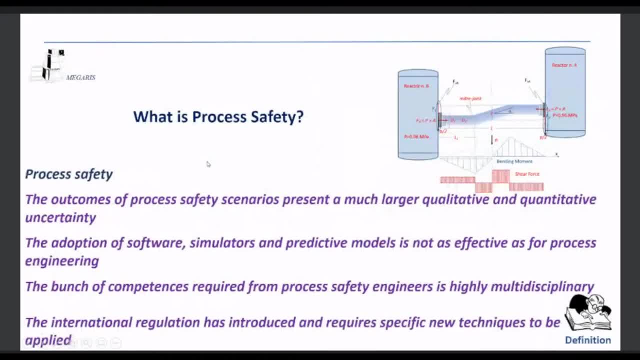 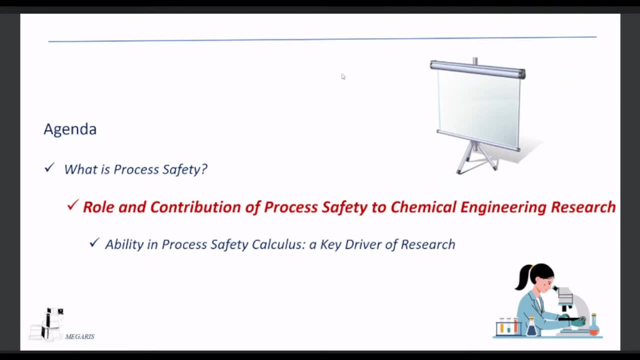 different process for process engineering. uh, the spread of competencies, the threat of knowledge is probably larger. it's difficult to say this is a scenario. this is possibly the scenario we could say: okay, so the second, the second question, the second subject is: what is the role, a contribution of a process safety to chemical engineering research? that is a 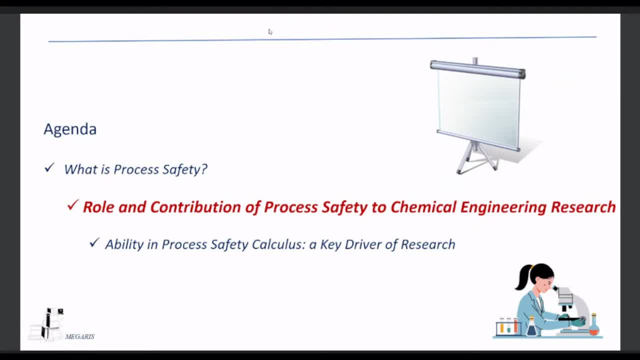 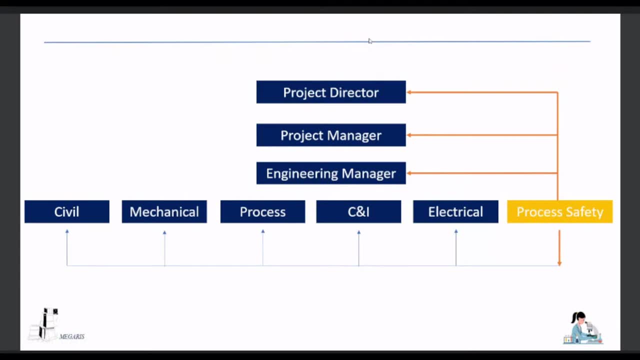 potentially subject that savio has just put on the carpet. okay, in order to cope with this specific subject, we have to consider: what is the organization chart of a, a project? we can see just just a summary of the of the specific specific areas. uh, we can recognize. we have a project director, we have a. 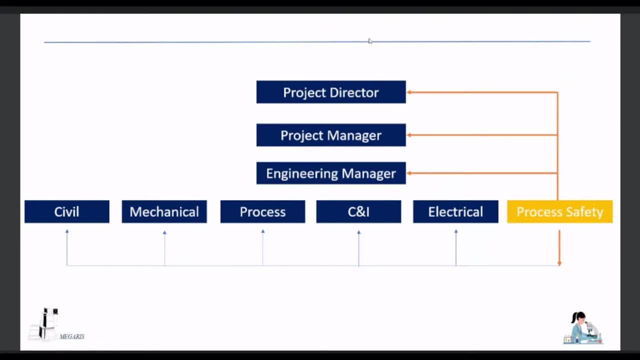 project manager, we have an engineering manager and we have some disciplines. What is the particularity? Why is the process safety engineer role so particular? As you can see, I've tried just to identify some specific relationship between these roles, also using a different color. 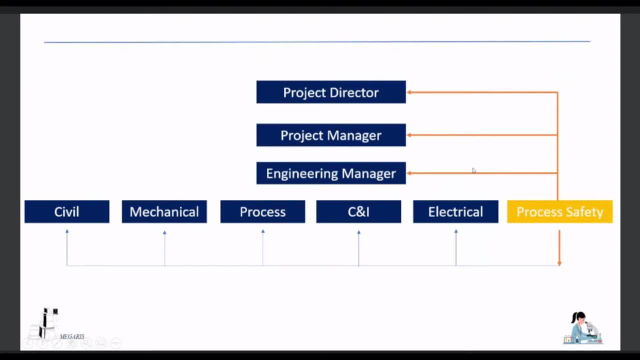 In my experience and from the legal point of view, we can say that process safety, okay, all the disciplines report to the engineering manager. It's unlikely, even if it is not completely possible, that a mechanical engineer, civil engineer, process engineer 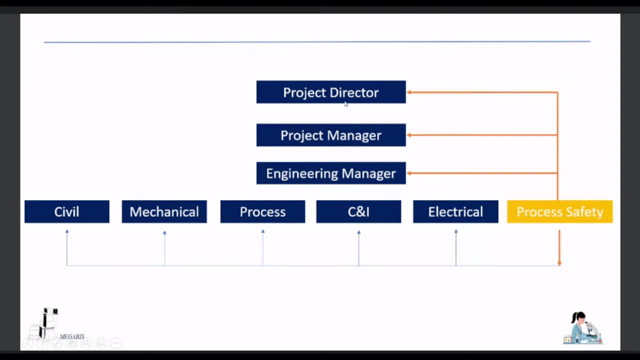 talk directly to the project manager or to the project director, But the process safety, the role of process safety is very particular because we are dealing with people, assets and environment. So the process safety has the capacity, the ability and also somehow the power to, in addition, to discuss directly. 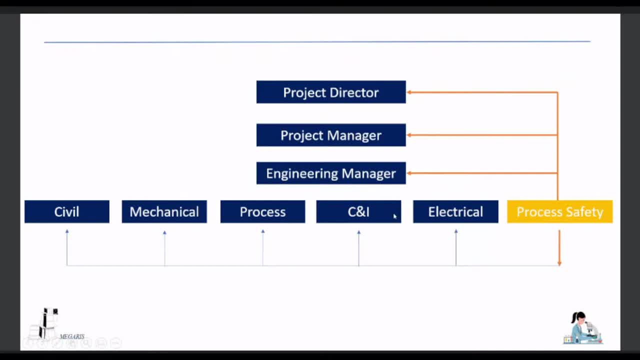 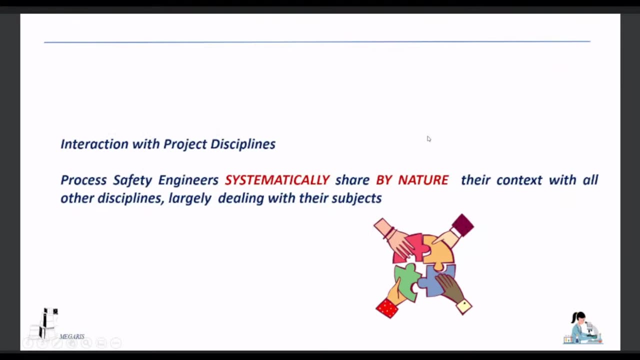 with the other discipline. Okay, In a meeting or just in the relationship of the task, also directly with the project manager from some specific aspect of process safety engineering, and also with the project director, This happens. We can say that process safety engineers systematically share. 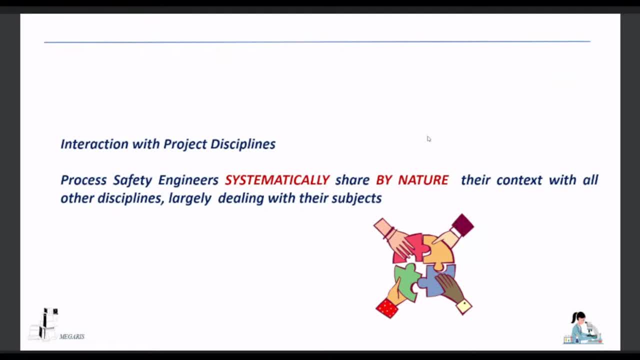 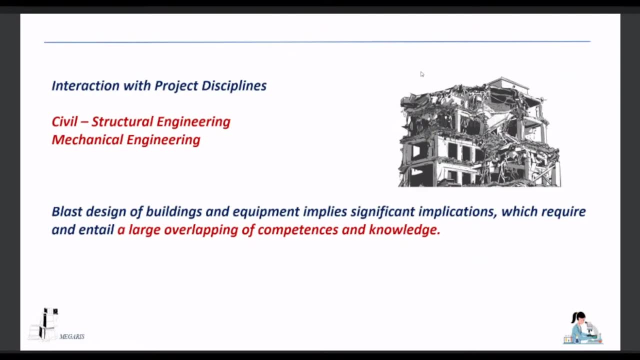 by nature their context with all the other disciplines largely dealing with their subject. We can have some example. I have been working in my latest EPC contract in Middle East for seven years with civil engineering working about blast the buildings. 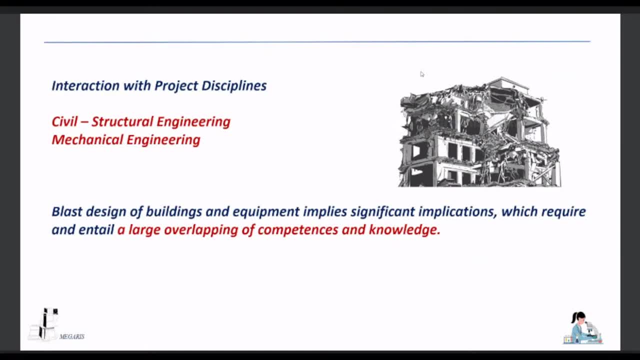 So competencies must be really large. Blast design of buildings and equipment implies significant implications which require and entail a large overlapping of competencies and knowledge. We can see here this is the result of explosion. We must be able to understand and to have the same wording of civil engineering. 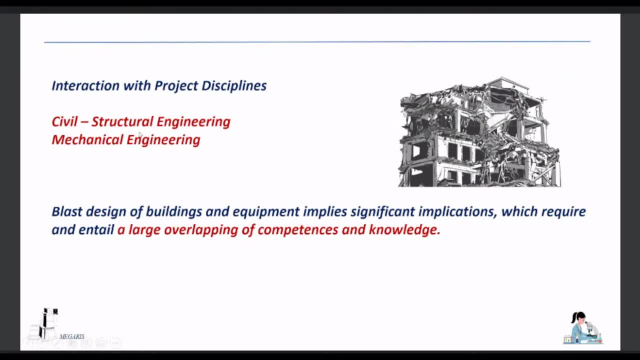 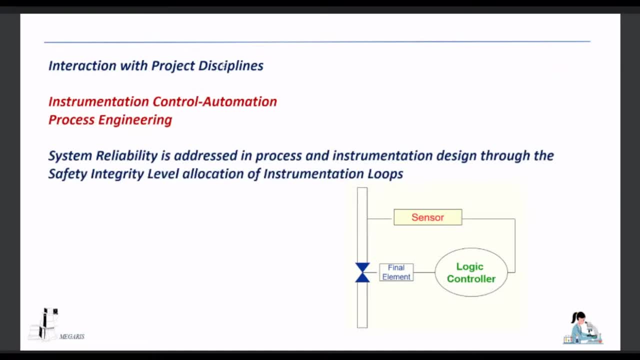 because civil engineering competence, of course, is large but is related to the process, It is related to their specific discipline. So you have to be familiar with some additional concept. We must be familiar also with instrumentation. You know that now functional safety is one of the most important. let's say 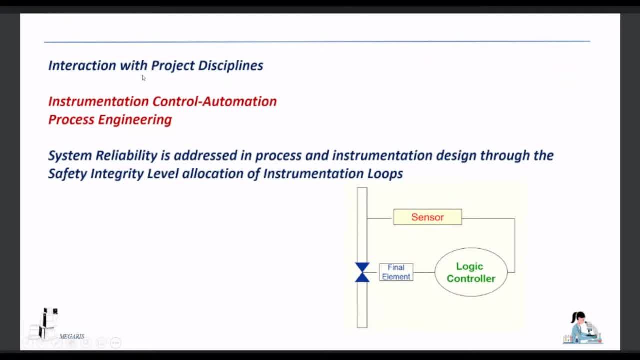 most important subject that we face in the project. So we must understand what does system reliability means? It is addressing the process of instrumentation design to the safety integrity level- allocation of instrumentation loops. But we must understand that the process of instrumentation design is not just. 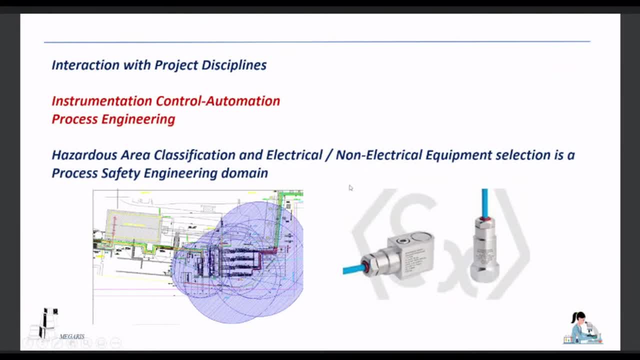 to the safety integrity level, allocation of instrumentation loops. We also have to discuss in terms of the legal and the regulatory implication, also with electrical engineer and in Europe also non-electrical equipment. so mechanical engineer, After the classification electrical and electrical is a process safety engineering duty. 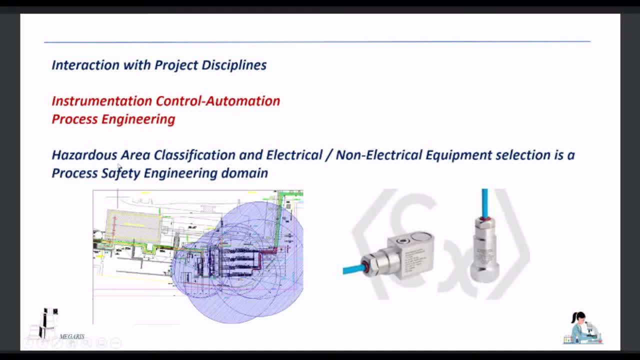 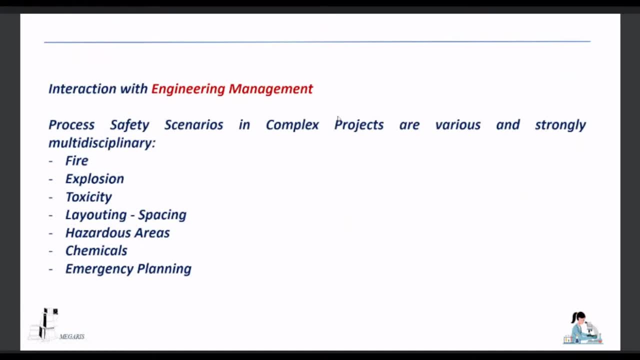 So we can see also about this. we discuss with the process engineer, we discuss with instrumentation and control, automation, people. So in reality, process safety scenarios in complex projects. complex projects are various and are strongly multidisciplinary. So we essentially deal with fire, with explosion, with toxicity. 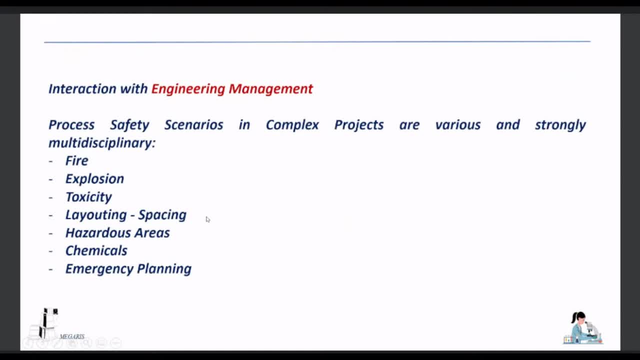 with blasts of structural engineering, layouting and spacing. so the layout, hazardous areas, chemicals and emergency planning. So this can probably identify the range of the concept and the knowledge that we have to manage in order to be effective in a project like this. 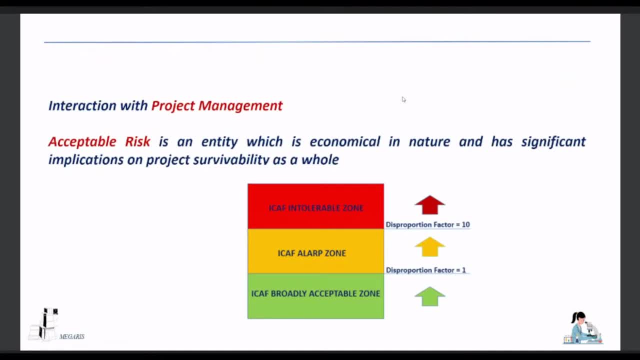 Last but not least is also the relationship with the manager, Why in the previous slide, I decided to relate the process safety engineer with project management. As you know, the project engineering, the engineering manager, is essentially related to the technical role and technical tasks where the project manager is the registered office. 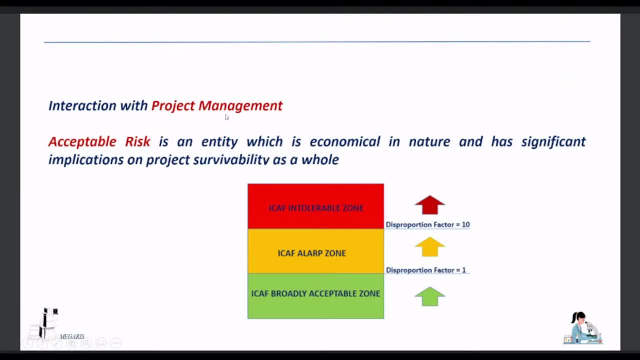 of the cost of the project, The ALARP. so the, let's say, acceptable risk implication that we have discussed before implies some cost-related aspects. This is not trivial because in reality, unfortunately, when we have to decide essentially if and when risk is acceptable, 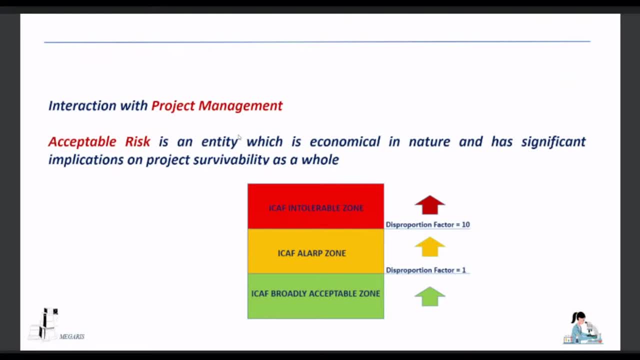 we have to consider that it is essentially, let's say, an economical exercise. So we have to discuss with the project manager, So we have to consider that it is essentially, let's say, an economical exercise. So we have to consider that it is essentially, let's say, an economical exercise. 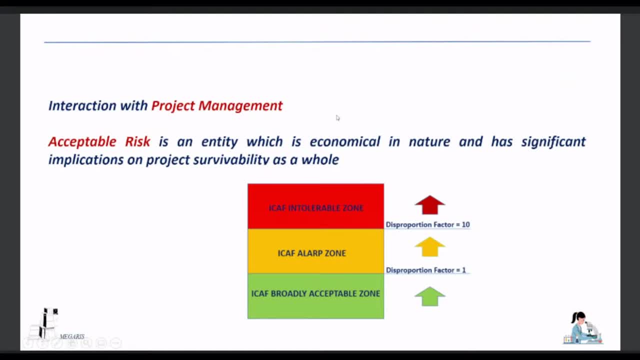 So we have to consider that it is essentially, let's say, an economical exercise To identify what is the risk for asset, what is the risk for environment, what is the risk for reputation and what is the, unfortunately, the cost of lives, the cost of people. 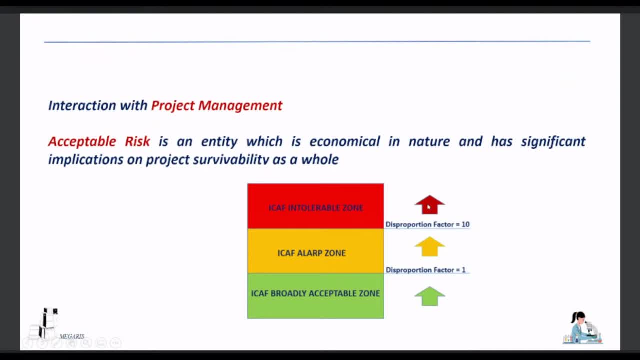 You can see here just a picture showing essentially the so-called methodology that is called ICAF. that has been introduced in the UK and also the major oil and gas companies use it in order to identify what is the so-called this proportional factor that must be managed in order to identify when the risk is acceptable, is broadly acceptable, is not acceptable. 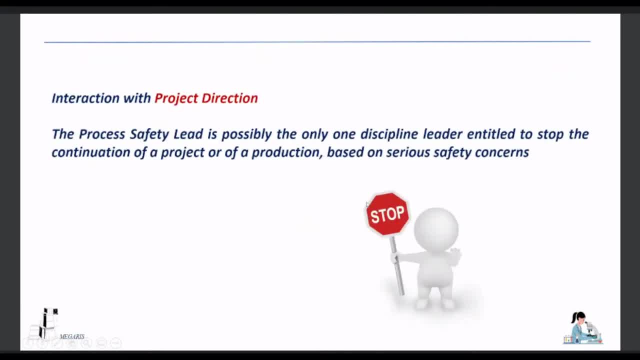 So economical implication In terms of project direction? we could in theory. it's, of course, unlikely and difficult, but process safety lead is possibly the only one discipline leader entitled to stop the continuation of a project or of a production based on serious safety concerns. 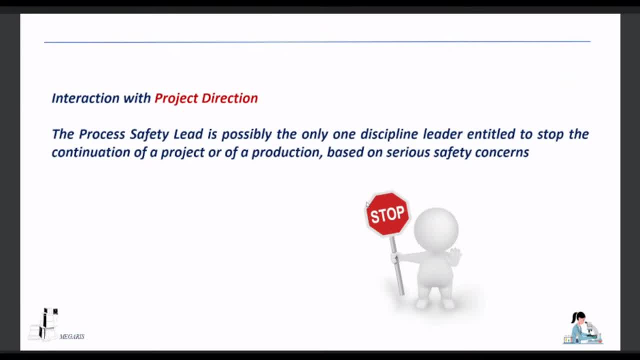 In my experience, in order to let's say okay, Okay, just to make everything robust and substantiate, I can tell you that I have been asked by a project director to fly from London to Kuwait Friday night to Saturday, because the project had been stopped anyway. 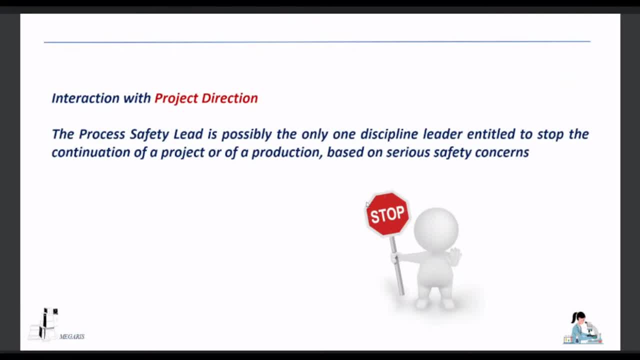 and there was the need to identify exactly the solution for some problems, for some issues. And, okay, the final green light provider was myself. So this is true, Just in order to show how important is the relationship of the process safety engineering task. 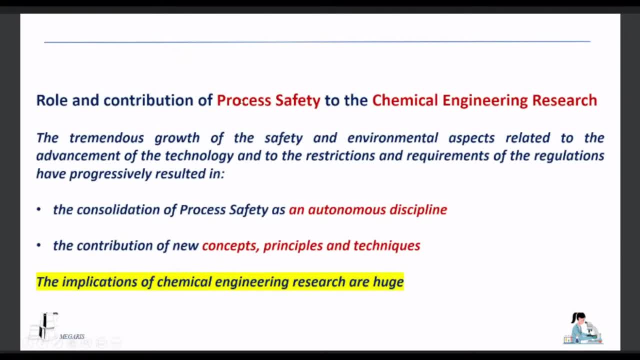 with the other part of the project Okay. so the tremendous growth of safety environmental aspect, related to the advancement of technology and to the restriction and requirement of the regulations, have progressively resulted in: consolidation of process safety as a standalone discipline, contribution of new concepts. 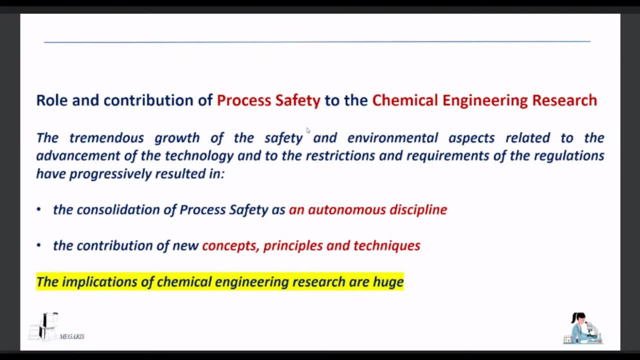 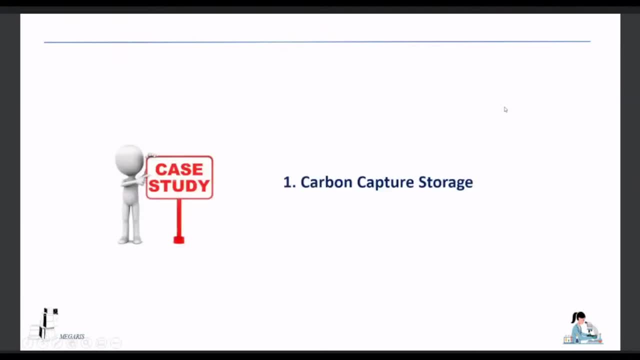 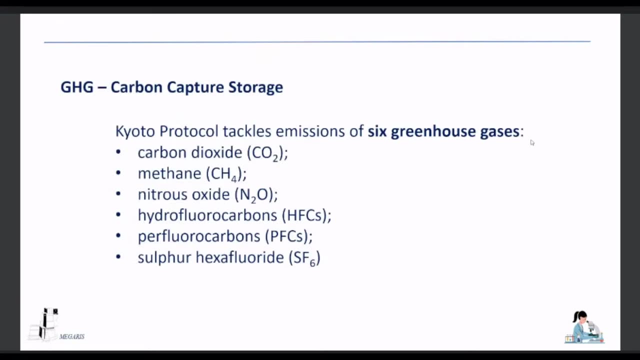 principles and techniques and the implication of chemical, So the implication, The implication of chemical engineering research are huge. So, for example, just in order to have a practical landing on the topic we are discussing, you know that the Kyoto Protocol has just identified: 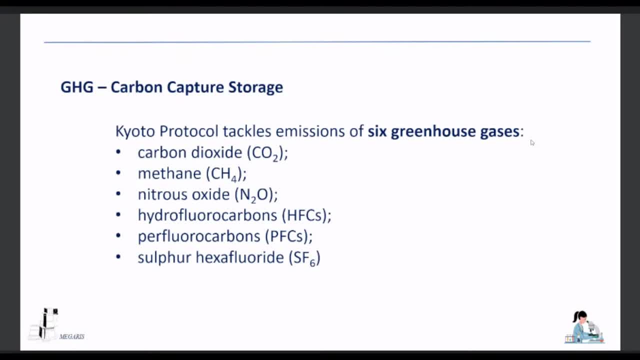 some greenhouse gases that must be reduced and, more or less, the different countries are now working in order to reduce, by some specific dates, the safety of the system. So, basically, the concentration, the release of some greenhouse gases. Of course, the enemy, the main enemy, is carbon dioxide, of course. 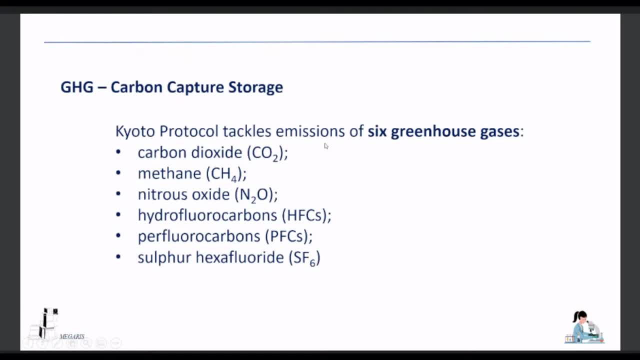 You know the war, you know what's happening everywhere in the world. Okay, we can discuss about the real effectiveness of this, but in reality, this is essentially just. these are the gases. Carbon dioxide is, of course, by far the most important. 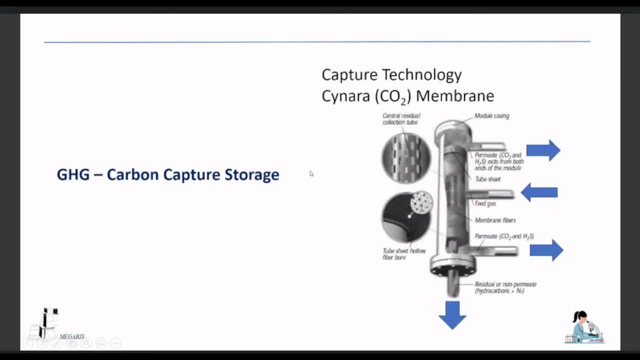 greenhouse gas to be reduced. Okay, I had some three, four experience. One is the carbon capture storage and essentially we can see here, for example, just an example of equipment that is essentially based on molecular sieve and membrane that was capable of removing carbon capture storage from methane. 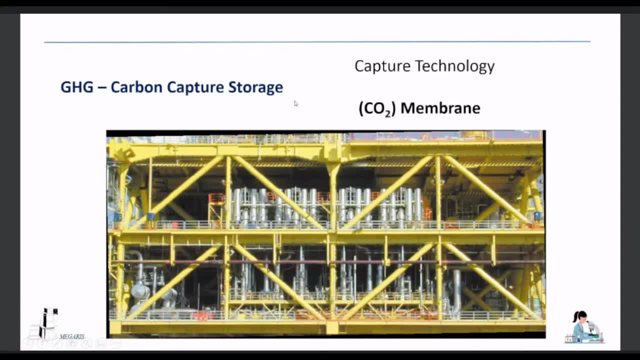 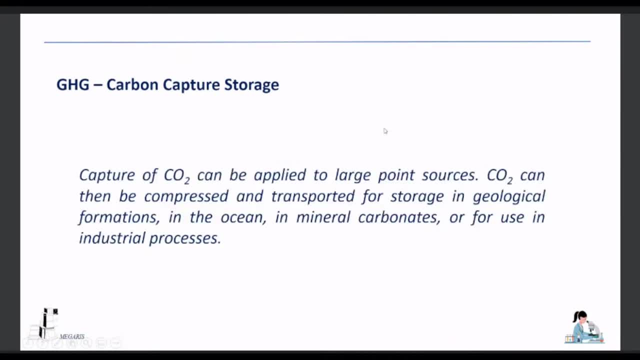 So essentially it was a carbon capture. Okay, we can see here just the overall arrangement of the plant based on membrane. so carbon, CO2.. Okay, what is essentially the defining? Okay, what is essentially the defining? Okay, what is essentially the defining? 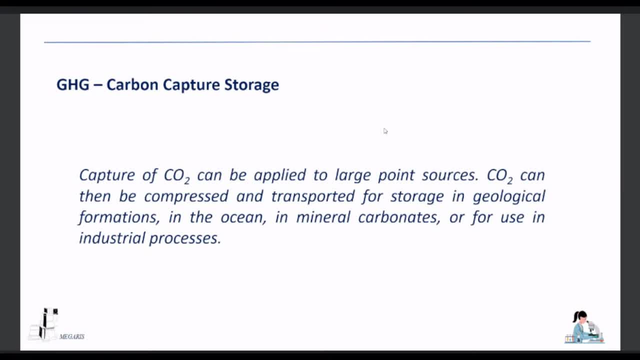 the final, let's say the final outcome of carbon capture and storage. Generally, capture of CO2 can be applied to a large point sources and CO2 can be compressed and transported for storage in geological formation, in the ocean, in mineral carbonates. 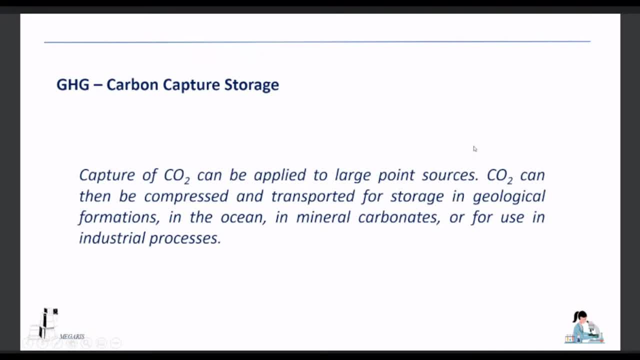 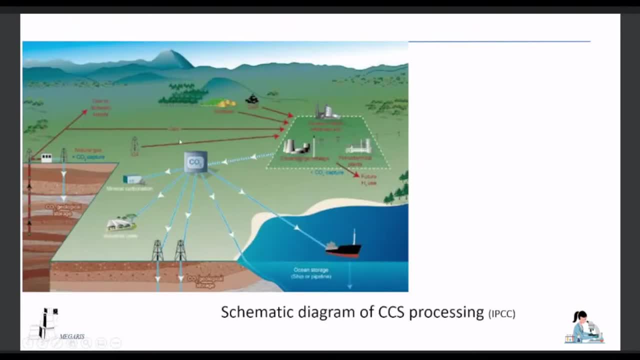 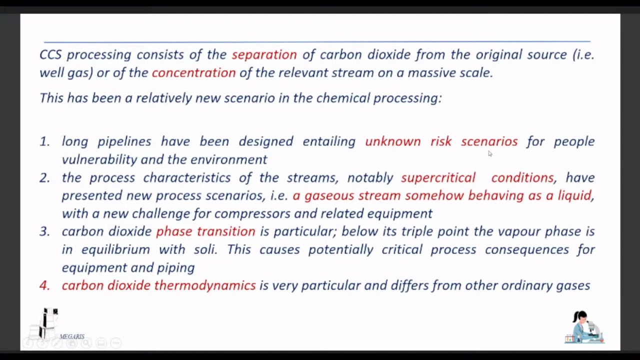 So it's easy to plan and just to foresee the way to remove and to dispose of CO2. And we can see here essentially just as a kind of multidirectional disposal of CO2.. But in reality there are some problems that have come out when we have tried essentially. 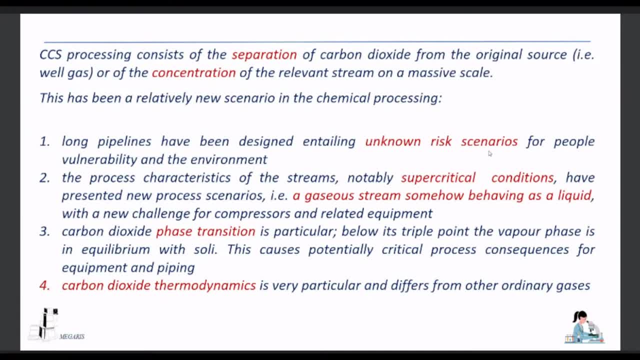 to deal about carbon dioxide, Why? The reason was essentially because, prior to implementing any carbon capture and storage regulation, the technology, the worldwide manager technology, was related only to some specific threshold of concentration and the threshold and limitation in inventory. The new problem was essentially that, starting from the carbon capture and storage new projects, 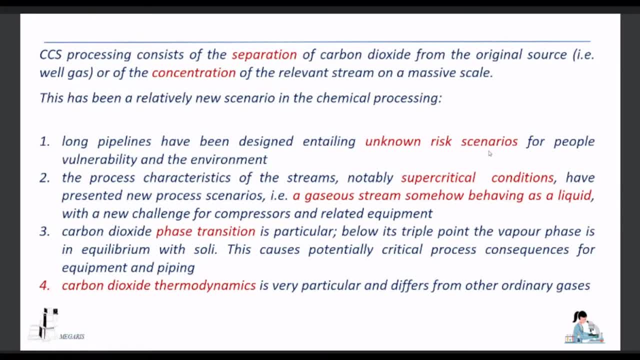 of course, we were essentially forced to manage new, let's say new horizons, just new tasks. So longer pipeline, So longer pipeline, So longer pipeline. And these new pipelines have been designed in turn unknown risk scenarios for people. 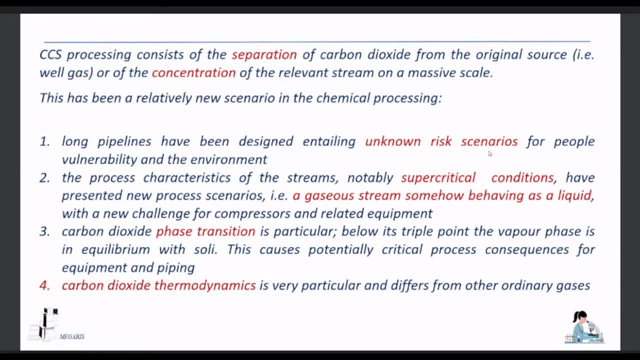 vulnerability and environment. We will try to understand why. unknown risk scenarios, The process characteristic of streams, notably supercretin conditions, have presented new process scenarios: Gasstreams somehow behaving as a liquid, with a new challenge for compressors and related equipment. 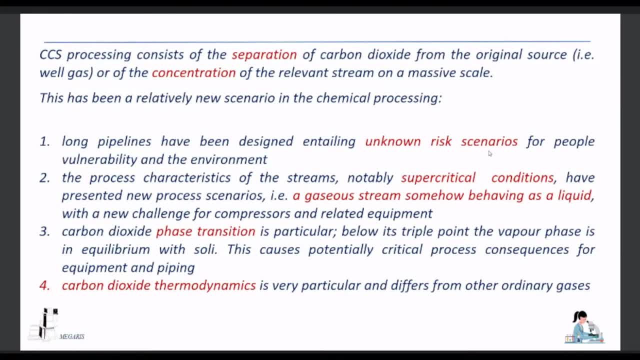 Carbon dioxide phase transition is very particular. Below it's triple point, the vapor phase is in equilibrium with soil, with solid. this causes potential critical process consequences for equipment and piping. last but not least, this is very particular and probably identify very interesting uh research, uh challenges and 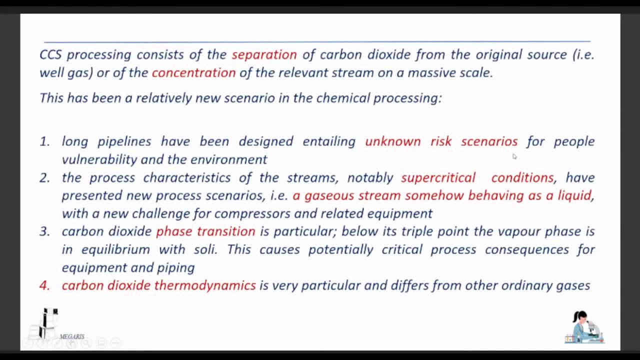 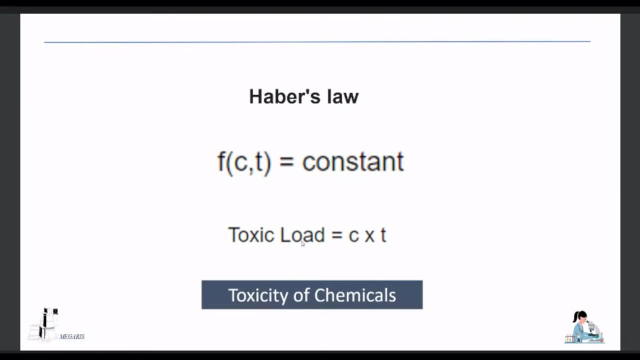 subject: carbon dioxide equilibrium thermodynamic thermodynamics. uh, doesn't work very well or does work completely, so it's very particular and differ from other ordinary gases. okay, we discussed about toxicity and about unknown variables, for okay, in what do we mean exactly? okay, we essentially know that the abers law identify a toxic load. toxic law for a chemical is: is a measure, is a product. 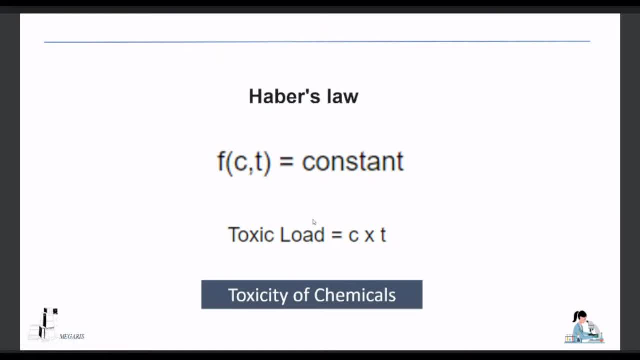 it is a measure to essentially take into account the two main parameters. one is a concentration and the second one is the exposure time. this specific, this couple of variables can probably cover all these variables. and then the second one is the exposure time. these specific, uh, this couple of variables can probably cover all these. 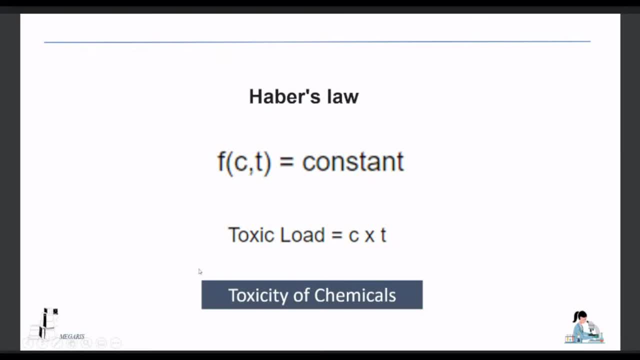 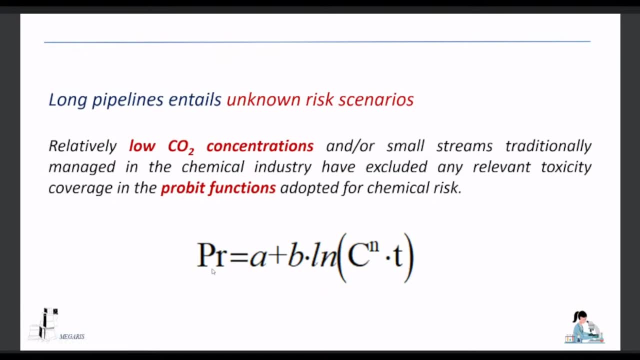 uh, the, the, let's say the- the important parameters that we have to manage when we deal with toxicity. uh, we know that essentially, uh, we, we can see that all the, uh, the, the, let's say the damage, the damage scenario for people. it's strange, but probably is a. i don't know, it's a, is a, is a law. 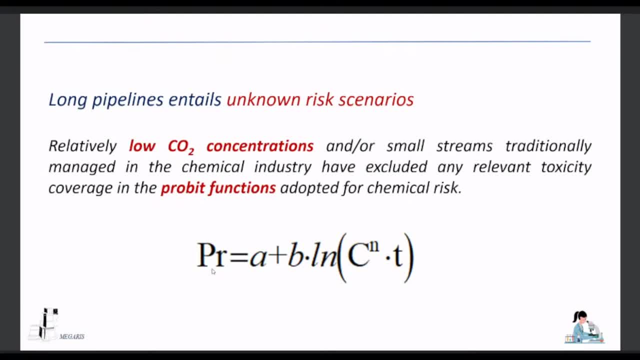 of a universe. okay, all the, the damage, the damage and the effect, the others. effect regarding fire, regarding blasts and regarding toxicity. works according to the law of the universe. works according a probably function. the probing function is, in reality, is the, the, the, the function that you can see on the screen. so we have essentially just the concentration with an exponent. 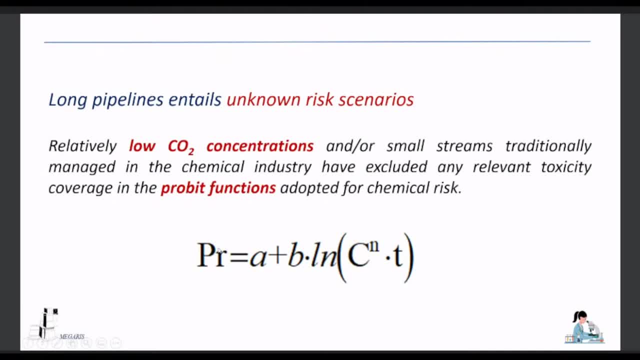 and we have this question time through the problem function. we can relate the problem function with the gaussian and we can. we can identify exactly what is the, the uh probability depending on concentration and exposure time. the probability of that of that or serious damage for people. uh relatively. 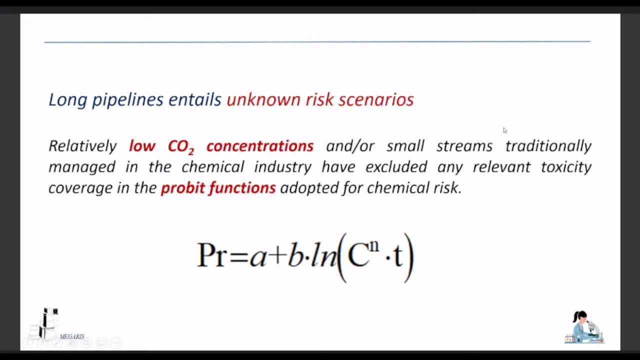 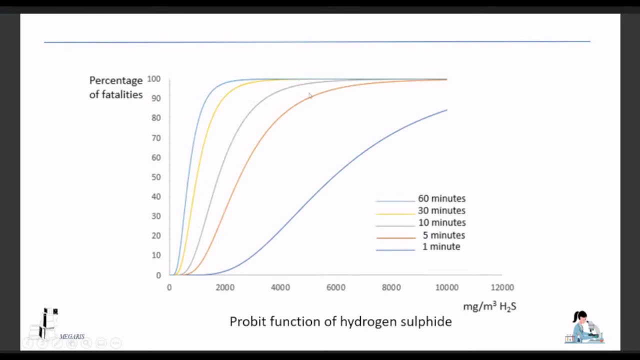 low CO2 concentration or small stream traditionally managed in the chemical industry, have excluded any relevant toxicity coverage in the proper infraction adopted for chemical risk. This is very, very weird because in reality, when we try to understand what happened, for example, for hydrogen sulfide, we can see that, using the proper infraction, we can. 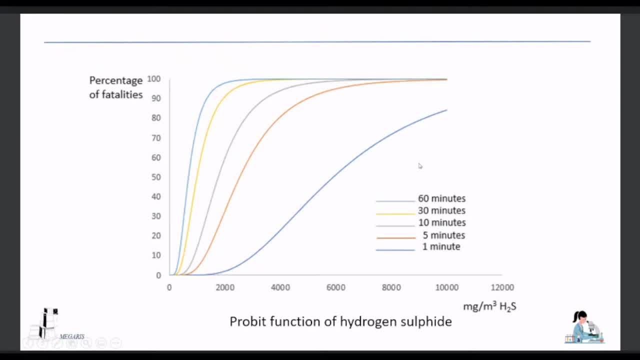 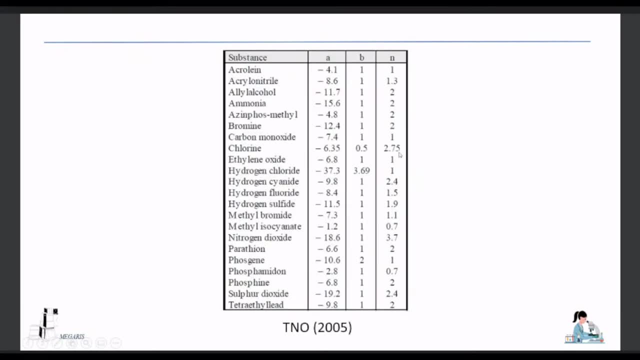 moving from one exposure time to another and depending on concentration, we can have a percentage of fatalities. In reality, the TNO, that is, you know, one of the let's say only monsters in process safety, is a very highly reputable institution, has just provided many years ago, much earlier. 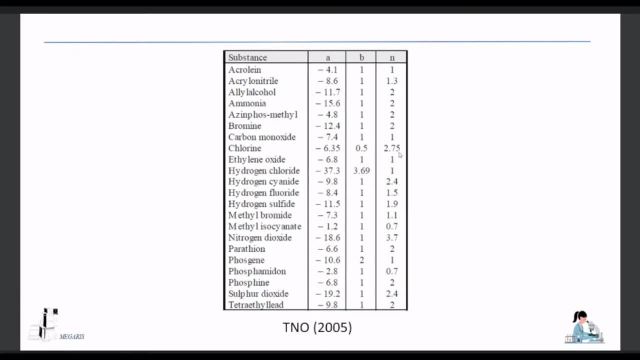 than 2005,, maybe in the 80s? okay, the list of the A, B and N that are the constant of the probing function, in order to enable the process safety engineer to arrange the probing function And to identify, And to identify exactly, let's say, the percentage of that. 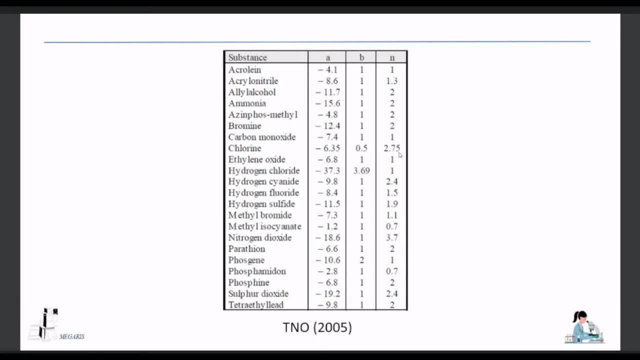 As you can see here, we don't have carbon dioxide. This is just, let's say, a strange way of thinking, because in reality carbon dioxide is a gas, so we have. probably we can expect some specific, let's say, threshold of toxicity. 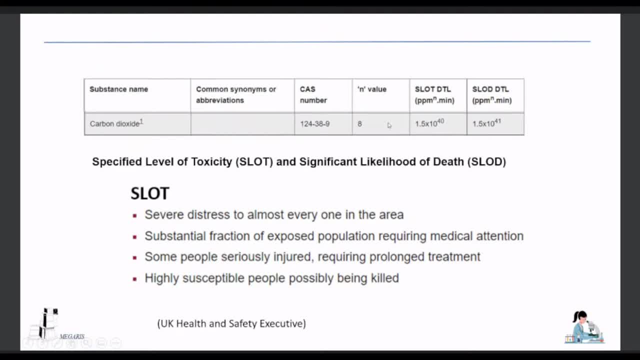 In fact the UK Health and Safety Executive. they have been working Just in order to complete the list And they have introduced Zlot and Zlot. So the Health and Safety Executive has been. there has been just a very strong research program. 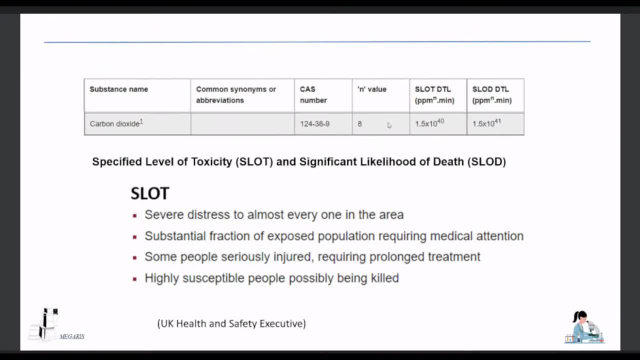 After that, essentially the okay. the carbon capture search has been introduced And in the UK there was a has been. there was just a national grid program. So the carbon, the carbon, the carbon dioxide, as you can see, is a very strong research program. 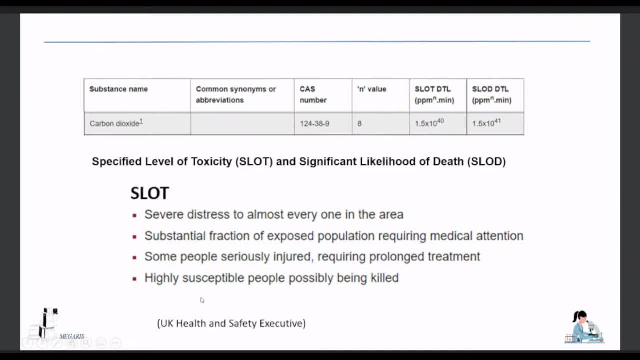 You can see now, according to the UK, Health and Safety Executive can rely on a specific probing function, So this is essentially the result of a specific toxicity research. All the other institutions, including TNO, has been working on CO2, because the problem 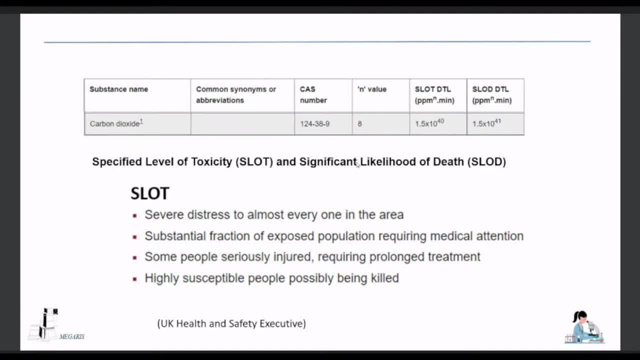 was: if we have a release, if we have just a leakage, how can we prepare our safety plan if we don't have any validated? So this is an example of how important is the chemical engineering Research in process regarding process safety for toxicity. the new challenge, the new. 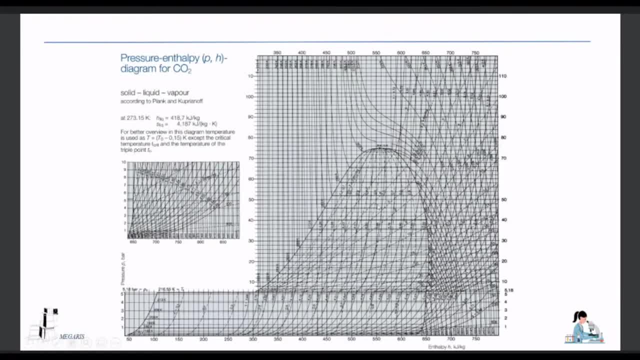 technology, the new regulation. Okay, this is the pressure enthalpy diagram for CO2, we can recognize. I think we can probably have. okay, we can here have the zone of liquid on the left hand side of the slide. we can have the vapor liquid. the vapor liquid, okay, equilibrium zone in the center. 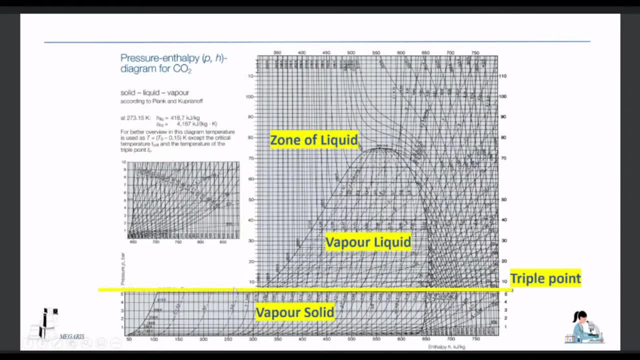 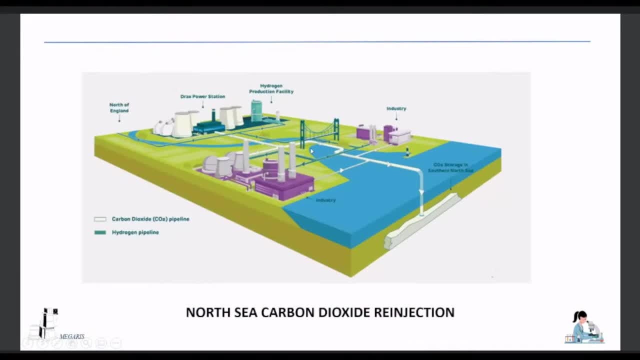 and we have a triple point. Triple point should be around the five bars below. below five bar, We only can have a triple point. We only can have essentially a vapor-solid equilibrium. If we can see here, we can see here, how the carbon dioxide reinjection was, has been. 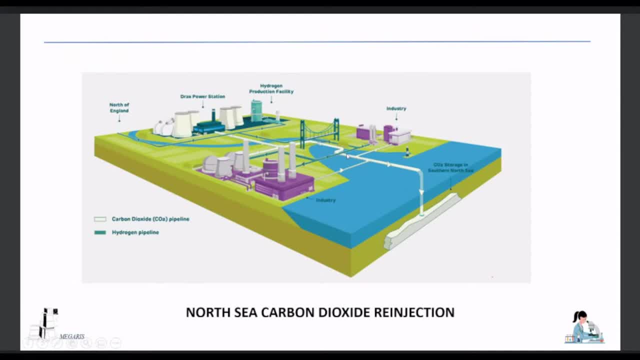 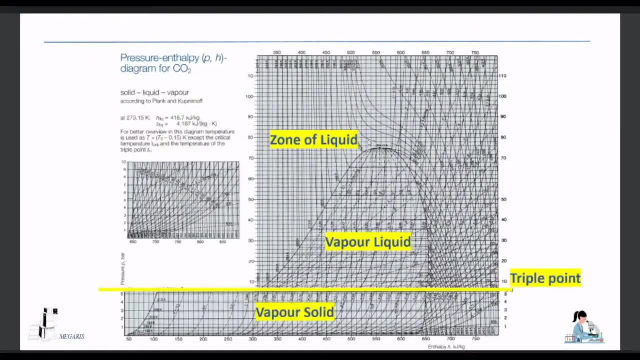 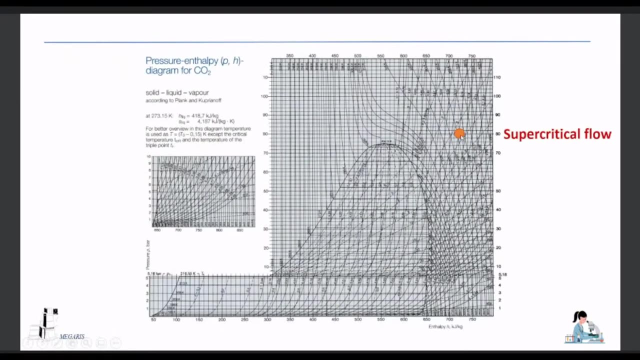 planned in the UK. I attended some specific project and so I've been working about the okay, the carbon capture and storage related to the national grid in the UK. It's important just to focus on this diagram In reality normally. normally, for example, I work in Mali. 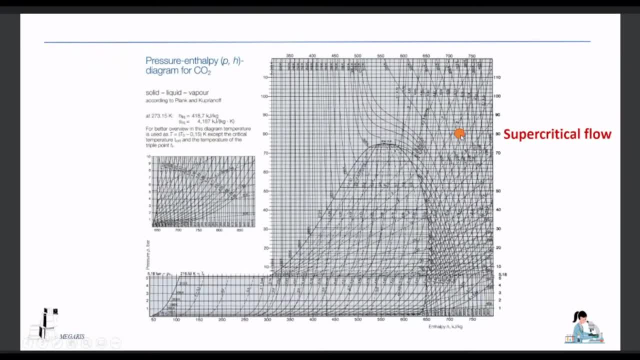 I work in Malaysia about carbon capture and storage And I remember that in reality, in Malaysia, the Petronas are planning to implement carbon capture and storage for their plant and they will be managing supercritical flow. So this is essentially the condition. 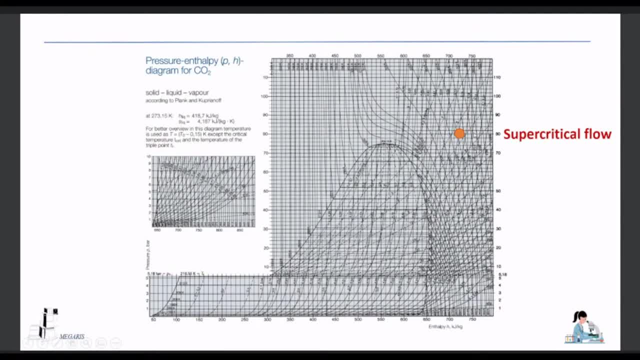 We should be around maybe 80 bar, okay, And we have supercritical flow. So if we, if you now just think about just the pipeline, you can see essentially, essentially we have supercritical flow And supercritical, supercritical carbon dioxide flowing. 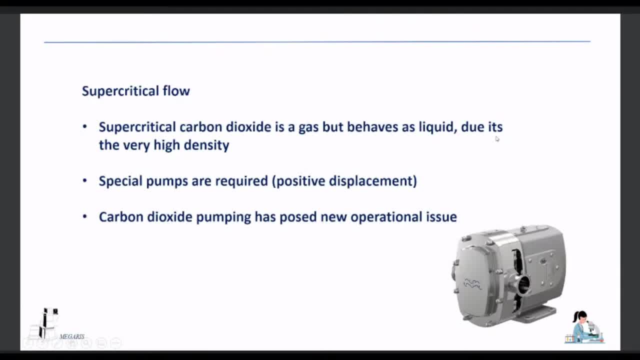 Supercritical flow means that it's a gas but we have as a liquid to its very high density. Special pumps are required and there was not memory. So there is the, the, the research and development. research and development, let's say research. 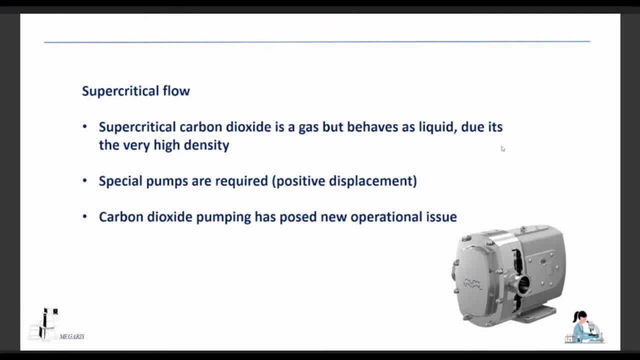 and development department of Petronas, they've been working a lot in order to identify exactly the process condition of just supercritical flow, Okay, Supercritical carbon dioxide. So carbon dioxide pumping has posed a new operational issue And, once again, chemical engineering research has been working and is still working about. 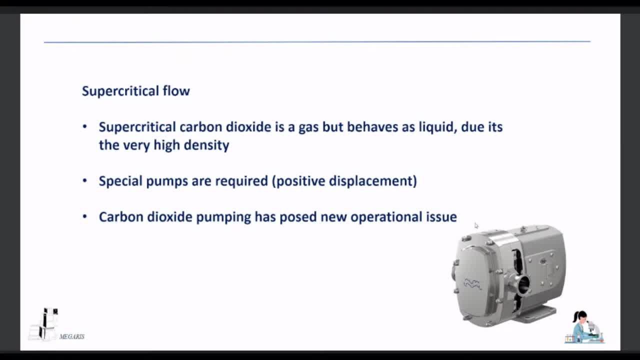 what is the best operating way to to, to, to, just to, to, to to to flow, just to to manage and to pump liquid or supercritical? So this is very specific. There was not, not memory about it. 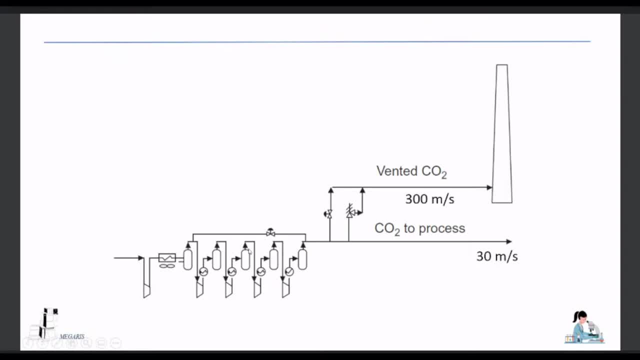 We can see here essentially just we have a comparison. Okay, We have a compressor and we essentially have just the. okay, the, the ordinary process line is the 30 meter per second is the velocity of the CO2 that is is going to be to be. 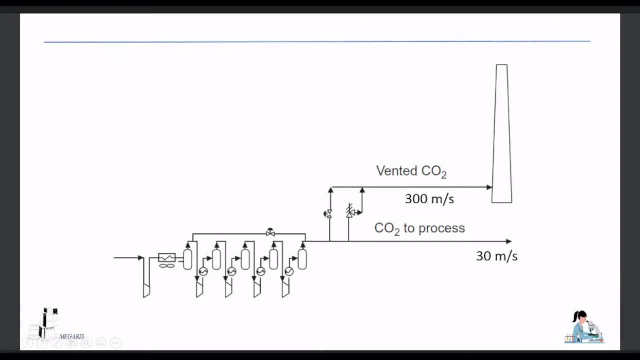 essentially flushed downstream, But we also have here essentially a pressure relief valve that is able just to vent CO2.. Of course we are in sonic condition. Okay, We have sonic condition, So expectedly our velocity, if we have the pressure relief valve, operation is going. 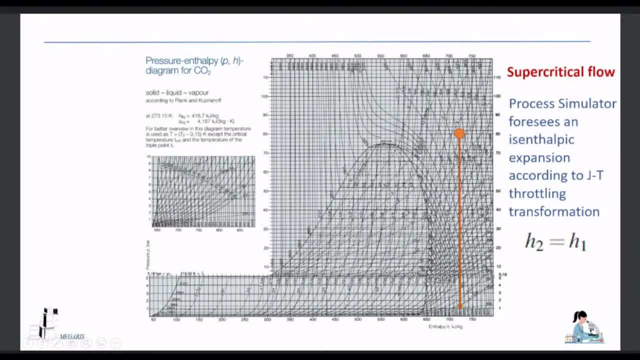 to be about 300 meter. second, Okay, I remember that I had just a specific, specific discussion with the process guys and they applied ICS. ICS said, okay, you have an isenthalpic because you can, you can have just the the John Kelvin. 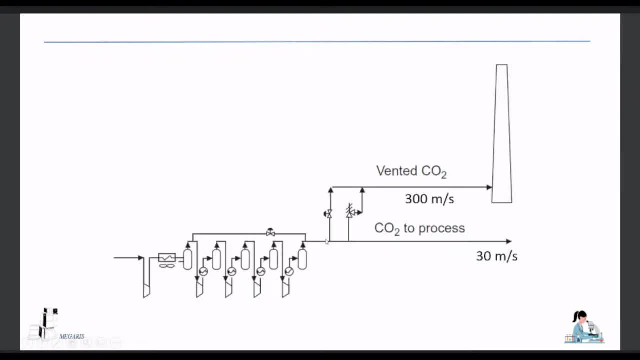 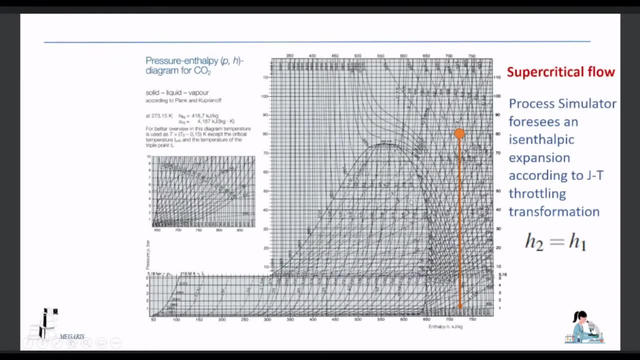 John Thomson effect. It is isenthalpic if you have essentially a release through the pressure relief valve because by memory- okay, the previous memory of the simulator was okay- It is an isenthalpic. So the downstream isenthalpic Okay. 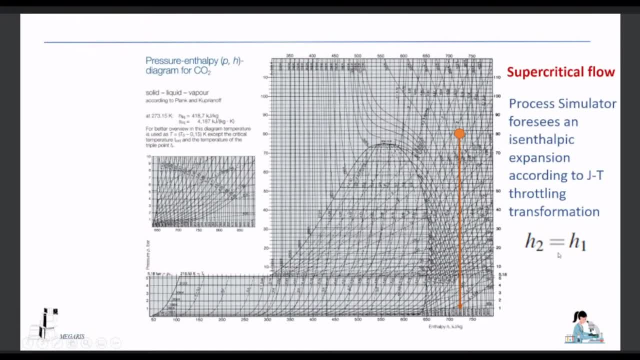 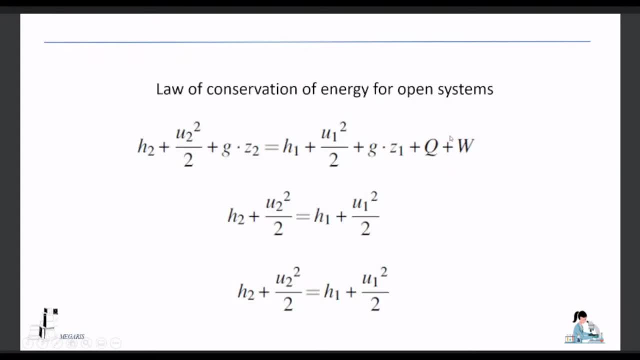 is the same as the upstream enthalpy. So processing, therefore, is an enthalpy expansion according to JT, throttling transformation. But we know that, in reality, the Joule-Kelvin-Joule-Thompson equation that we can see is obtained from this equation. 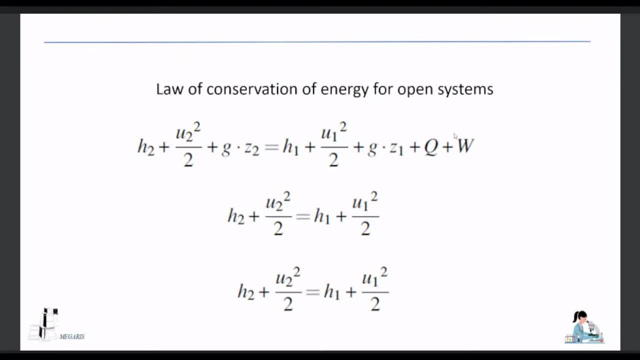 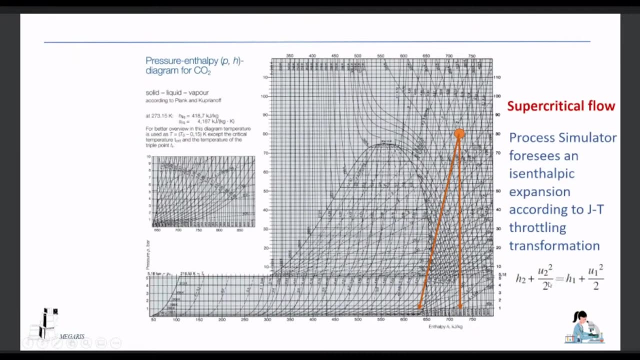 that is essentially the law of conservation of energy for open systems. We can conclude that we can have an isenthalpic and isenthalpic transformation, but provided that the velocities are the same. Otherwise, in reality we have essentially a different value of the enthalpy downstream. 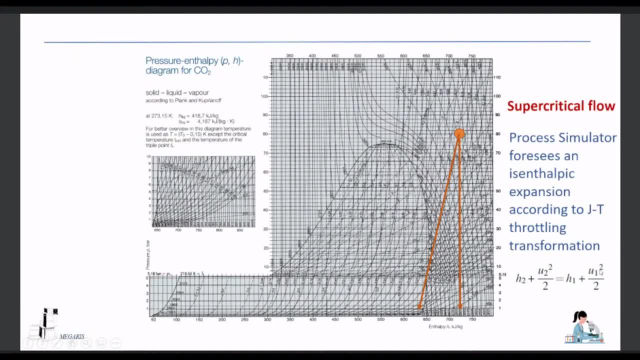 In reality, we have essentially that, if we consider that we are starting from 30 meters per second and we arrive at 300 meters per second, probably we don't have an isenthalpic, We can have essentially just a slope. regarding the transformation line, 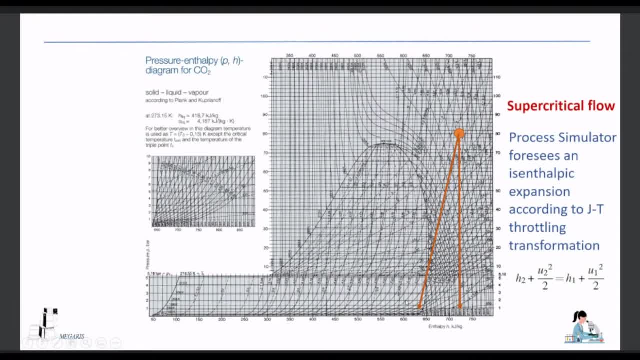 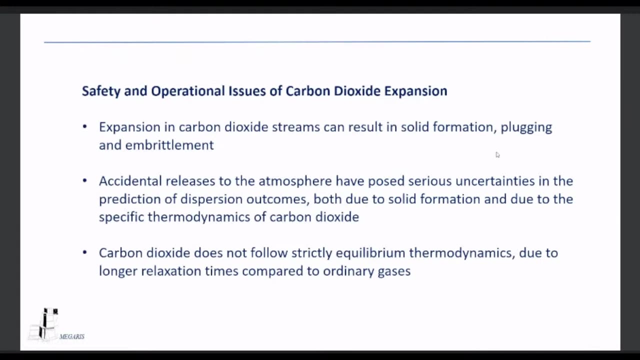 And do we have the risk to enter the solid formation zone? This was a problem that was not in the memory of people and it required a specific research approach just in order to adjust the calculation. And, in reality, expansion in carbon dioxide stream can result in solid formation, plugging and embrittlement. 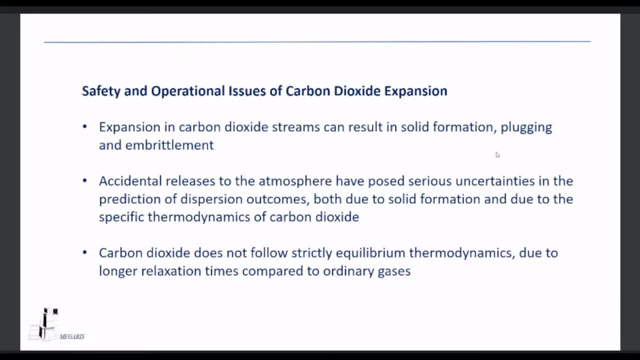 Accidental releases to atmosphere pose a serious uncertainty in the prediction of dispersion outcomes, both to the solid formation and to the specific thermodynamics of carbon dioxide. Carbon dioxide- Carbon dioxide does not follow strictly equilibrium thermodynamics due to longer relaxation time compared to the ordinary gas. 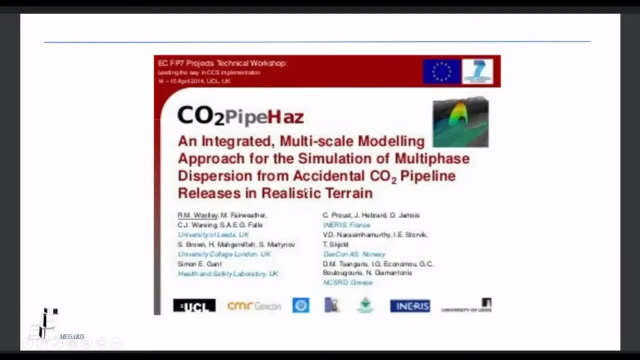 The last sentence is very important. It is so important that there was a £12 million research regarding CO2 carbon capture and storage that was led by University College London And the challenge and the final objective was: and the final objective was, and the final objective was: 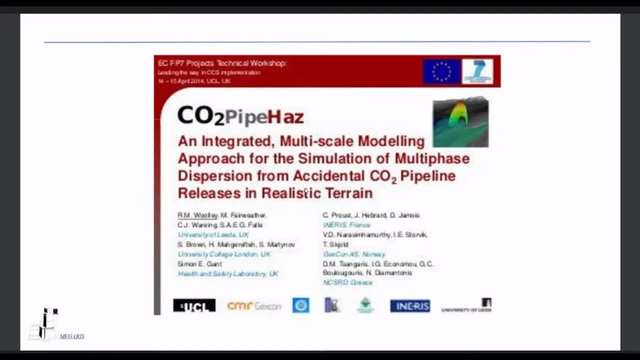 was just to try to identify what happened if we ever released from a long pipe, Because there was no memory. There was many, many differences regarding the behaviour of CO2 because there was no memory. So this was an integrated, multi-scale modelling approach for simulation of multi-phase dispersion. 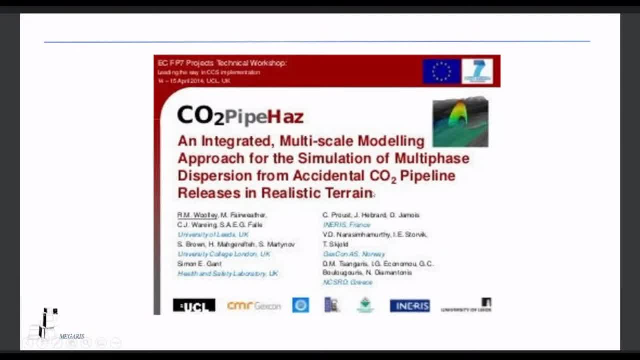 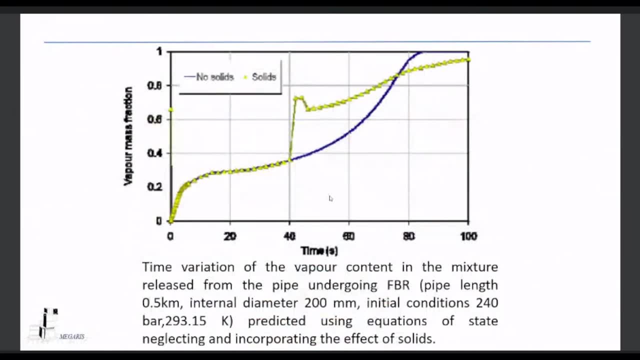 from accidental CO2 pipelines in a realistic term. This is essentially the flowchart of the project We can jump. This is very important And it's probably the heart of our discussion that we are going to finish And we can see here that in reality, 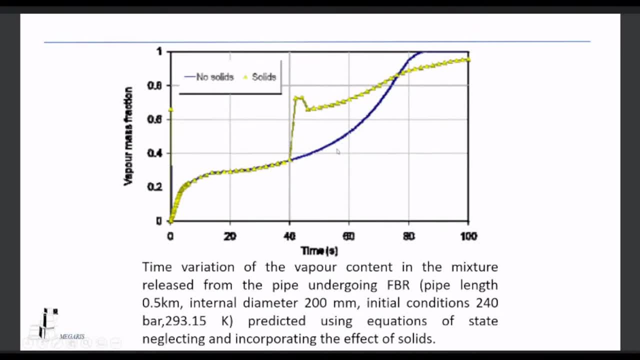 the blue line is the line that probably we can expect to follow if we apply equilibrium thermodynamics. What the researchers discovered regarding this project, the CO2 pipe adds. in China there was a long pipeline industrial scale that was operated in order to understand. 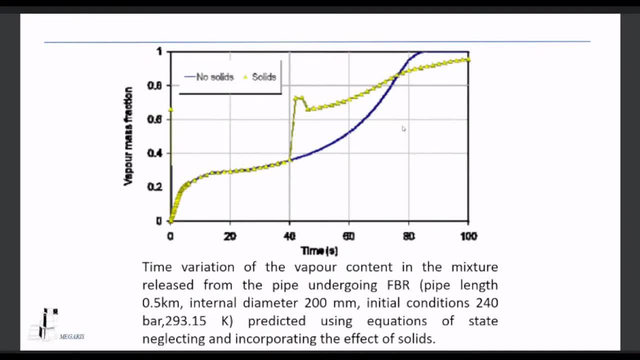 And there was a simulation of release and the measurement regarding essentially the behaviour of CO2.. And they discovered essentially that in reality there was a significant departure of, let's say, CO2 in terms of the vapour and the vapour solid, because here we are below the triple point. 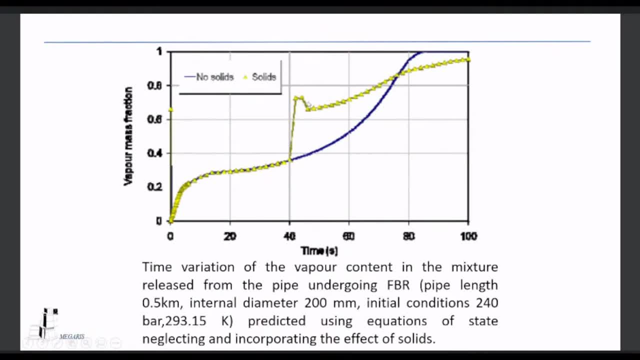 There was a kind of over-saturation. We can follow the yellow line because the relaxation time, that is the time taken by the CO2, to follow just a phase transition, For example, if we have nitrogen oxygen or if we have water, and we are following a transition. 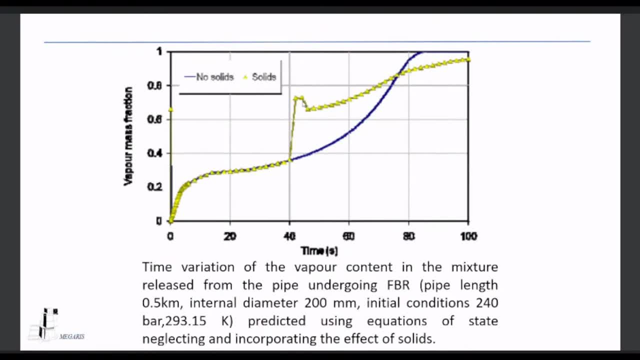 we can probably expect some time in order for one phase to move to another phase. In this case we have essentially a much longer time. So they experienced essentially an over-saturation, accumulation of, let's say, higher concentrations of, let's say, higher concentrations of, let's say, higher concentrations. 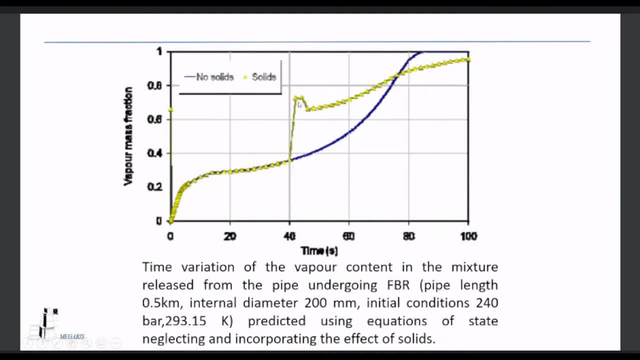 of vapour mass. that was not expected, adopting the equational state of the carbon dioxide prior to moving to the solid. This was essentially achieved, obtained just thanks to the research program. It was a long, long, multidisciplinary program that was essentially aimed just to understand exactly. 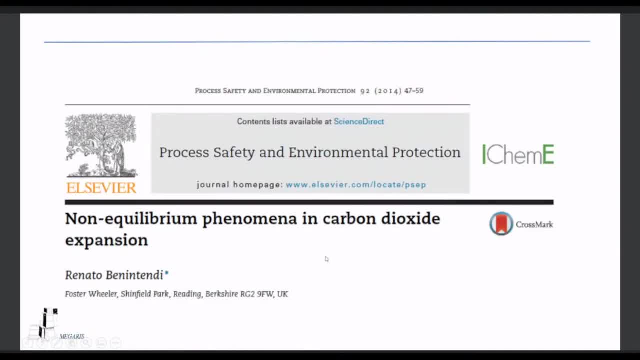 what is the behaviour? because there was no memory. I just played about this point and I in reality, it was very nice to me to try to have a kind of theoretical model to explain why is carbon dioxide so different And why, when you are going to have just a plant, 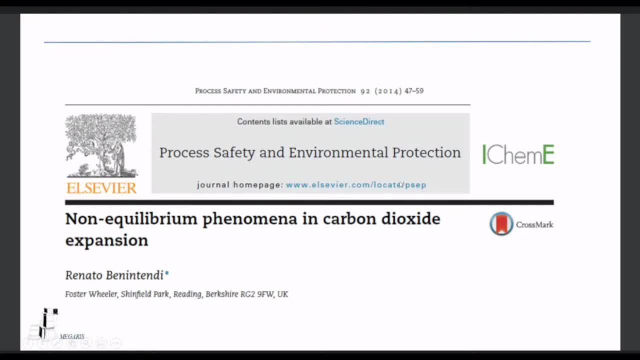 and you are feeding carbon dioxide, you can expect to have some strange and unexpected behaviour that can impact and can be really that can be really really bad for the environment. That can impact and can be really really bad for the environment. That can impact and can be really really bad for the environment. 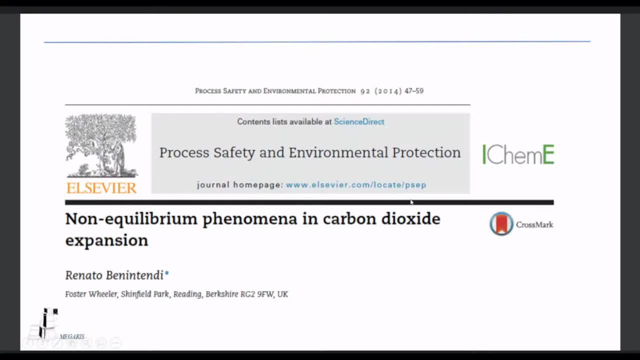 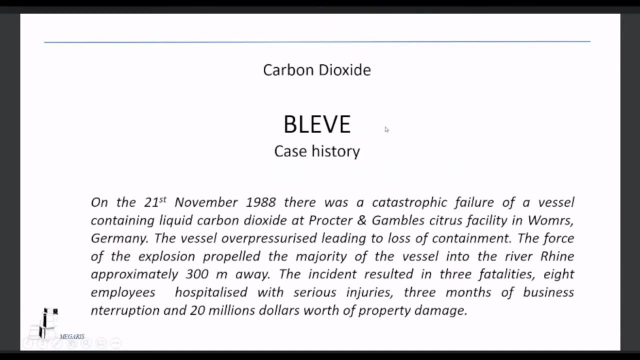 really serious in terms of the equipment health, but also in terms of process safety. Okay, very, very, I'm very fast. Carbon dioxide can undergo plating because of course, it's a liquid And if we have just a catastrophic failure or collapse of tank, ruptured tank, 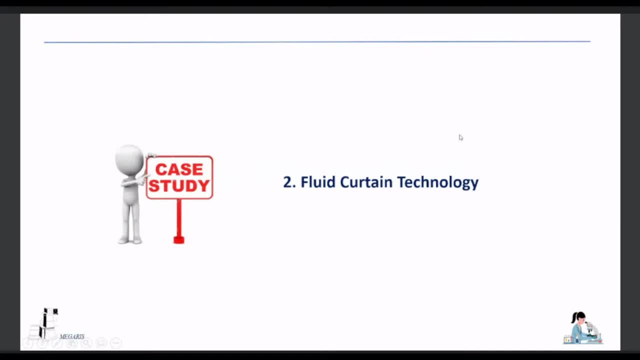 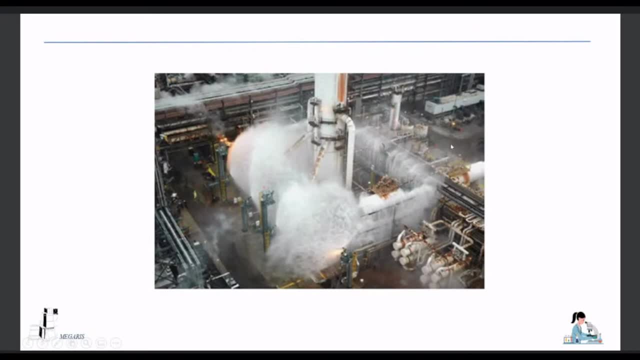 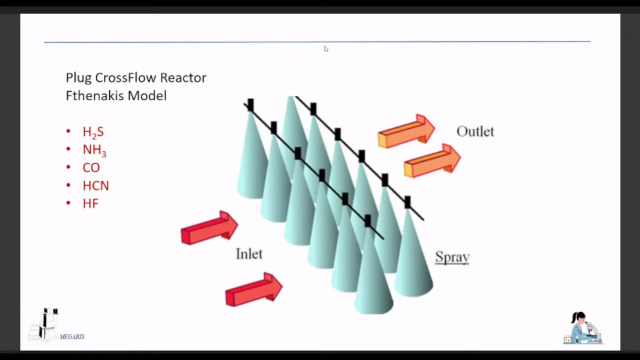 we can have essentially just an expansion And okay, and going on, we can just close this discussion. presented: fluid coordinate technology. Okay, fluid coordinate technology is essentially just a process safety mitigation system that you can adopt when you are in presence of some specific hazardous chemicals. 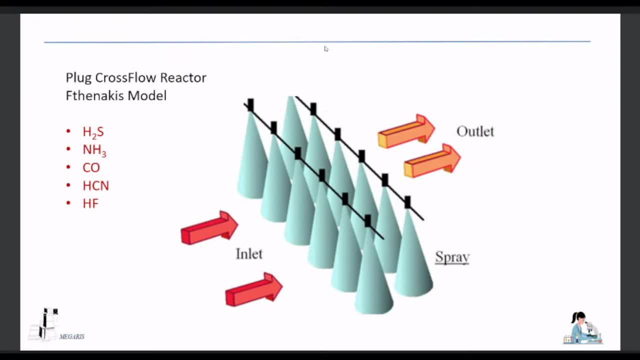 such as H2S, ammonia, CO, HCN, HF and others, And your risk scenario has not been, doesn't comply with risk limits. So prevention: If it doesn't work, you must mitigate it. Okay, I personally have just been working a lot about this for three years, in my last project. 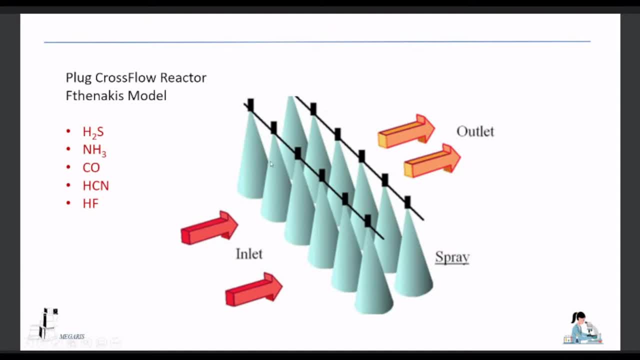 And the peculiarity of this specific system and process is that this is a plug cross flow reactor that works according to the Fenakis model. Professor Fenakis is a professor And I've been discussing with him after my just some publication And you can see that it's unlikely that you can have this specific reactor configuration in process engineering. 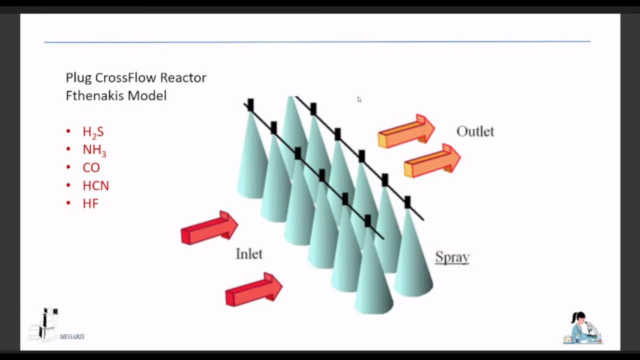 So I can say that this is specific for process safety. So it means that just a specific dedicated research program for just a reactor configuration like this can just result in Being effective, because normally this is an open space, an open space reactor. You have essentially just release of leak of H2S, ammonia. 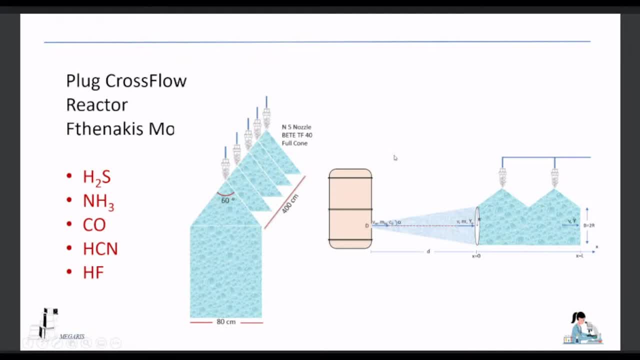 And you can have a specific configuration that you can follow here. You, that is is is not- is not very easy to design because must work according to very, very specific parametric range And and you can have, you can have a reduction, you can remove, preventing the release from impacting on people and 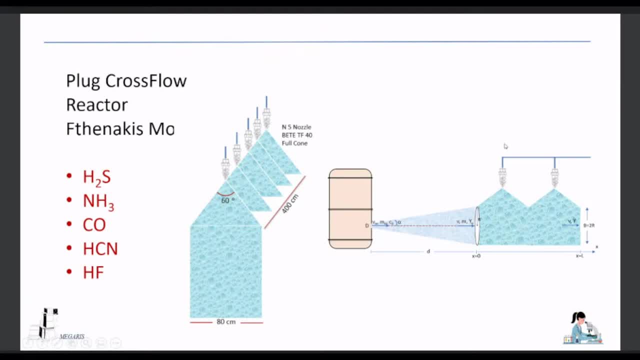 environmental by 90, more than 99%. This is a specific, specific configuration of reactor configuration that belongs to process safety engineering And the C requires a lot of of research efforts in order to extend- I probably may be the chance to to adopt this, this technology for H2S. 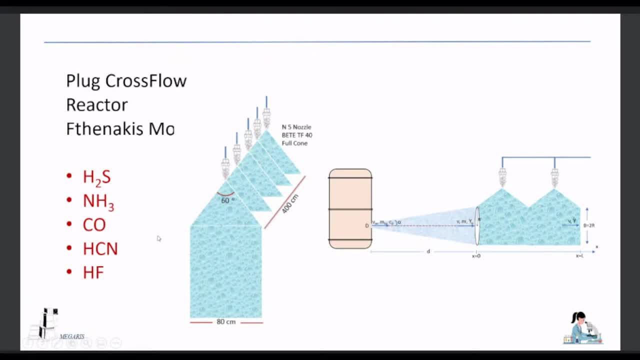 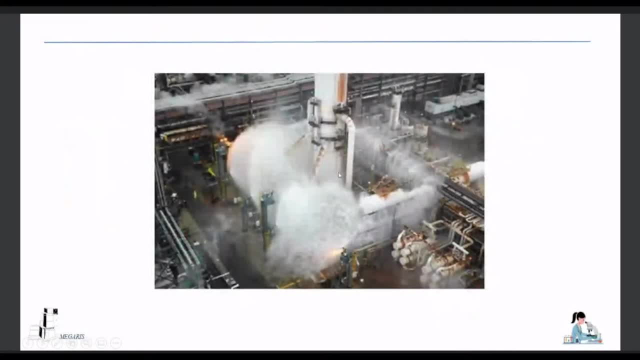 Typically this, this, this has been applied in the past to HF. You can see, probably, no, probably, it was okay. you can see here the picture: uh, this is maybe a Ramco. uh, in the alkylation project you have HF and there was a very lucky and effective adoption of of fluid curtain for HF. 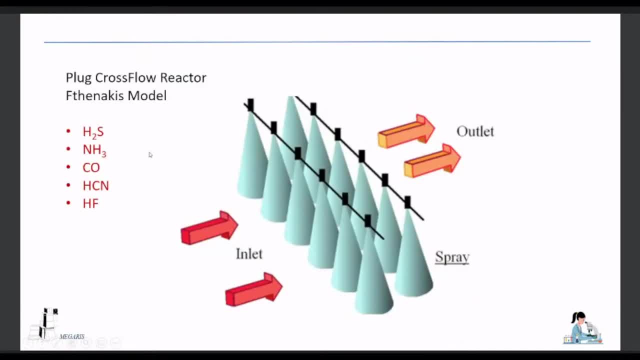 There was no memory for H2S and there was a big project in in in uh in the Middle East And I was. I've been working a lot in order to adjust because it was different, especially, especially because H2S cannot be the every. 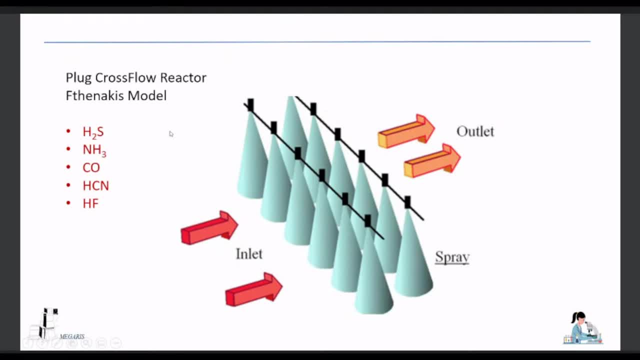 Okay, Coefficient for absorption is not good. So we have to work a lot and we we carried out a research program, a program in order to adjust and to adapt this uh specific uh cross flow reactor configuration to H2S. 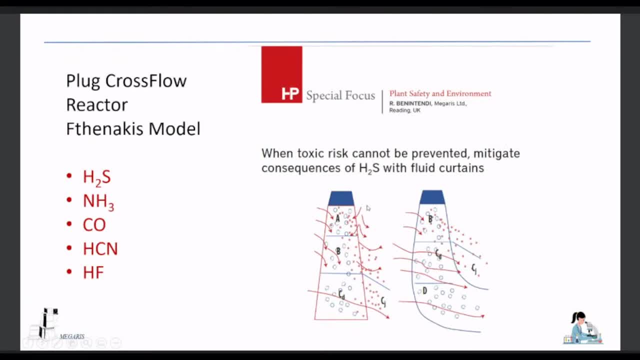 This is an additional example. Uh, here you can see the thermal fluid dynamic. The fluid dynamic part is very important. If you, if you fall outside the range, the system doesn't work. So this is very, very difficult and require a lot of study. 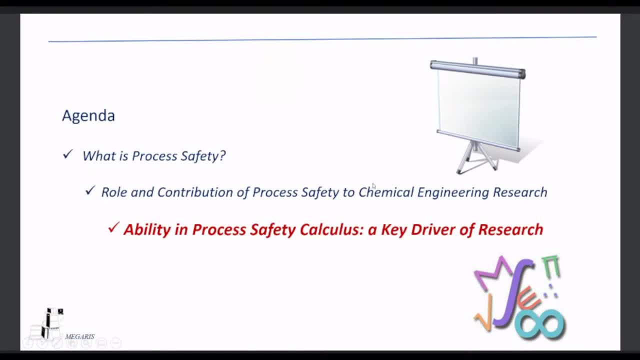 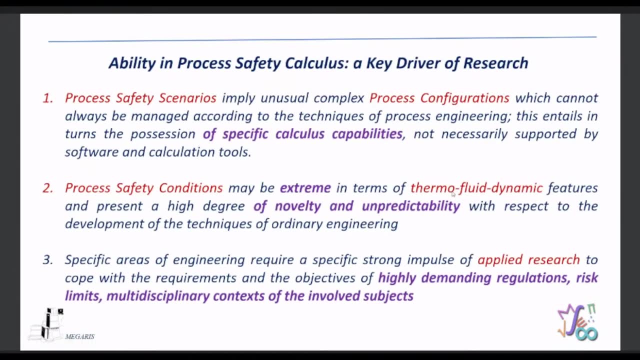 Okay, Uh, now we conclude with Three, four slides. So ability and process safety calculation, a key driver of research, We can say we can conclude. process safety scenarios imply unusual, complex process configuration which cannot always be managed according to the techniques of process engineering. 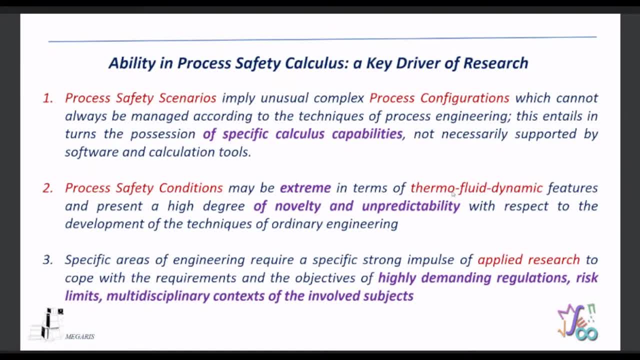 This entails, in turn, the possession of specific calculus capabilities, not necessarily supported by software and calculation tools. So the process safety engineering must be very, very clever. in calculation process safety condition may be extreme In terms of thermo fluid dynamic features and present high degree of novelty and unpredictability with respect to development of the tech techniques. techniques of ordinary engineering. specific areas of engineering require a specific, strong inputs of applied research: research to cope with the requirements of objective, highly demanding regulation, risk limit, multidisciplinary context of important subjects. 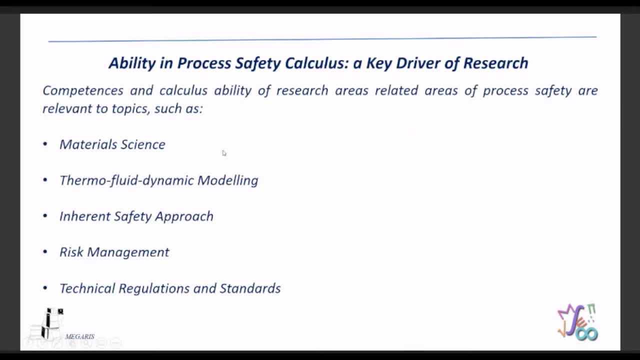 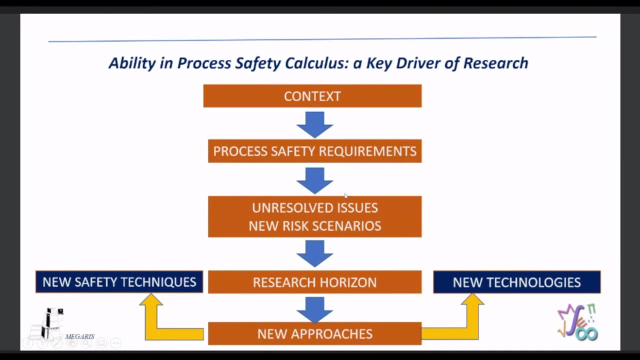 So, uh, what, what, what, what is the, let's say the, the, the, the, the panel of competencies, I think material science, Thermal, fluid, dynamic modeling, you know, in safety approach, risk management, technical regulation and standard, she are. we can, we can see, uh, a kind of uh, just a conclusive, uh summary, uh, what is the relationship between an ordinary route of the process, safety engineer task and the research? and, okay, we can say that we have normally a context. 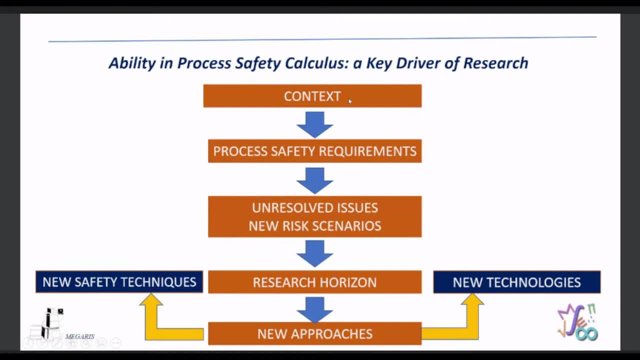 This is also consisting with my experience. Uh, we have some process safety requirements. Okay, Typically we can have not, it doesn't open always- but we can have unresolved issues and new scenarios. So we we have a research horizon We are forced to up to, to essentially face new approaches. 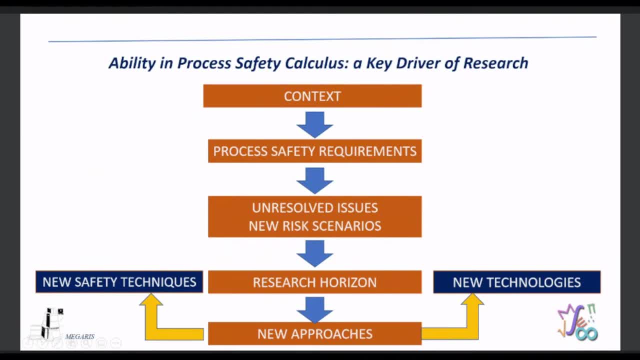 What? what is the final outcome of a new approach can be new technologies and the new safety techniques. So we can essentially uh split the final outcome of uh, the, uh, the, let's say the research in in process safety. 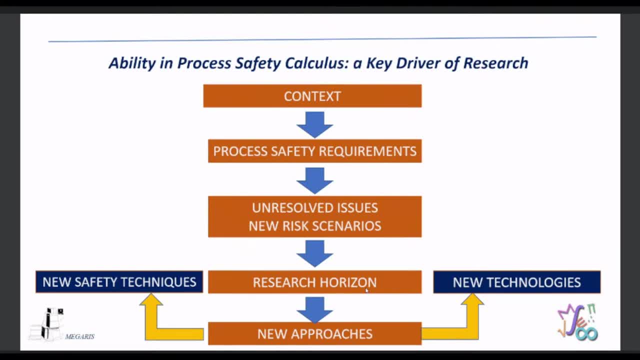 We can have. We can have the final game that we can earn. We can have a final gift that consists of new technologies. means new technology also, let's say, other than a process safety. No, we can have a lot of new materials. 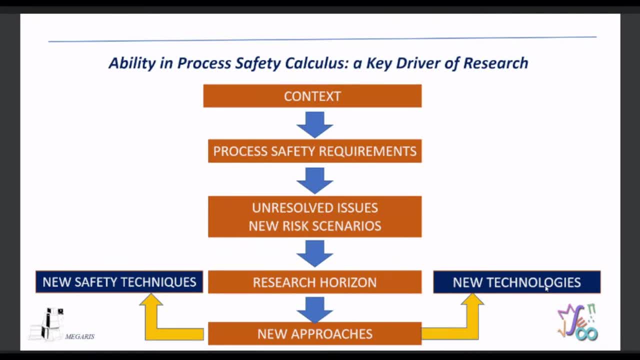 We can have a lot of new technicalities, new process configurations coming from the process safety scenario, and we can also have new safety techniques themselves. So working for uh, let's say uh process safety in order for uh- making a process safety more effective. 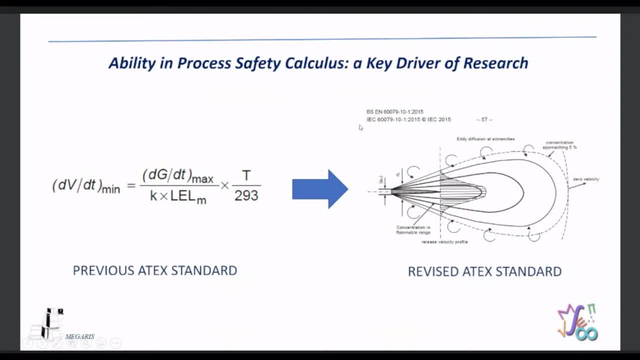 Uh, for example, and I conclude, uh, this is, this was essentially the previous eight X IEC and European norm. uh, until 10 years ago you can, you use it essentially the low explosion limit and you have absolutely huge cloud that were absolutely unaffected because you, you were using a low explosion limit, whereas normally you don't have a low explosion limit, that is is very low concentration. 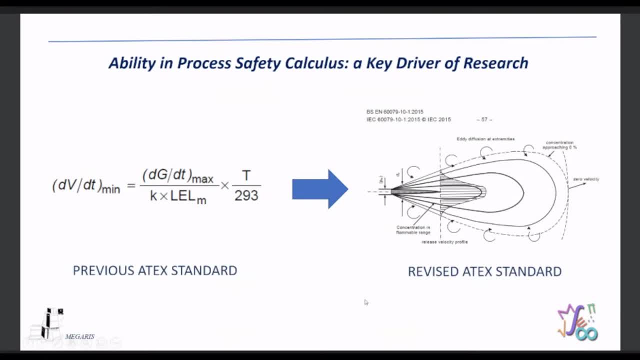 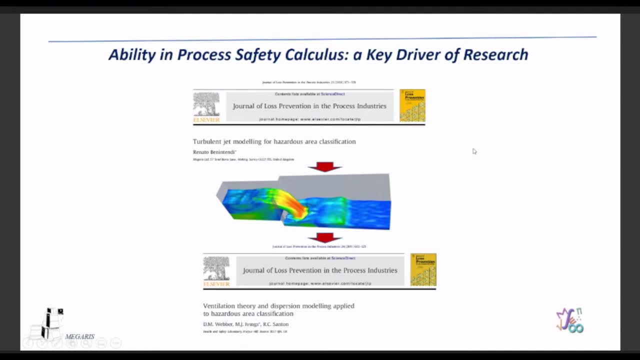 That means big cloud, And so there was a kind of of, of, uh, just a revised eight X standard. I am really proud to have to head up out in this revision because in 2010, I essentially discovered that that the terminal jet modeling for that there's a reclassification due to the air entrainment- reduces the concentration. 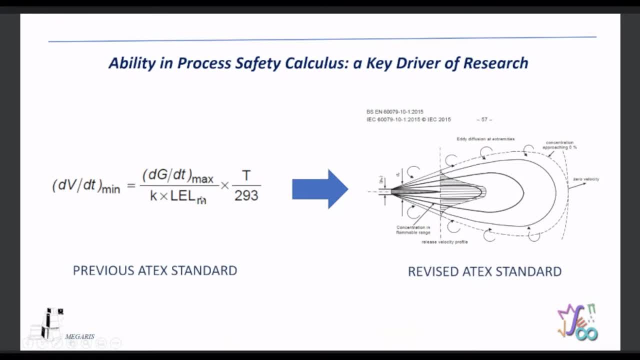 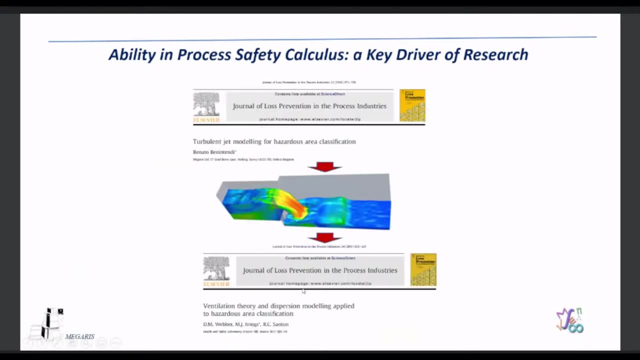 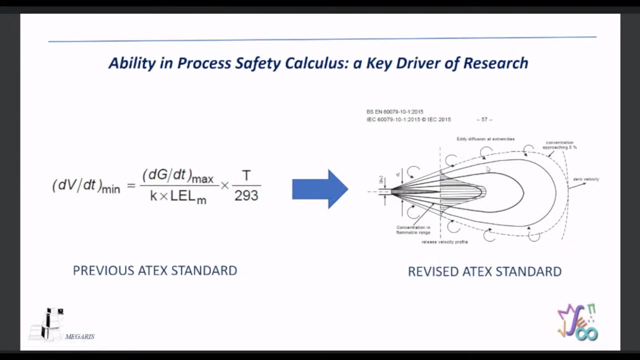 So the adoption of a low explosion limit was a, was a, was an absolutely huge uh. let's say uh, serious, serious, Uh, a drawback for the company because you had the huge uh. in reality, if there was the health and safety executive in the UK, they carried out another research program using fluent CFT and they discovered that, in reality, uh, the, the, the cloud, the real cloud, due to the air entrainment, was much smaller, much, much smaller than the original. 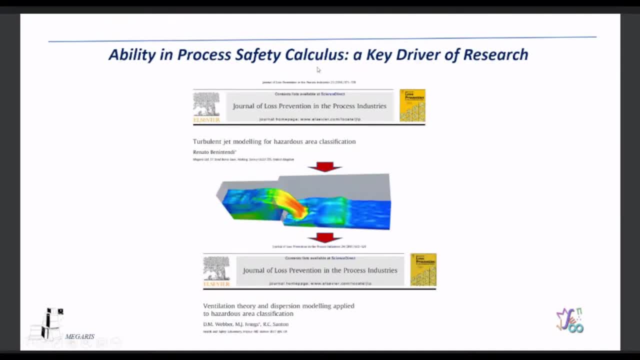 So this is essentially a clear indication on how uh ability process, safety calculation And the, the- let's say the uh, the- the execution of a, of a, of a research program was effective. Now there is a new standard that is used, with much, much smaller. 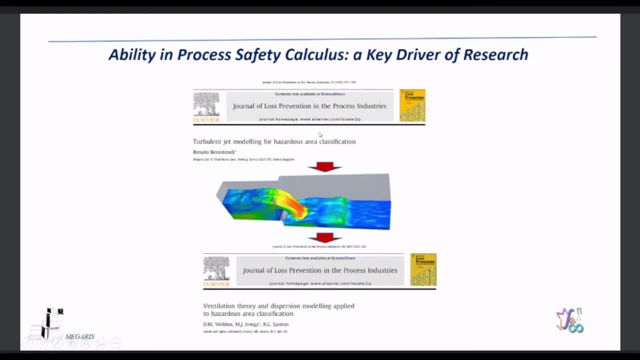 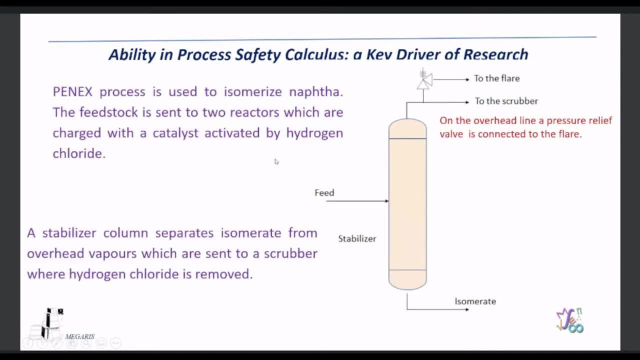 Uh, you can see here, they, they recognize the okay, the, let's say, the effectiveness of my publication, and this has been incorporated in the new standard. Okay, The last, the last one is: uh, it's, it's. I think it's interesting because during Hazel there was a, a very important. 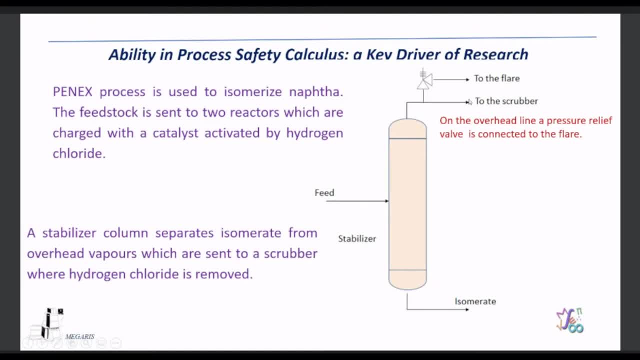 Uh, uh, licensor, uh. that essentially explained that, in reality, uh, HCL that was used in the in the Penex process as as a medicine process could be flared, And there was no, essentially no, conclusion about what was the outcome of this. 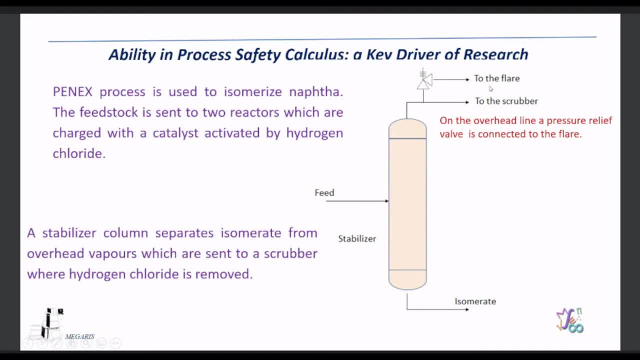 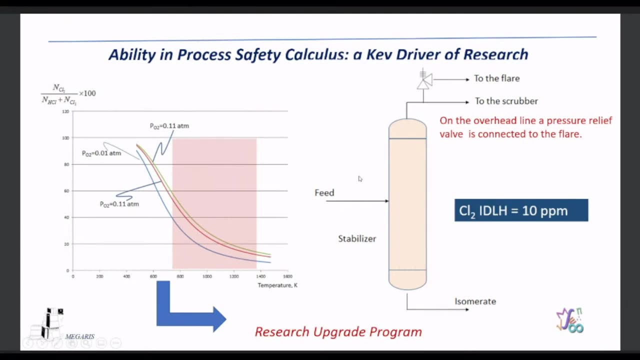 So I remember that I say, okay, what about HCL? So hydrogen chloride to the, to the flare, you can have some problem. If you are lucky you have, you can. you can keep hydrogen chloride But you can have also CL2, they were completely silent and they and they recognize that was a part of the technology that probably was not complete complete. after that they were own, just trying to cope with the problem. 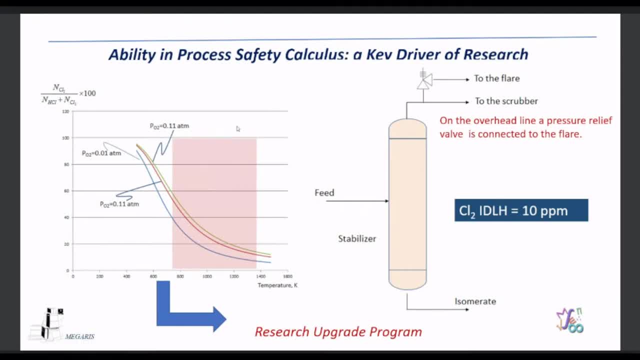 And they essentially worked about, uh, just the equilibrium, the equilibrium of the economy, that is essentially the equilibrium between CL2 and HCL, in order to find the best of the, the best of, let's say, the, the best working working point. 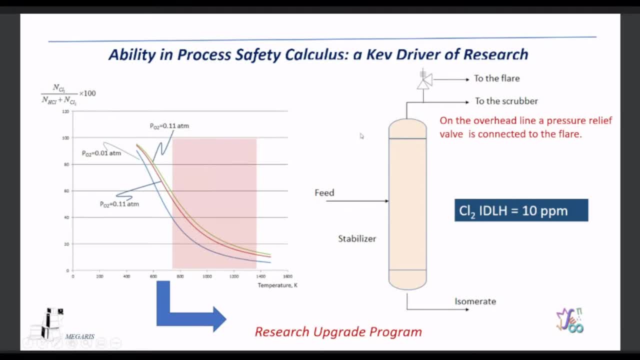 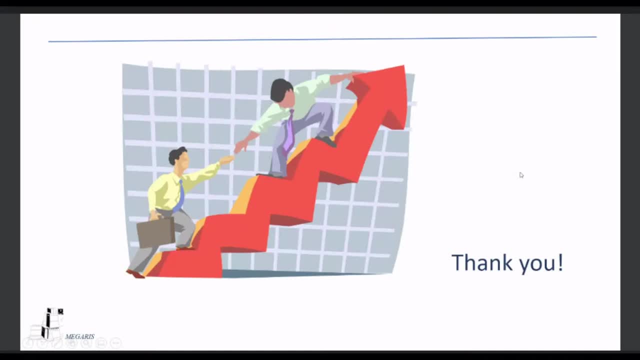 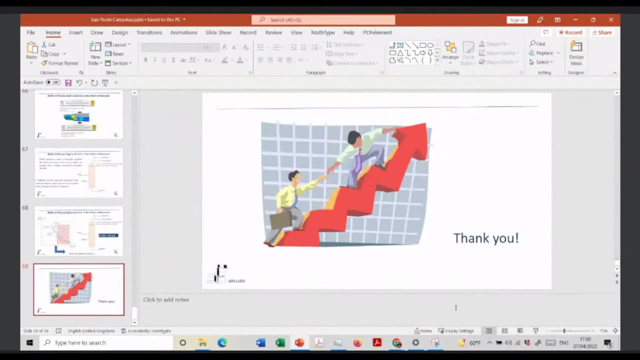 Which is basically how they. they take the most optimal, most optimal analogous conversion of the process in order to reduce any kind of risk. Okay, Thank you very much. I hope that just not be too long And I am happy just to discuss, uh, with you, with you what? 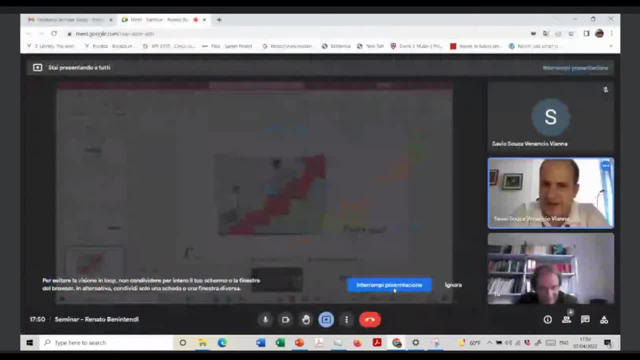 Thank you, Renato. Thank you for the presentation, for accepting our invitation. It was a uh lovely and comprehensive presentation. Uh, we have a few questions here that now we'll be going through them. So if you'd like, uh, to take a look at some other key points in this presentation, you're welcome. 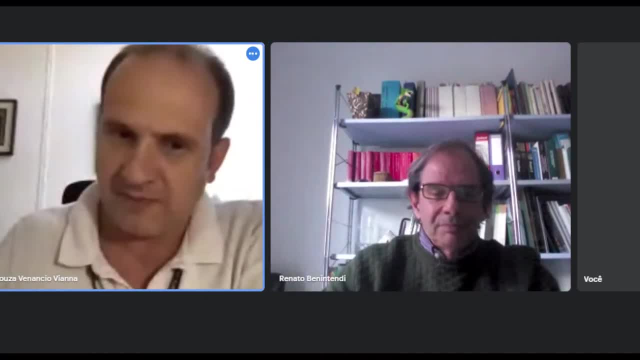 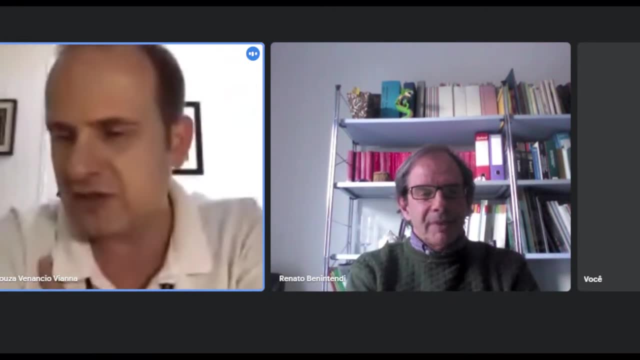 Thank you very much. Thank you very much for your attention. Thank you, And we're going to discuss a little bit. As I told you before, there's a bunch of people here from undergrad graduate students and researchers. So just assuming that the questions are, 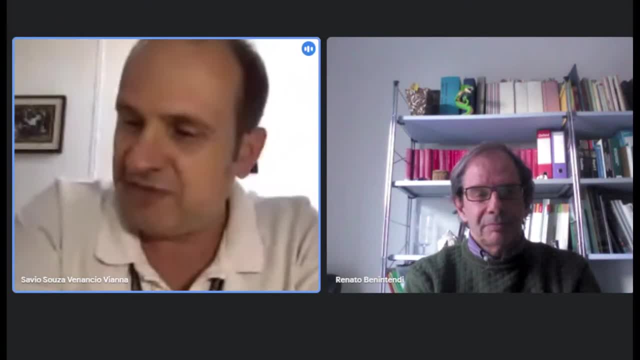 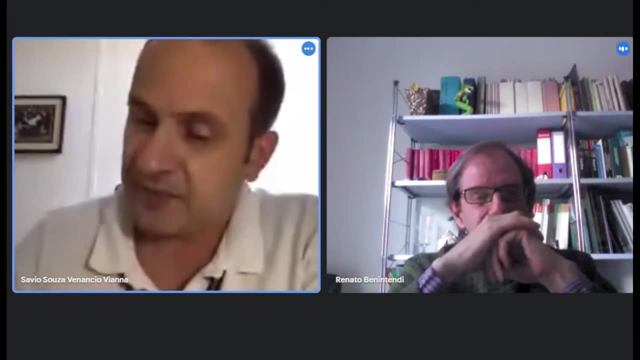 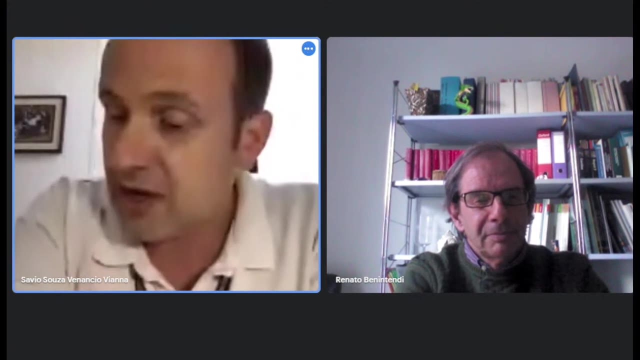 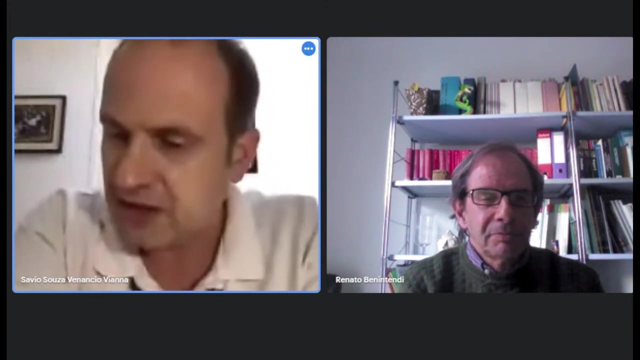 going to be pretty mixed, But the first one goes like this: One of the students- undergrad students- is asking, as far as the fluid dynamics is concerned- probably he's taking this course this semester- how important is the basic fundamentals of fluid mechanics in the context of process safety? 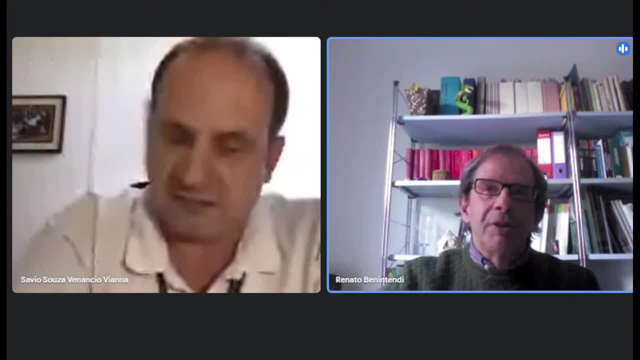 Yeah, it's a very good question, Fluid dynamics in particular. Saryo, yes, Fluid dynamics. OK, It's a very important question. Sorry for not addressing this Iriane, But I was very careful about your time. 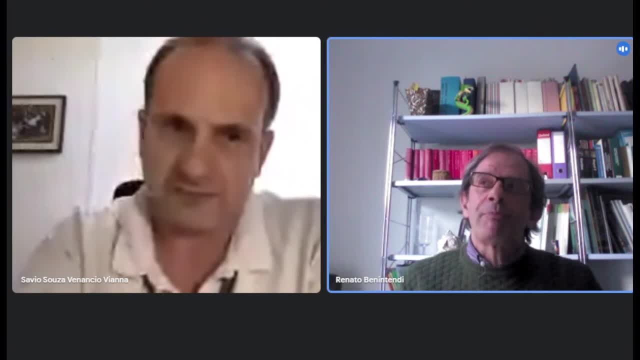 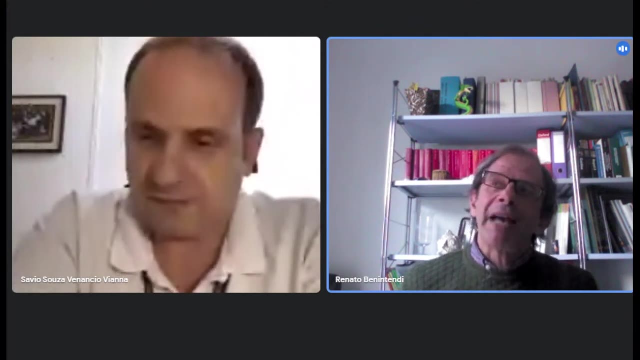 So, as you know, because you have been a very, I hope you have been able to use my book to sleep very well all night. But in reality I dedicated my first six chapters of the book to fundamentals Because I found out that in reality, even 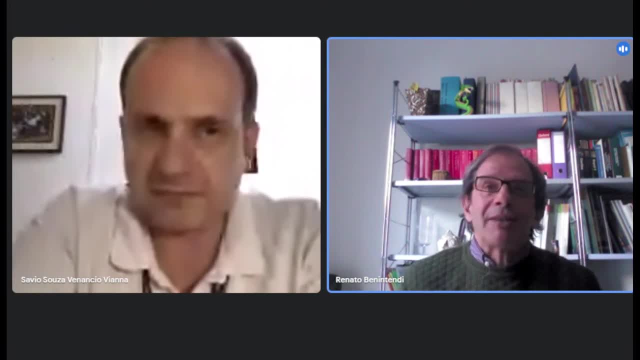 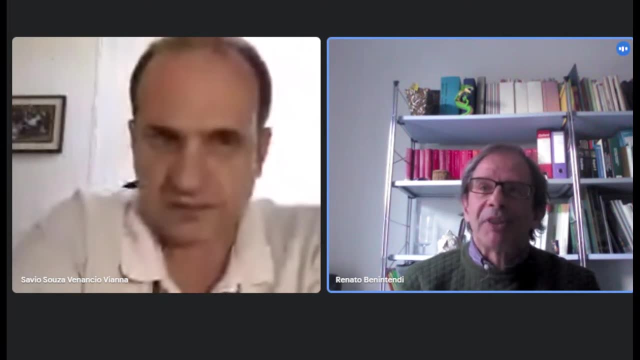 if we are chemical engineers. so we essentially have just a kind of background preparation that should cover everything. But in reality there are two possibilities. There are two points. The first one: some specific subjects are not probably necessarily just for economical reasons. 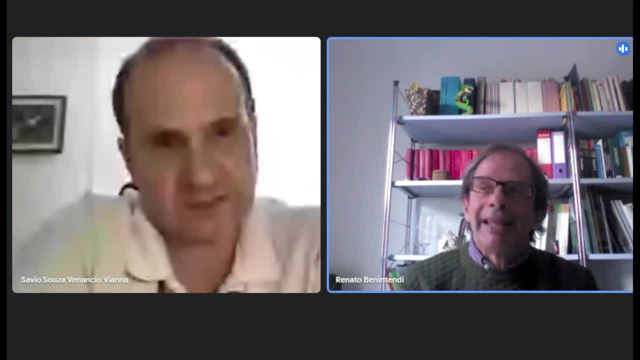 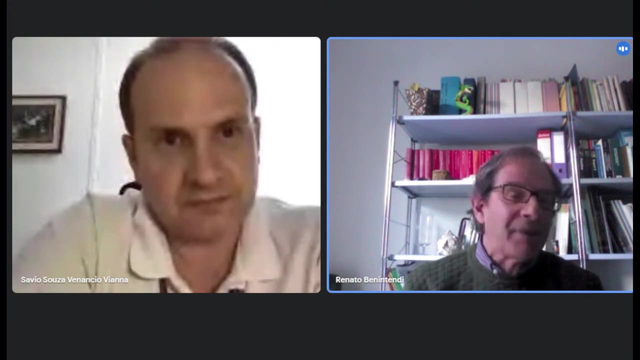 not completely covered during the studies And, the last but not least, some specific chapters are not specifically addressed to process safety. One of these, for sure, is fluid dynamics. Fluid dynamics- OK, I graduated more than 35 years ago And so it was very robust. 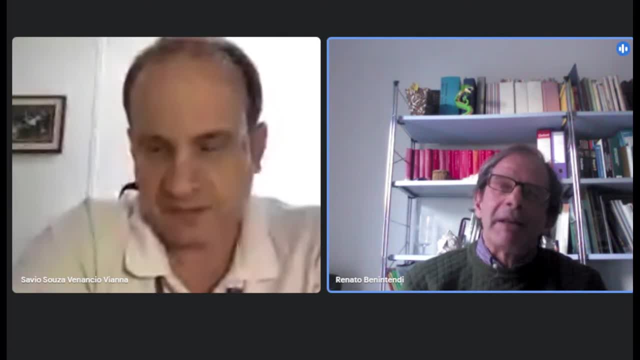 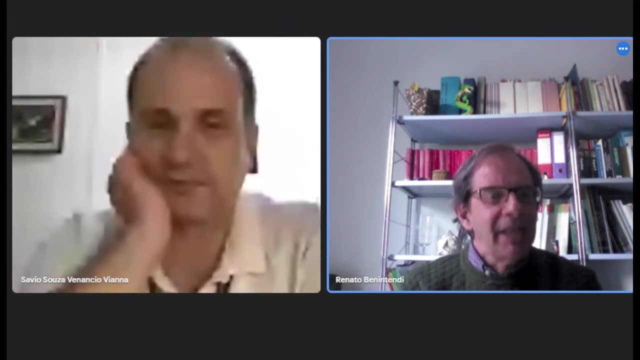 And five years in Italy. It was very, very And I remember I had a very good preparation for fluid dynamics. But in reality I recognize now it is not enough. It would not be enough. It would not be enough for two main reasons. 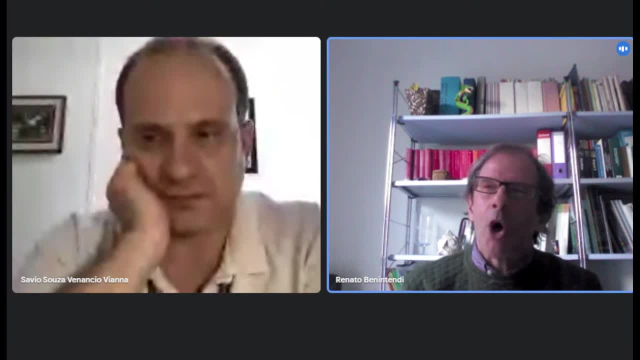 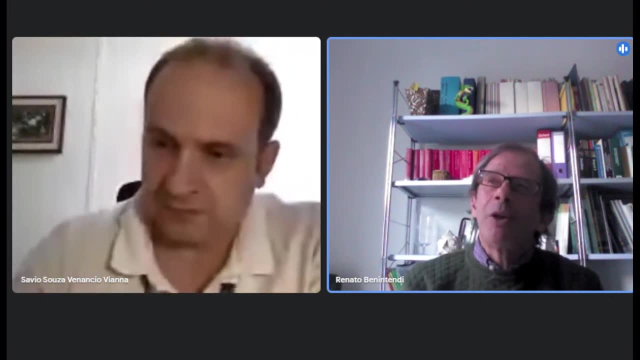 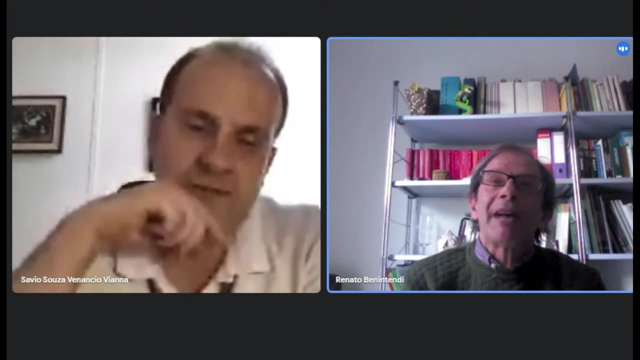 The first one is the complexity, absolute complexity, of the scenarios that we have to cope with. Let us not forget that normally we deal with release, So we have loss of containment, Loss of containment, Loss of containment, And containment means that we are essentially not. 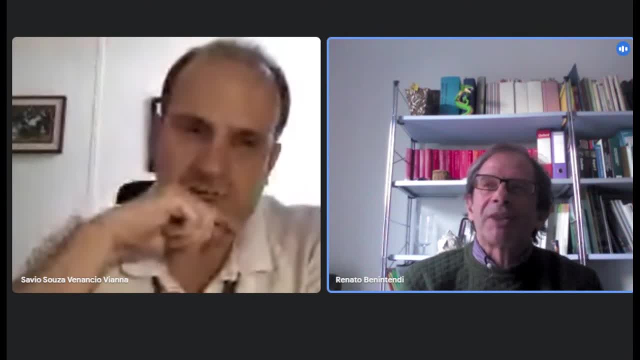 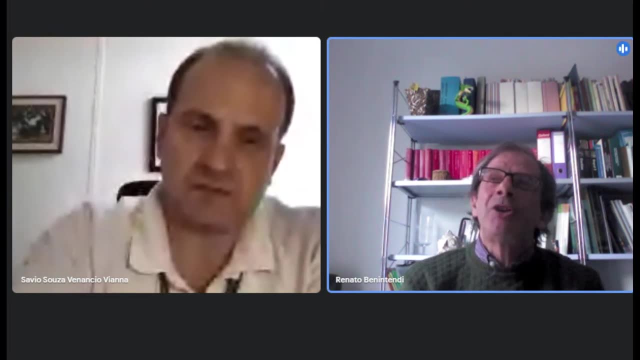 in the position to check, to control, let's say, the fluid dynamics regimes. We know, for example, how important are parameters like Reynolds number and the entrainment, And normally we have some specific regimes. after a release. We have the Mach disk. 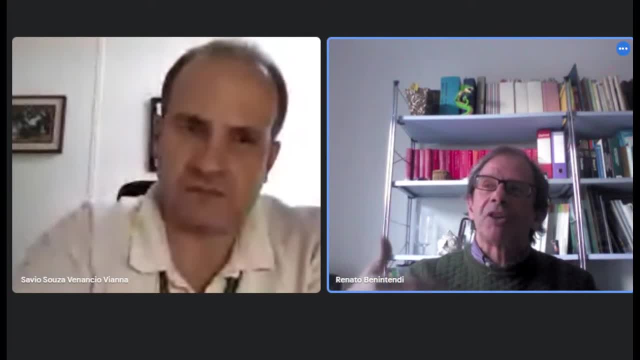 So we can have some specific speed that are higher than the sonic speed. We are hypersonic. So the gas dynamics, it is a specific, It is a specific, It is a specific subject of the mechanical engineers and aeronautic engineers is important. 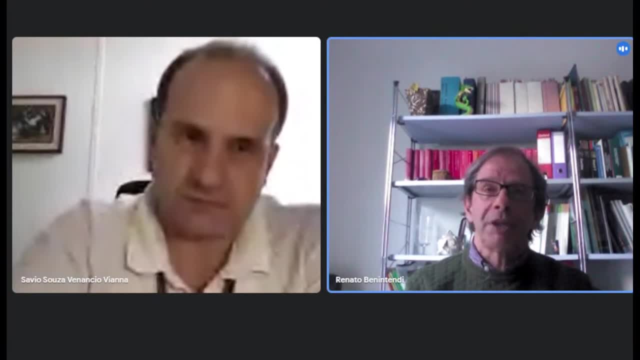 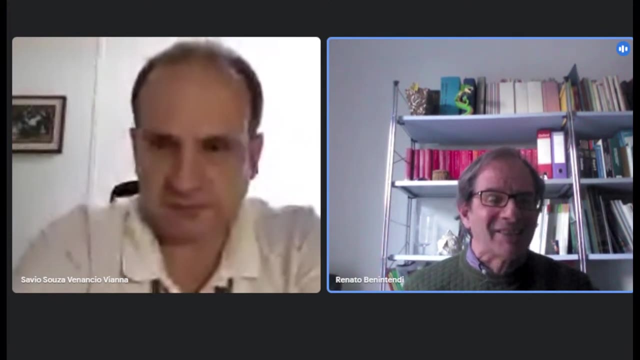 I had to go into the gas dynamics in order to become familiar. And then you have to consider that you have to quantify what happens after the first five meters. the second five meters, You have to consider how important is the dense gas. Sometimes you can have essentially a gas that is ammonia, but after the release it's very. 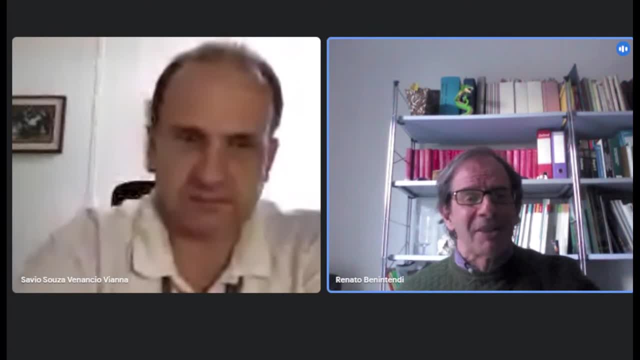 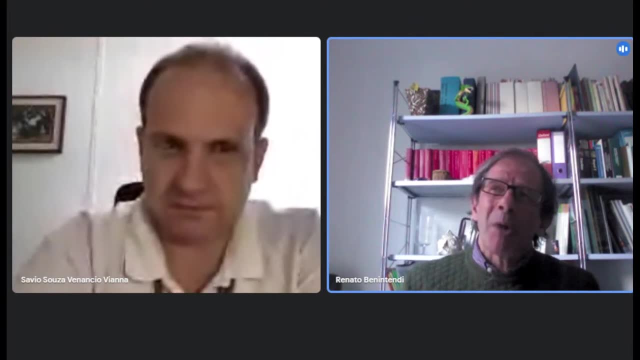 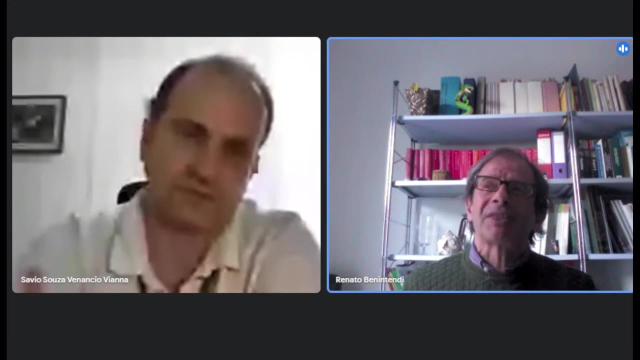 cold. It is lighter than air, but in reality it behaves like heavy. So I would say it's a very good, good question. I probably would say that the fluid dynamics is one of the pillars, particularly if fluid dynamics, let's say, tie into process safety. 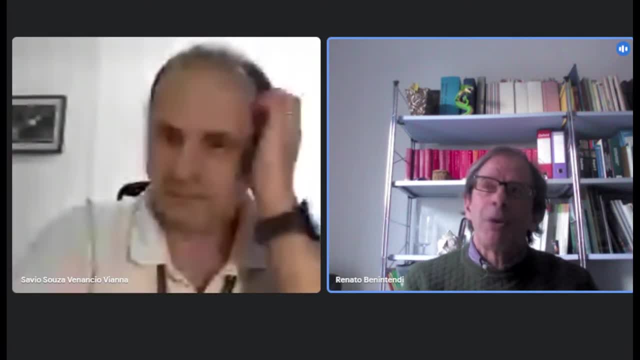 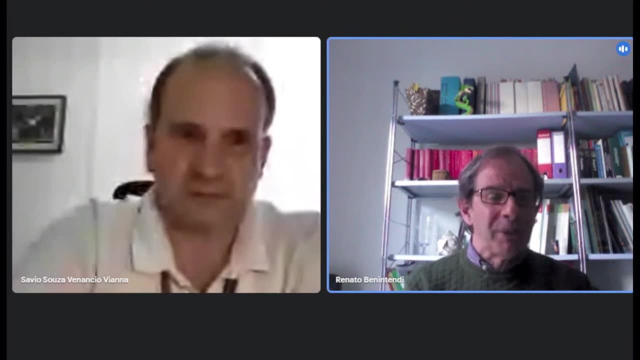 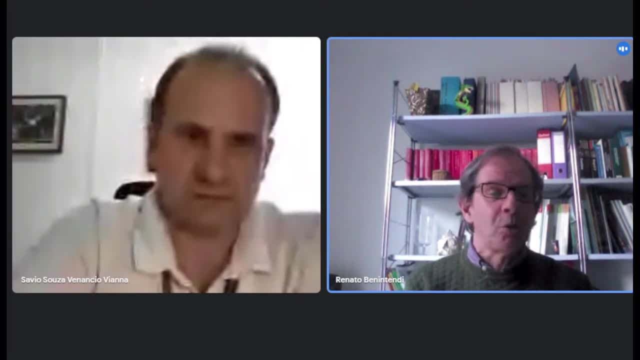 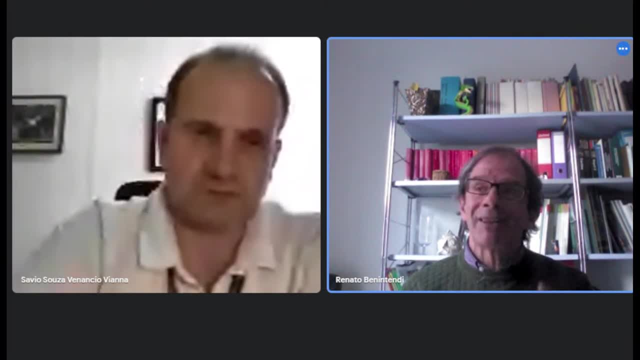 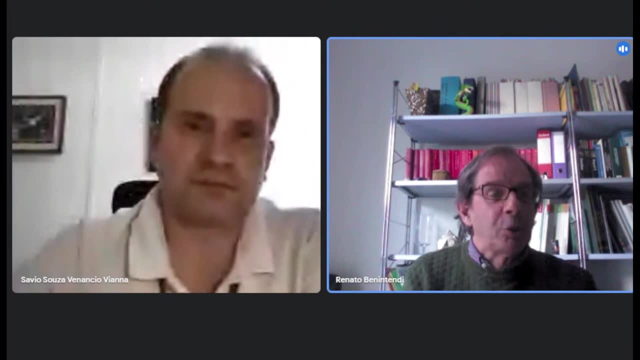 And this happens also when you run softwares. A software sometimes- because software software is is just, is a car, It depends on the driver. If you have a good driver you can have a good response- And sometimes the software, even if. even if they are good software, they cannot cover. 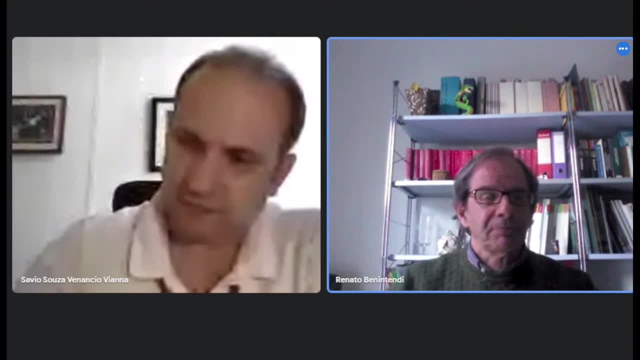 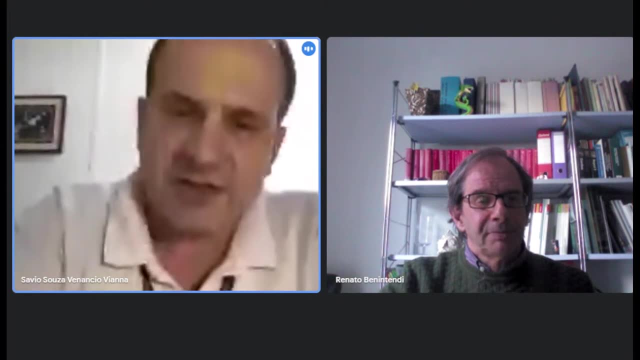 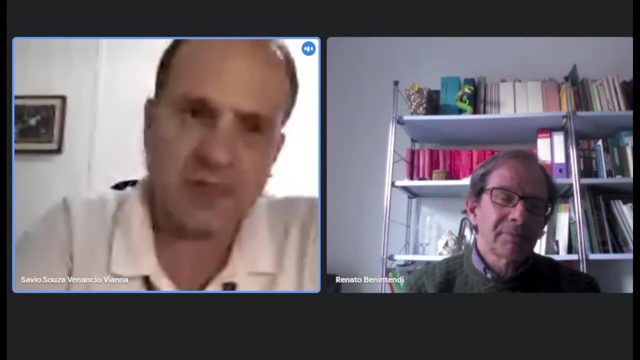 all the fluid, dynamic notions. Yeah, indeed, Yeah, Right, Yeah, I totally agree with that. In the same subject, Renato, as you mentioned, your book is a reference book in the Process Safety course here, so we use it throughout the course. 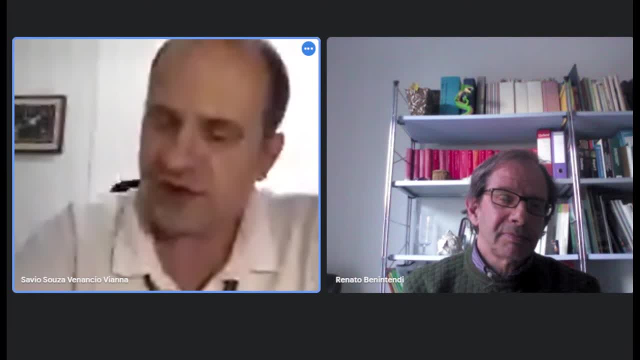 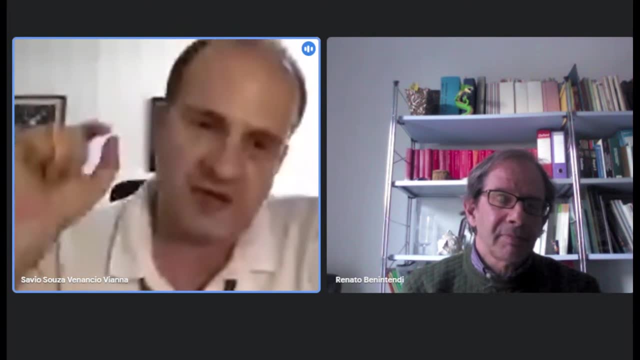 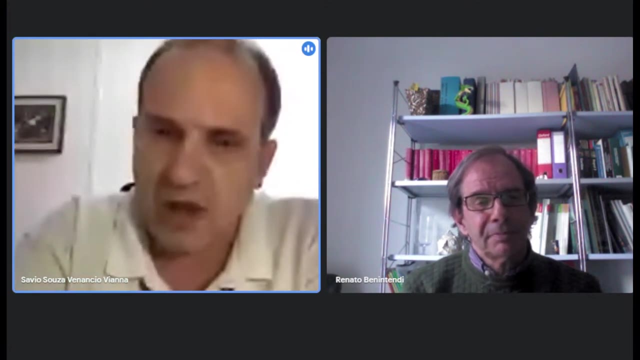 And one of the students just called my attention for the bell, for the bell shape that occurs in the region very near to the leak orifice. And then his question is: when you go and you try to model gas dispersion using CFD, quite often we ignore the fluid dynamics in the region very close to the leak. 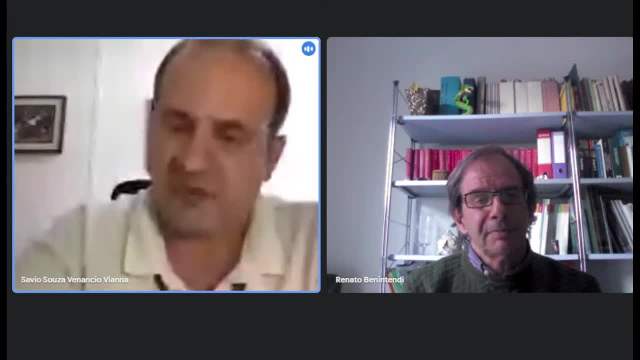 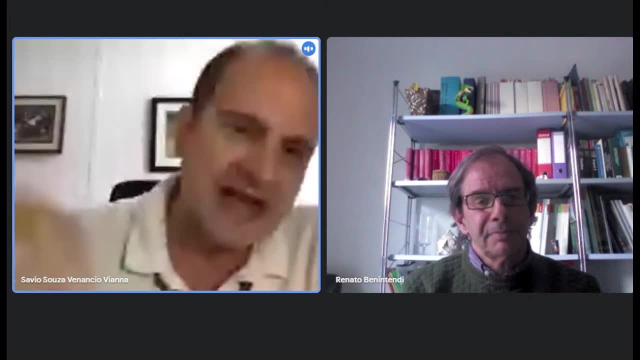 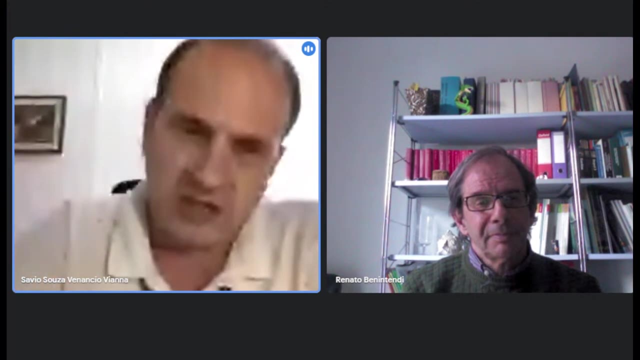 where this bell shape is formed And we kind of move the boundary condition a little bit downstream. the release, because we are, at the end of the day, interested in the gas concentration as it disperses and not in what is going on in the region close to the orifice. 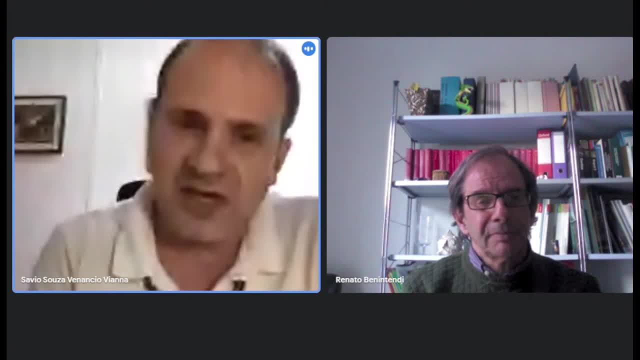 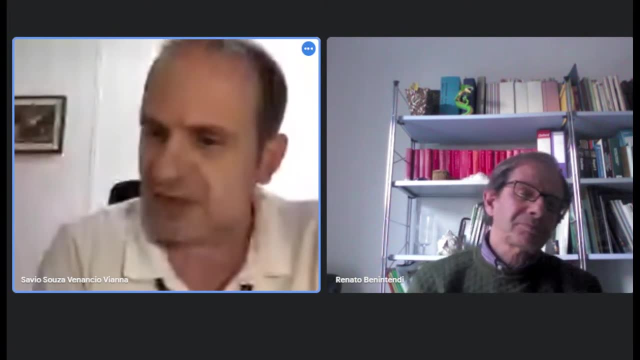 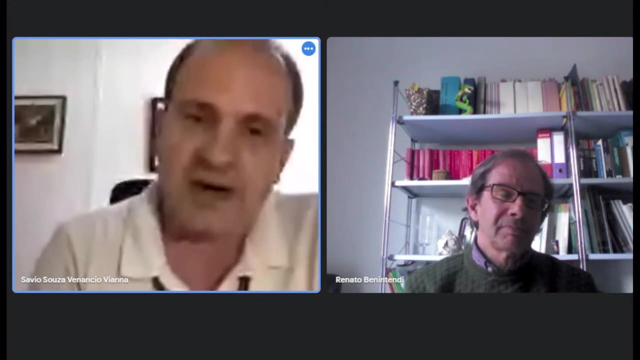 So, in that sense, in your opinion, do you think that the modeler that's operating the software is- let's say, it's- committing a very big mistake in ignoring this bell shape, or it's something that needs to be taken into account when modeling CFD scenarios? 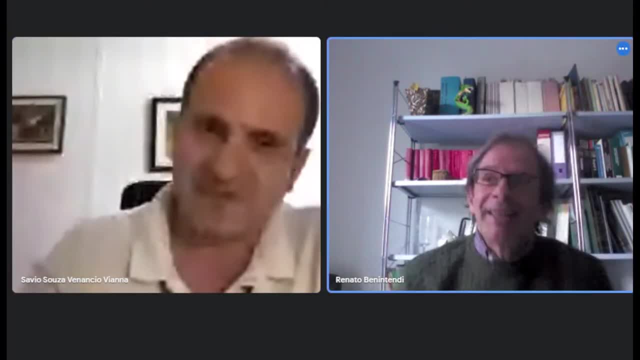 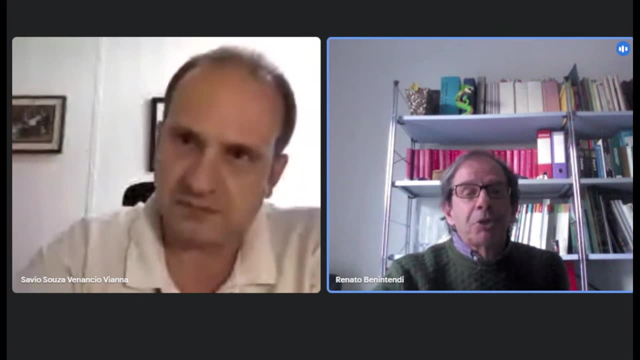 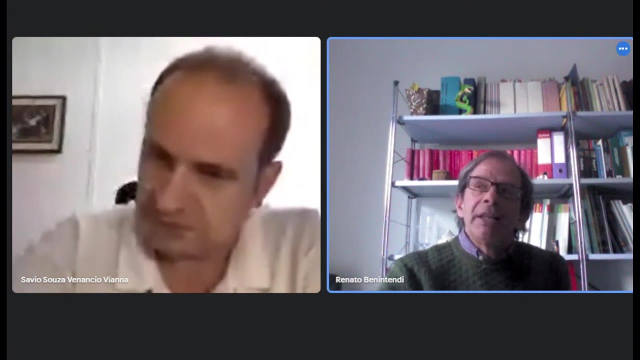 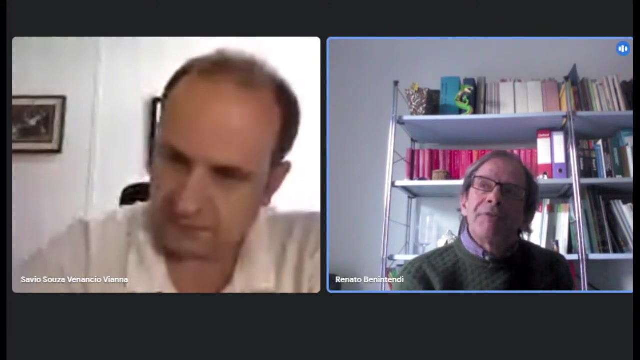 Okay, It's a very specific question because we are zooming the part of the release that is, in reality, very close to the orifice, And you know that we have. essentially, we have a distance over which very complex and somehow unpredictable phenomena happen. 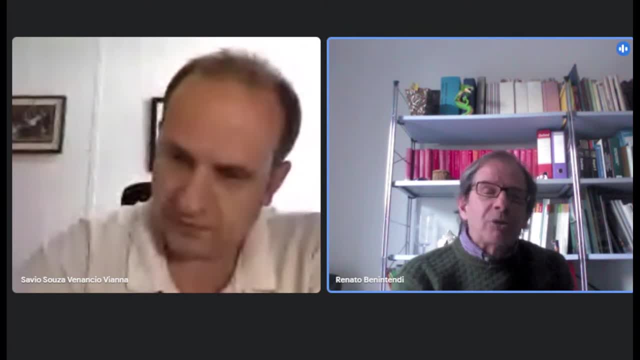 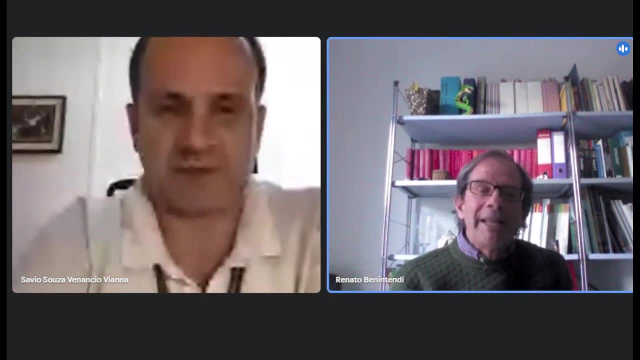 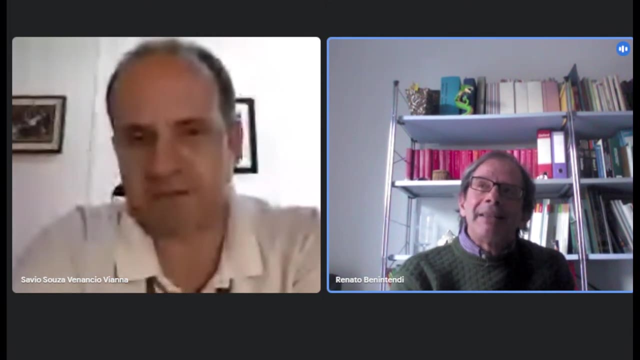 I have tried to anatomize, no To characterize. I have tried to create a kind of anatomy of what happens when you leave the structure, the pipe, the tank And in reality I think that you can be affected by significant mistake. 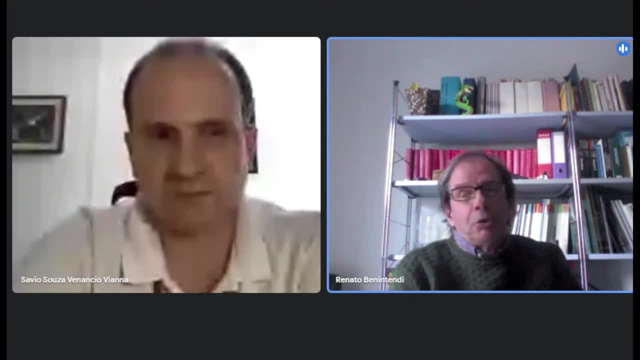 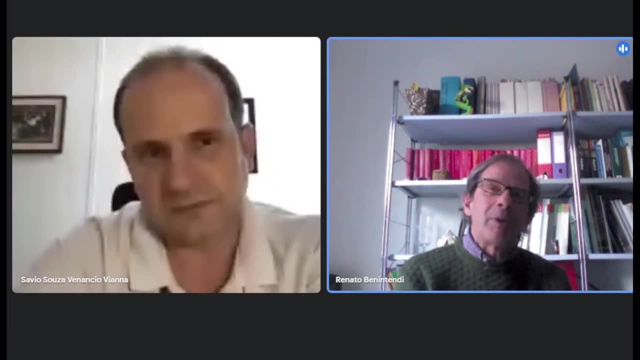 Of course, it depends on the liquid, on the fluid that we are managing, Because, of course, for example, just in order to provide you with an example, I will not mention, of course, the company And I will not mention the client, of course. 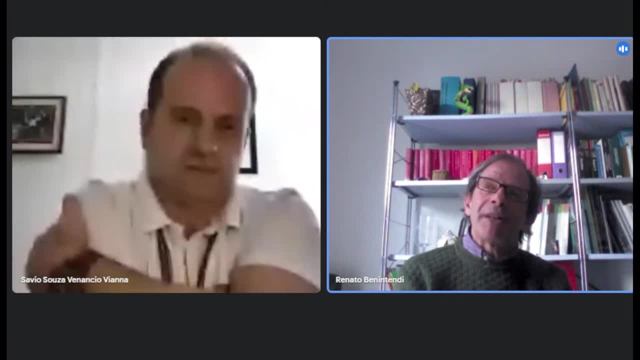 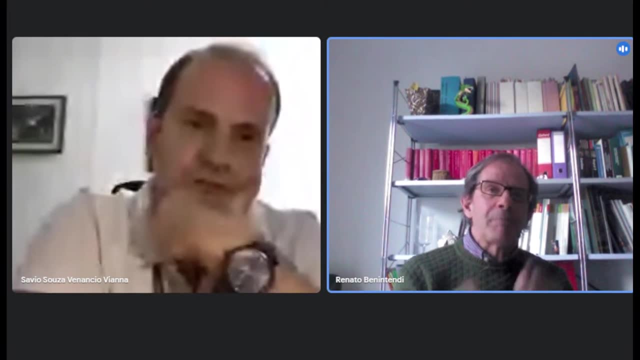 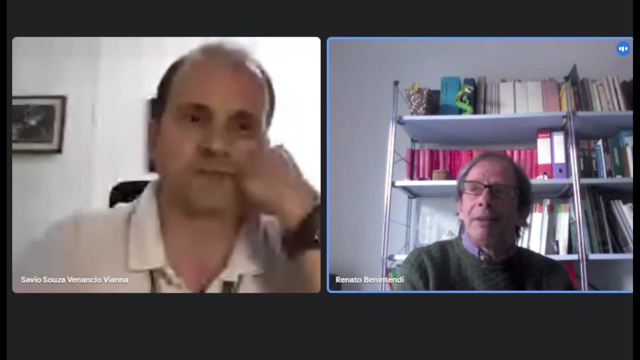 We have seen, for example, that there was a very important project in the Middle East And they modeled it essentially with an important software. I don't mention software, for that I don't know how did they, let's say, manage the software? 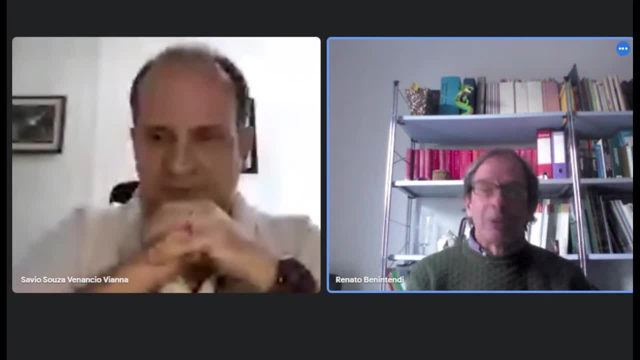 So probably I don't know if the mistake that we found. I don't know how they managed the software, So probably I don't know if the mistake that we found, I don't know if the mistake that we found. 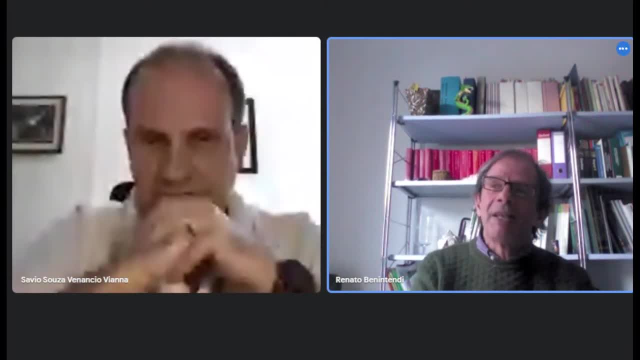 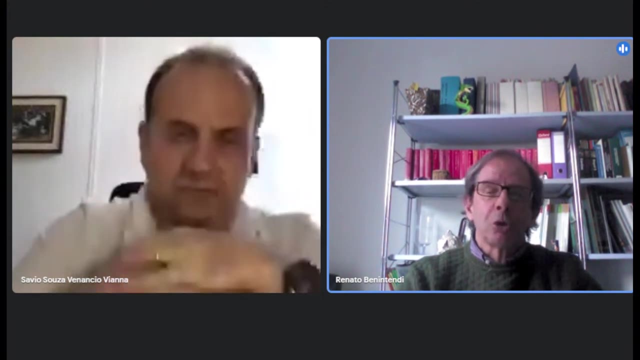 was related to the software or was related to the way they. But in reality they found that HCN- liquid HCN- had been just released And the temperature was down was so low to reach minus 40. That was absolutely impossible. 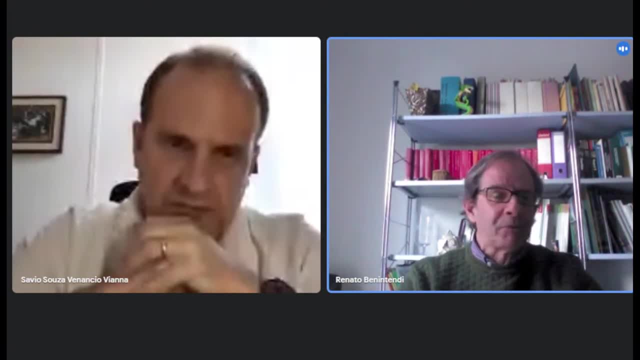 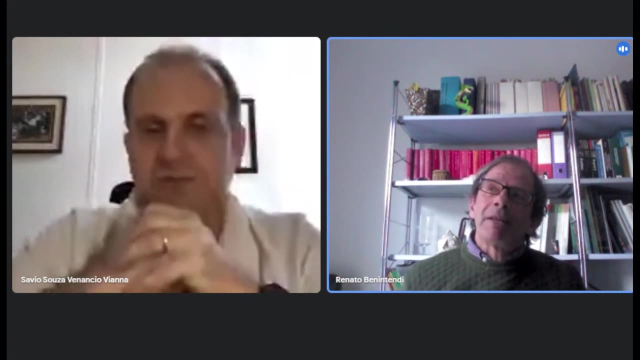 Impossible, because this can happen, for example, for APG. So I would say, generally speaking, if you carry out a CFD study, I think you can be. of course, you can be probably entitled to have some more words. 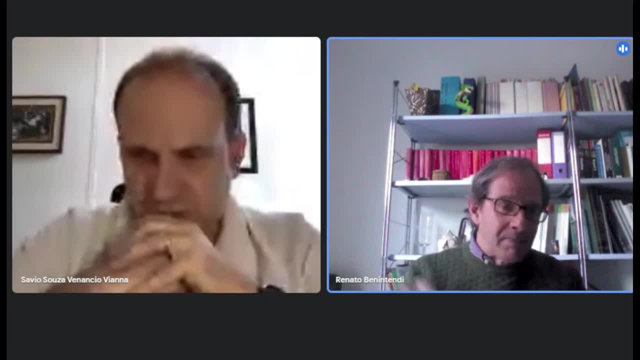 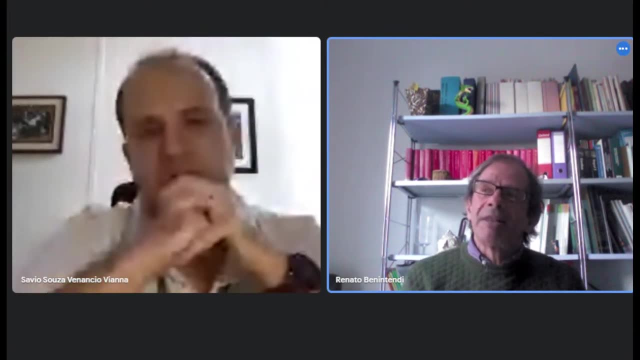 if you compare to the use of software. For what regards the bell shape, particularly the bell shape, you know that in the book you can find, in the literature there is a big discussion about you can find essentially some specific validated. 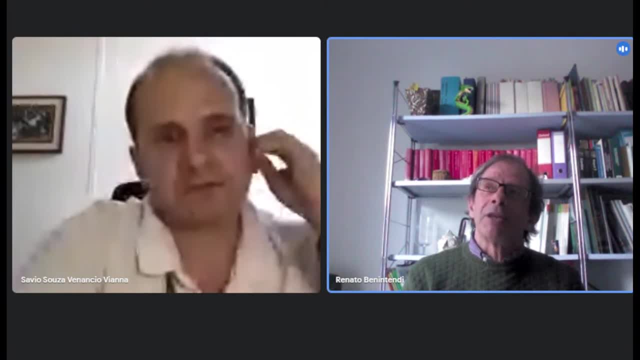 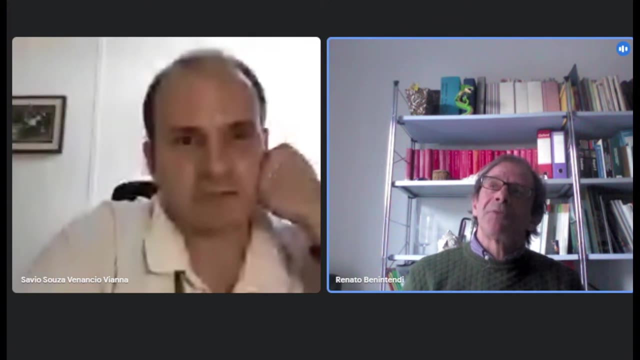 range over which you can assume that you can have essentially the development of specific regimes And, for example, CCPS provides some specific guidance, Because the problem is if you carry out just a CFD model or if you can use some software, or if you can use, for example, OpenFOAM. 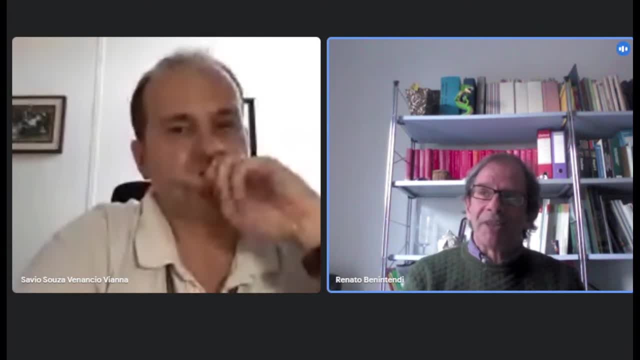 probably you can know OpenFOAM, that is, if you can use, for example, OpenFOAM. Probably you can know OpenFOAM. that is, if you can use, for example, OpenFOAM is probably the only one CFD tool that can be comparable to Fluent. 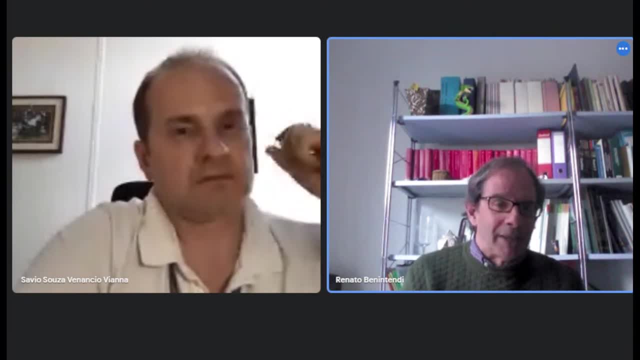 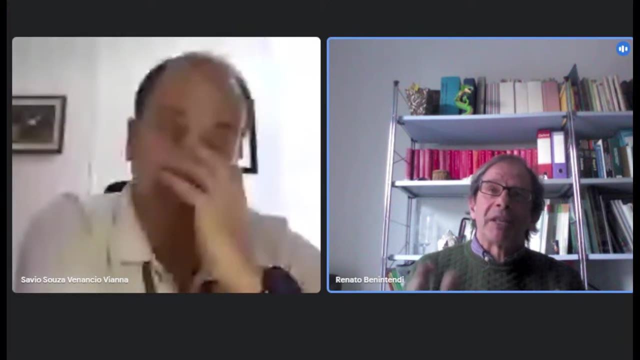 The thing is that you have to validate what you are doing. That's the problem. So if I speak to you as a process safety engineer, as a process safety manager, I must validate your final conclusion. We know that, essentially, we have some specific range. 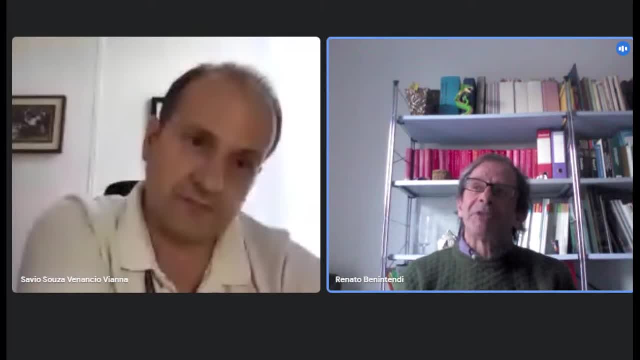 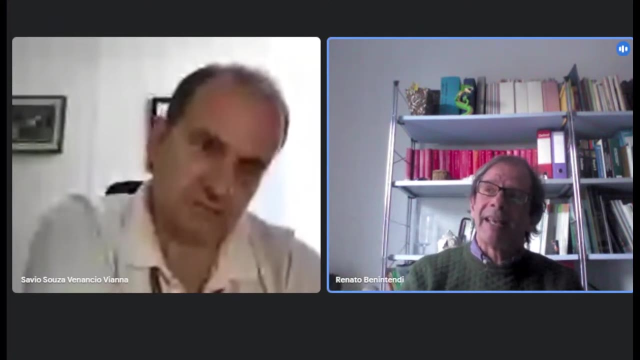 over which you have the MAC disk. After the MAC disk you enter, that is, the underexpanded zone where you can exceed the sonic velocity, the sonic speed. Then after that you can assume that you have essentially just the sonic velocity again. 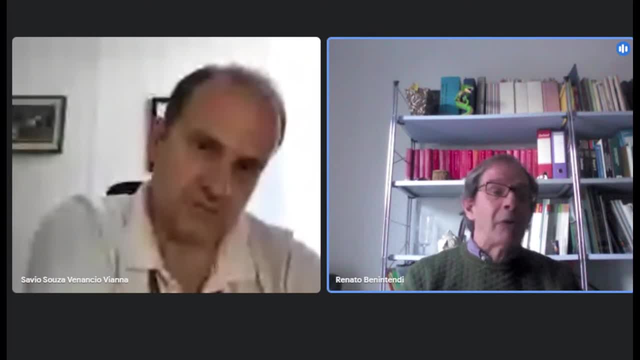 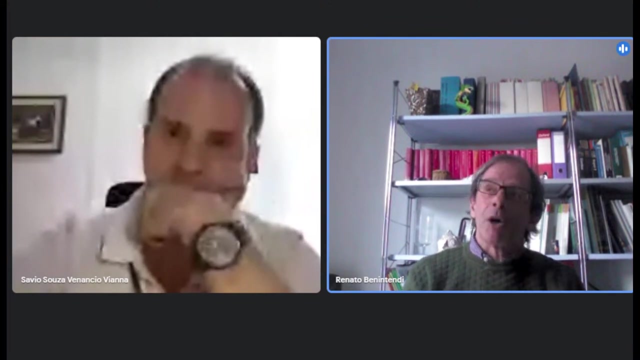 that you can reach the Gaussian zone. The mistake that you can. of course you can be affected by a mistake, depending on the assumption that you do. The problem is that the complexity can be very high Because normally when you carry out the fluid dynamics calculation, 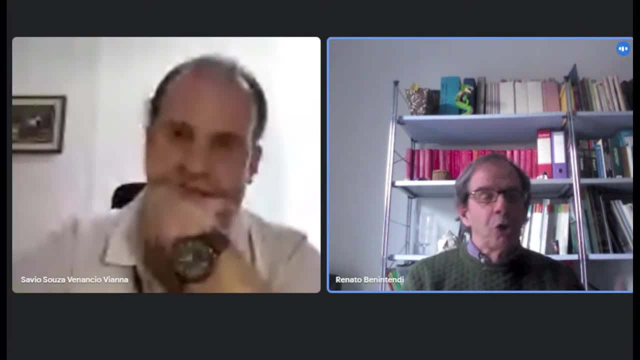 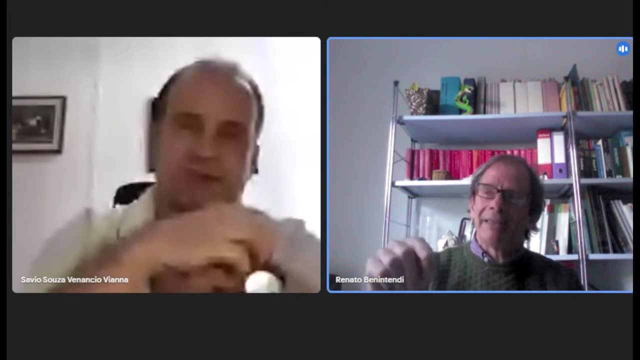 you must consider the thermal effects. Normally you have in the book you probably find, let's say, the profile of the concentration, the profile of the temperature and the profile of the velocity, And you have to come together and it's not easy, of course. 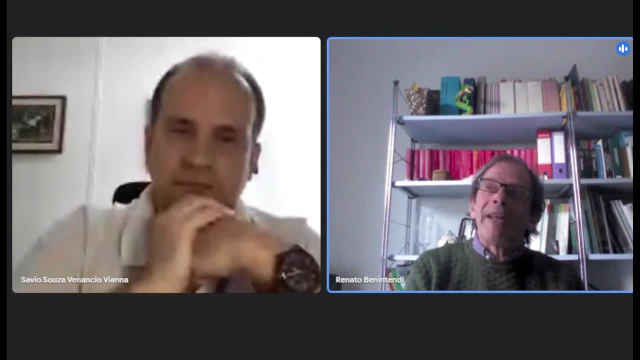 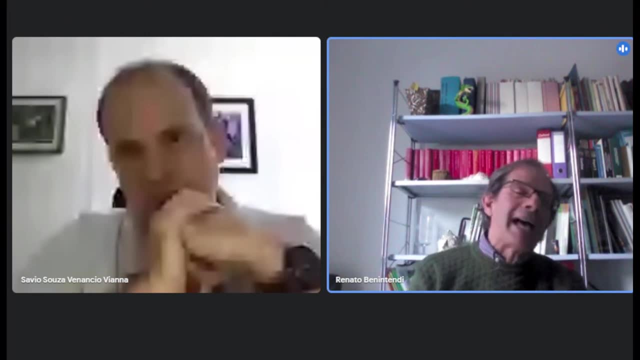 to have a regular approach for this. So when you are involved in a real project, typically you should comply with validated rules. Because the validated rules are important, because they are defendable. Otherwise, you must work a lot in order to. 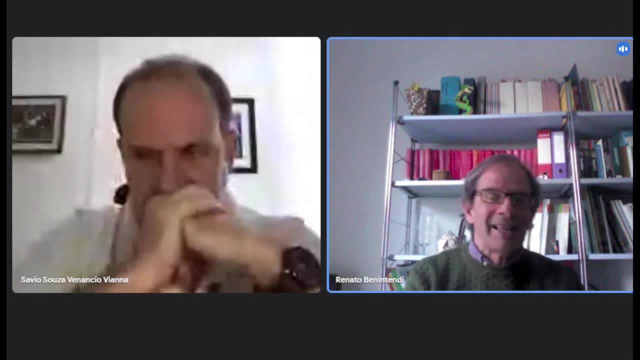 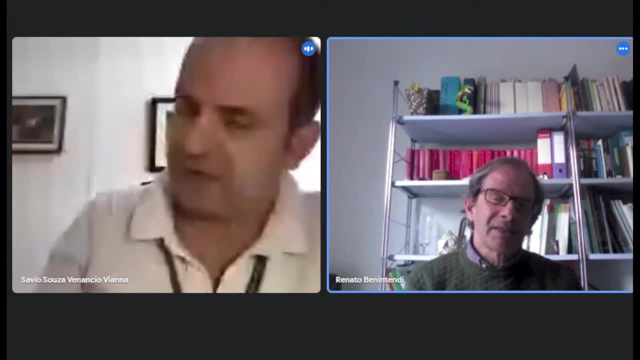 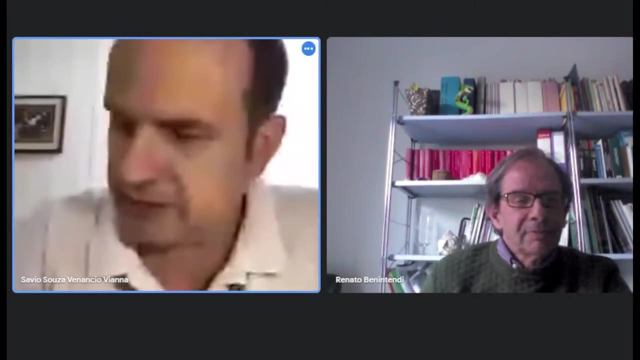 just to accommodate together the different profiles and the different parameters of your project, Of your work? Yeah, absolutely. There's a couple of other questions here. This one comes from one of my colleagues in the department where I work, And then she wants to know: 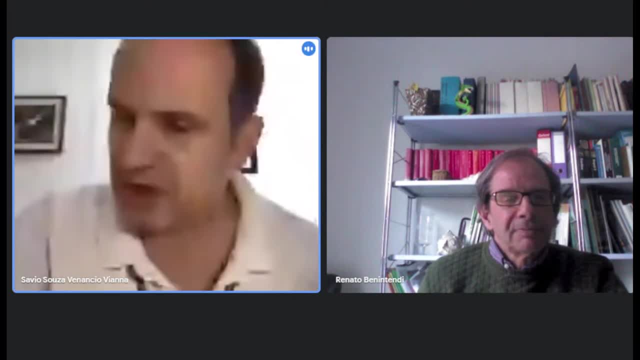 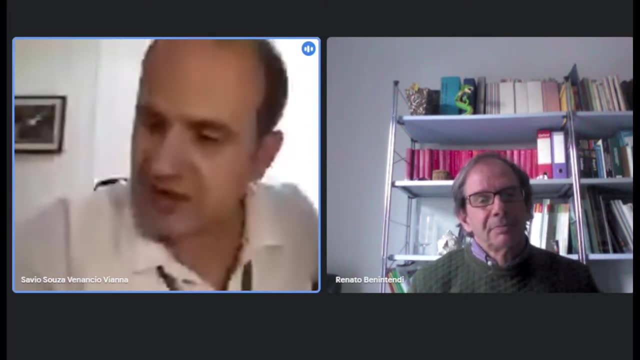 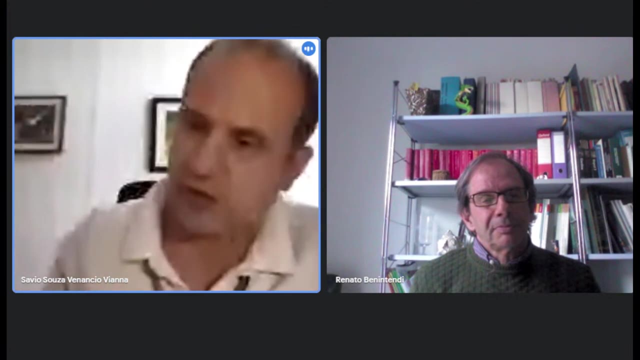 she wants to hear from you. She works with a process control, So she's asking, in your opinion, the advanced process control. what is the role of the advanced process control and how it can deal with process safety in your opinion? 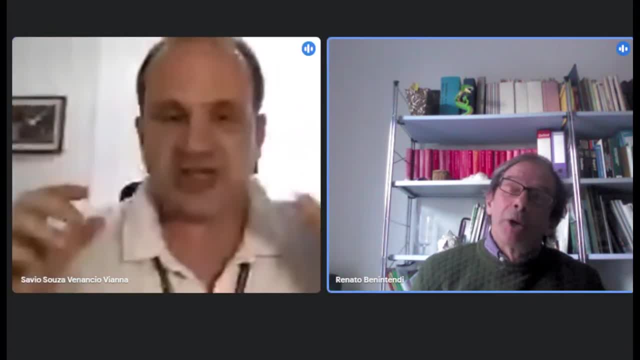 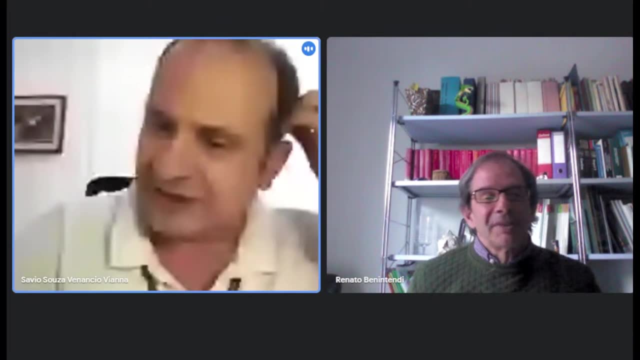 Okay, Okay, She mentioned just one second. She mentioned one more thing, Renato. She says what she really means is that, considering the process, considering that the process design can be modified, So you have something which is frozen there. 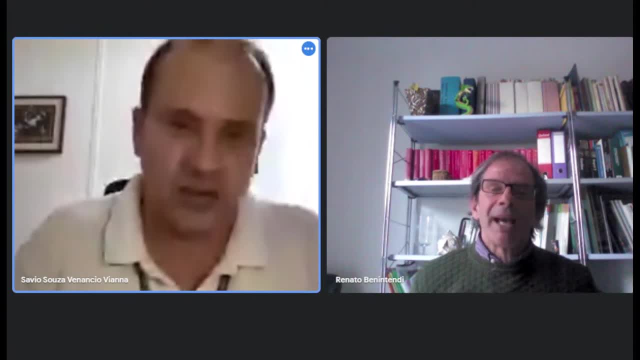 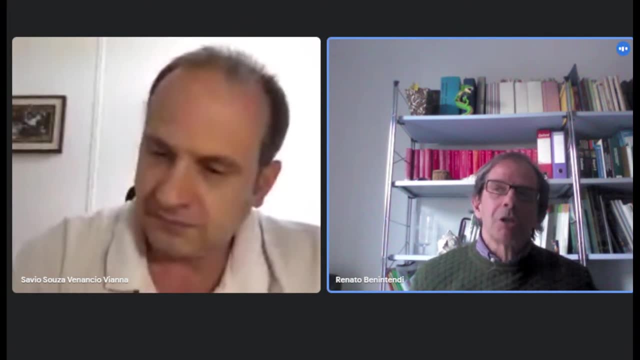 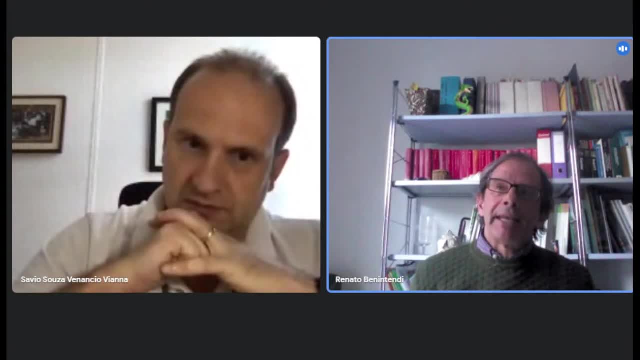 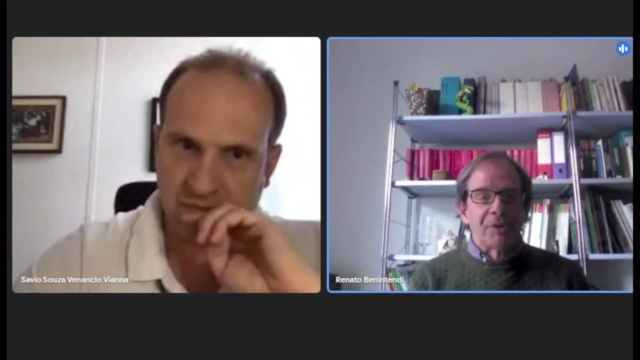 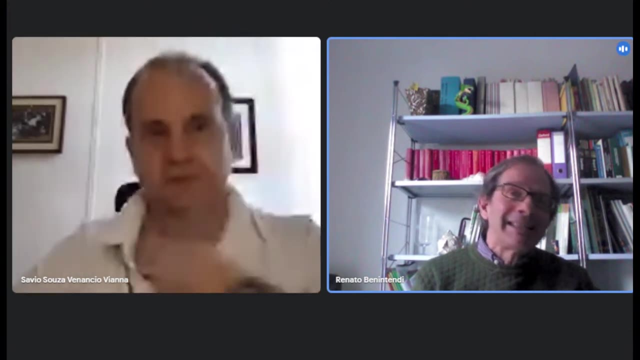 have become absolutely ordinary, And and and and I would say the relationship and the implication and the relationship between the advanced control and the process safety. the process safety are huge. The I I think this is. I could be wrong. 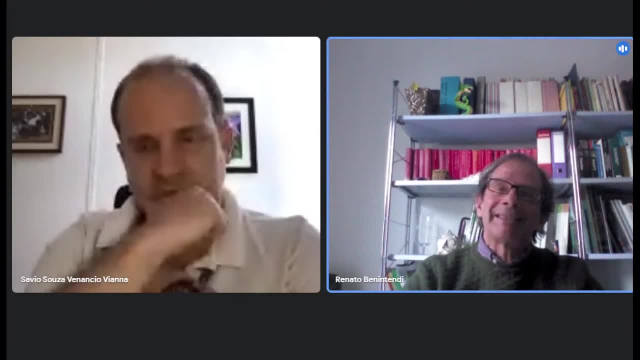 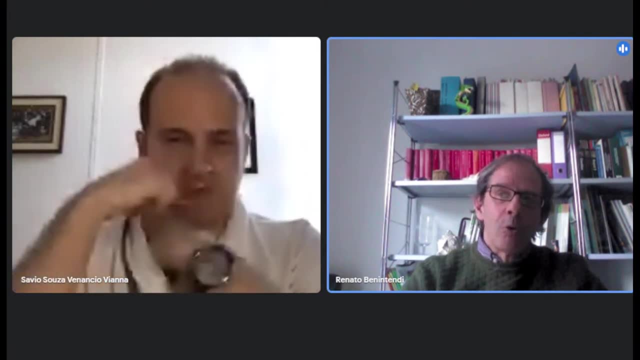 or I, or I could be partially right, But I think that, in reality, we, when we, when we carry out a SIL review, when we, when we, so when we are, when we are, we are involved in SIL allocation. 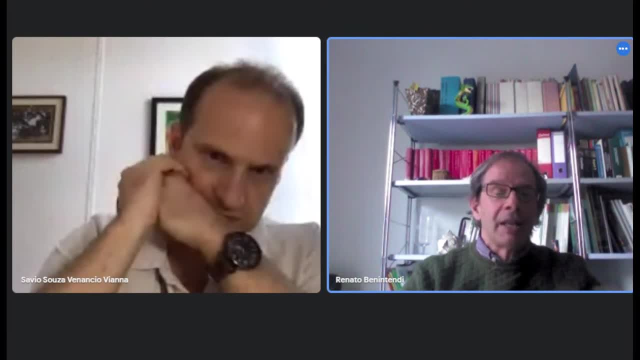 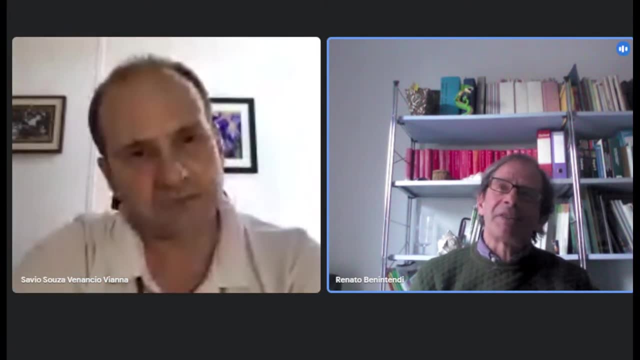 And and so when we are involved in loop, in in in complex loop architecture, normally, normally this this is carried out in in a very, very automatic and ordinary way. But in reality I have been involved many times. 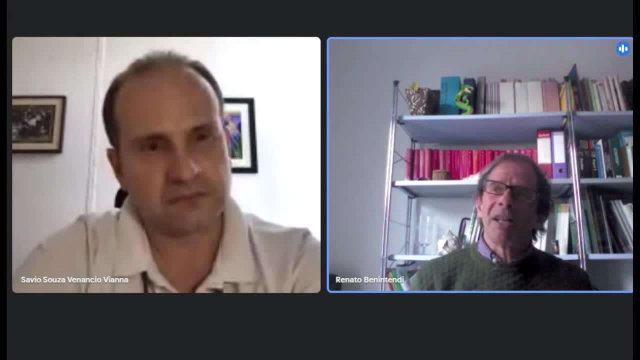 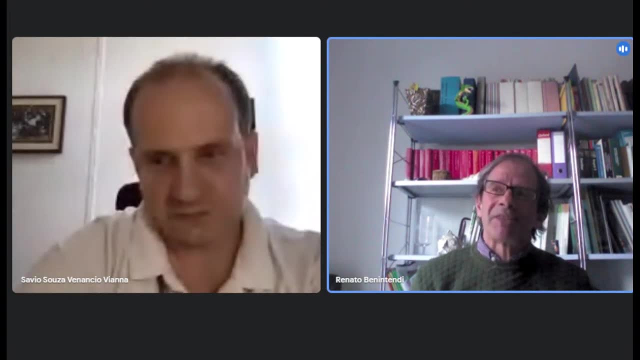 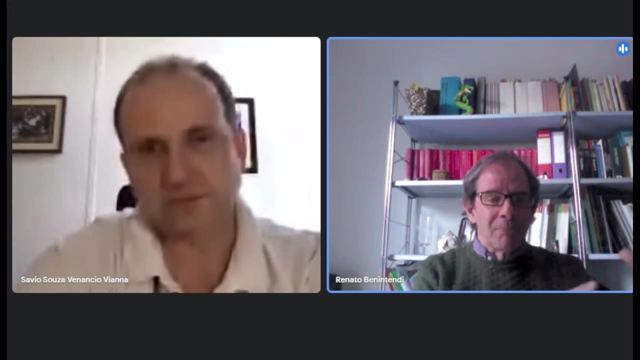 in specific question coming from from instrumentation, people, and, and and and automatic control. that forces myself to to have a specific focus entering the, the, the, the, the control architecture, much more than typically you can expect to have in. 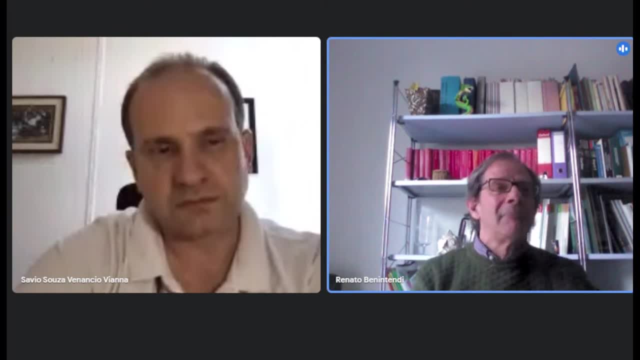 but especially for process safety engineer that are very clever managing the, the, let's say the, the, the functional safety in terms of the application of, of I don't know- and and the other software. But when you have to carry out the, 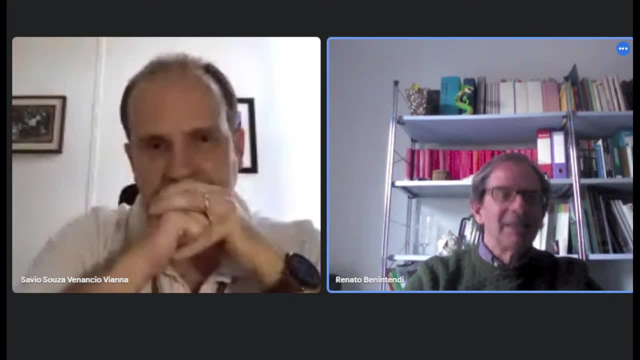 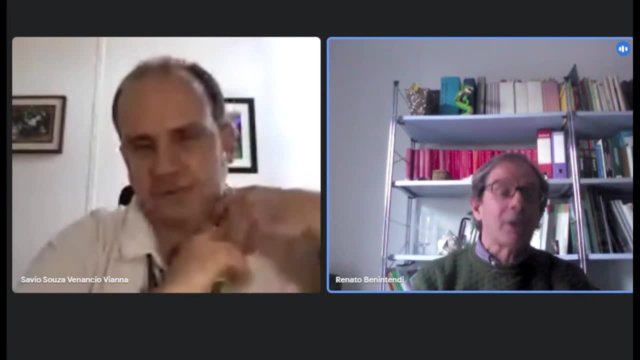 the, the, the, the reliability, the, the reliability exercise applied to, to, to, to complex control and and and advanced control is completely different story. So I would say it's very important And I would say that implication are huge. 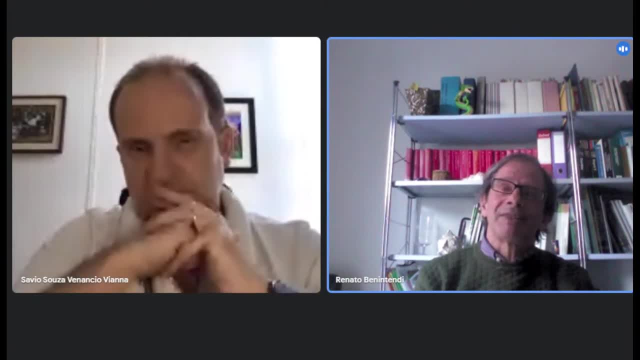 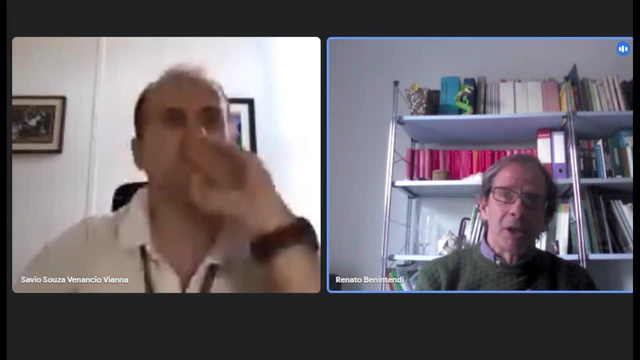 I have tried to explain why is the, the, the, the role of the process safety engineer so so difficult? And and and in my opinion, I have been working in the, in the in the last 10 years as the knowledge. 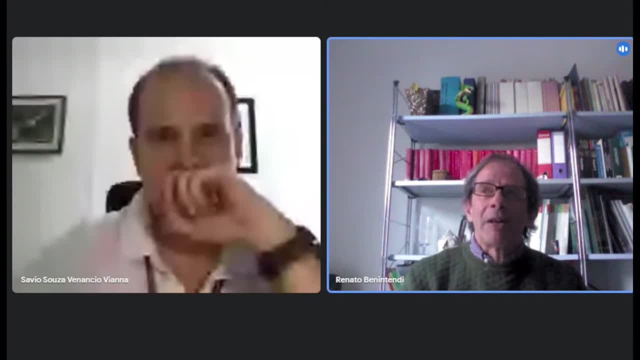 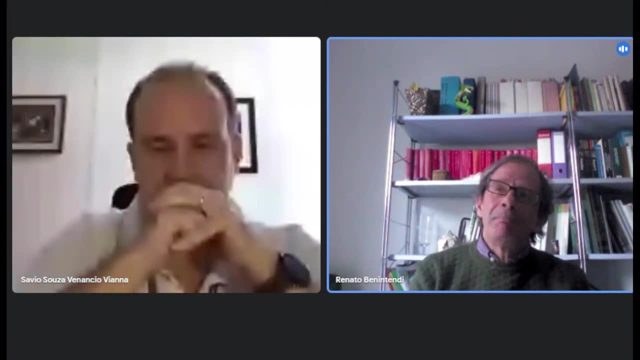 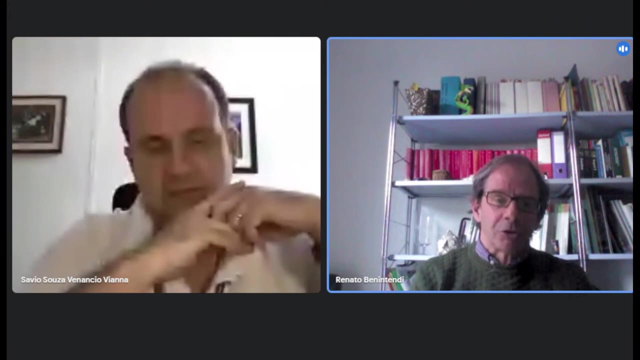 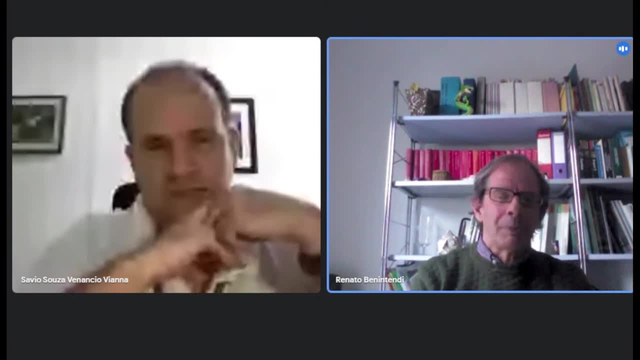 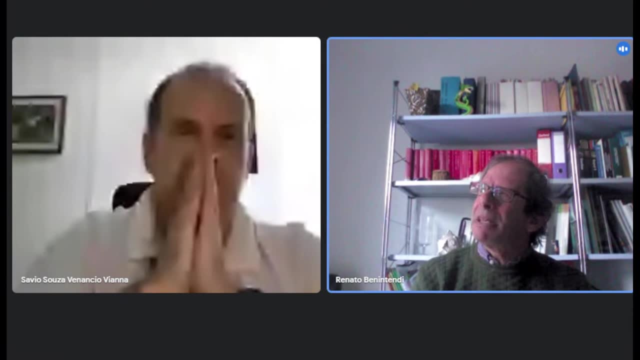 Oh, I get it. Yeah, The investment tool piece, the, the, the, the also should have taken away from the real. Yeah, It's a good question, but I, I, I think that this might be not all. I have just looked at. 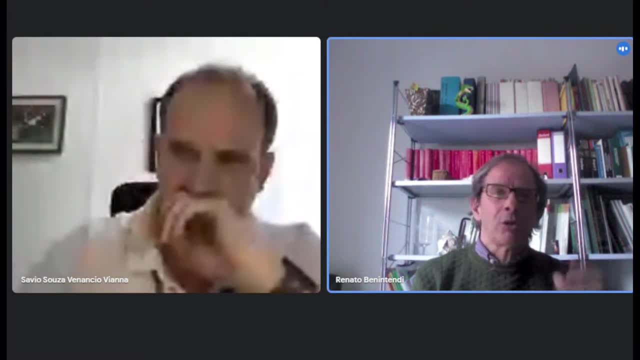 Uh, I was looking in my in in my into this part of the world and we we found a lot of of areas that were not very clear, so I would say that is very important. this and sometimes is not covered by by process engineering, but should be covered by- yeah, absolutely. 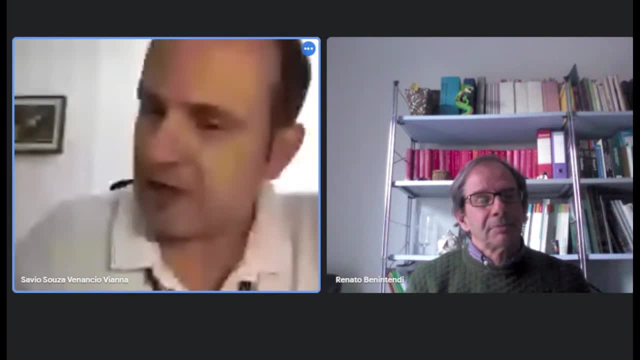 we have. we have one last question here, let me get it just one sec. it comes from one of the research student students. he's asking: in your opinion, what is the next step in the research as far as the process? a third, yes, okay, I'll try to. 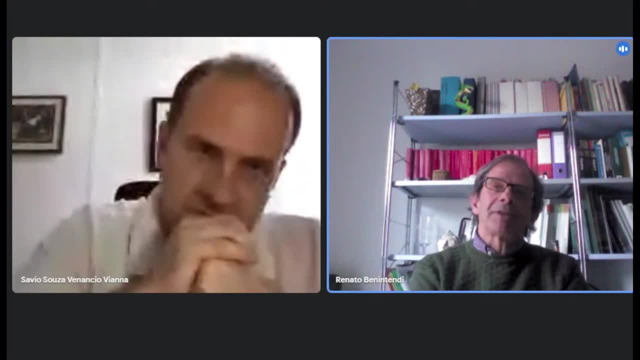 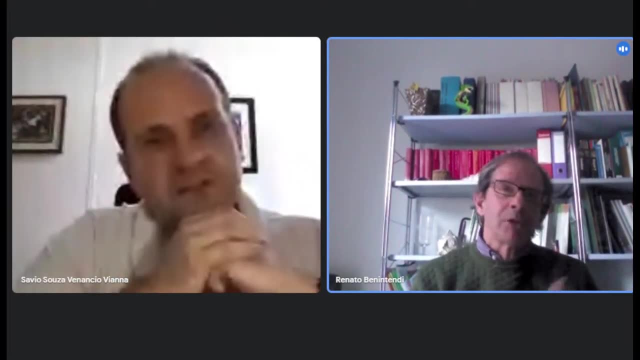 complete the okay, my answer, the answer that I have provided, provided. okay, it's it's a thank you. it's a very good question. it's it's it's a very happy to be able just to brainstorm this. I my my my last slide was in reality, related to this question, because you 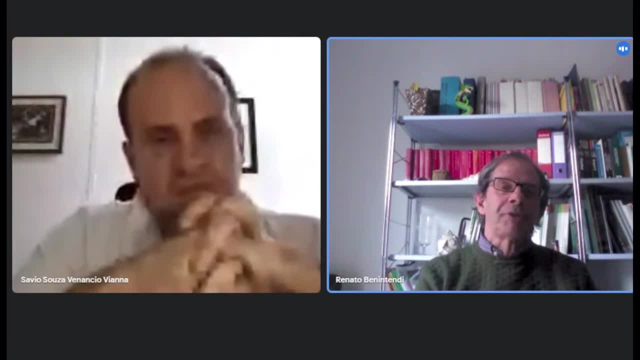 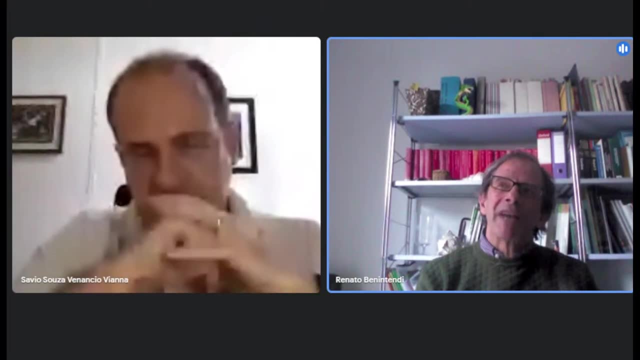 normally, you normally go to the, to the, to the ordinary route of a just process, safety, process, safety task. and we are discovering, we are discovering in the. I would say that the, let's say the- the rise of these, these considerations started first July of 2003. 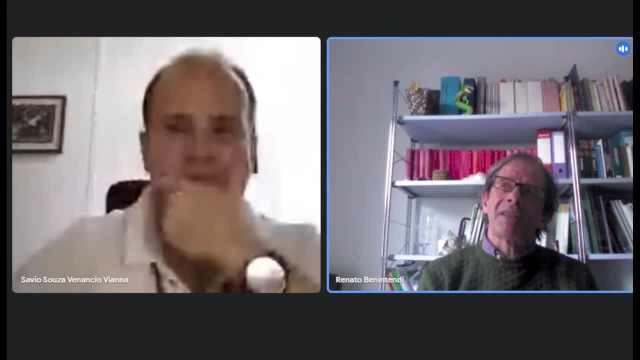 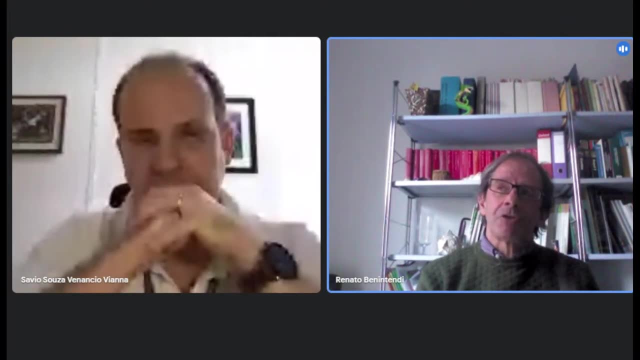 in the the first July of 2003, the 8x regulation was was implemented in Europe. all the, all the electrical engineers that they, they, they supposed that that it, the 8x, was just the, the new, the new, new chapter, not the new, the revised. 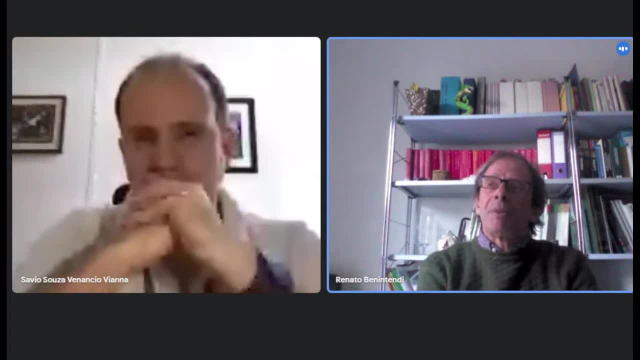 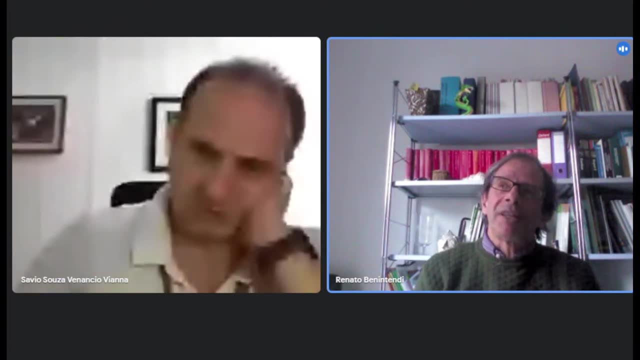 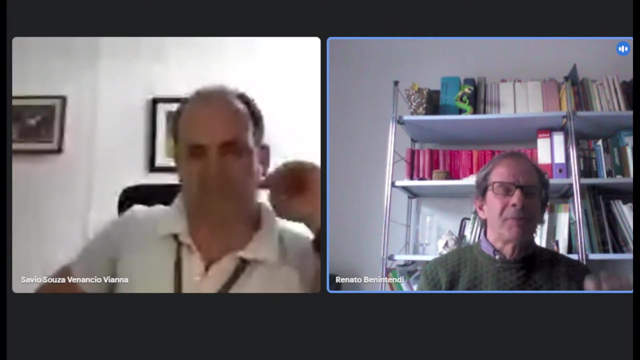 revised standard of the previous, the previous approach, but they were definitely wrong because the 8x is introduced is introduced as a comprehensive set of of of disciplines into the specific objective to prevent ignition and so it was completely different from the previous standard. just to tell you that, in reality, the 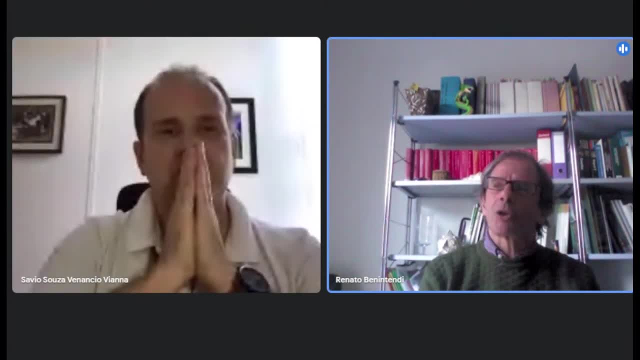 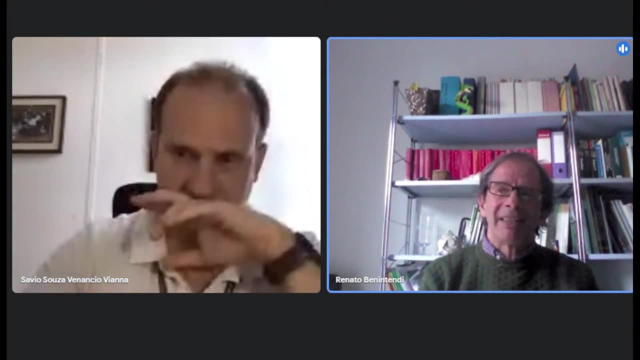 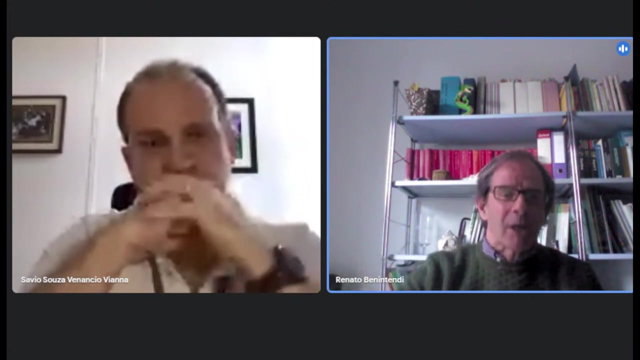 challenge that the regular, the regulation of the regulation you in Europe we had essentially, I don't know in the US and in in South America, but in Now in Europe, the regulation is forcing companies to move just to adjust their knowledge and just to speed up and implement research programs inside the companies, especially the manufacturing companies, just in order to comply. 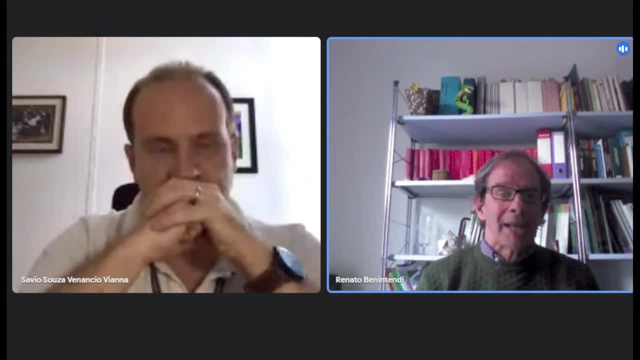 Because otherwise the production cycles are no longer cost-effective. ATEX is a universe. There was a sense, especially for the non-electric equipment. just an example: ATEX could be, let's say, the subject of a specific seminar. 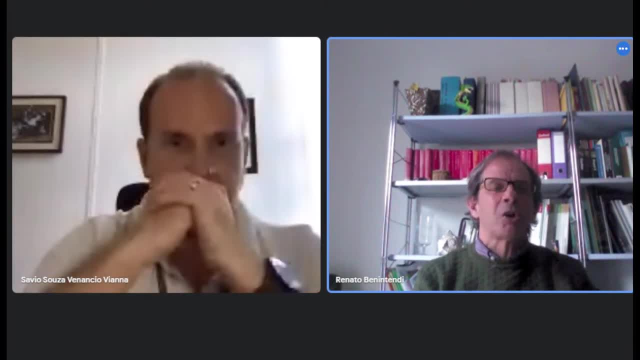 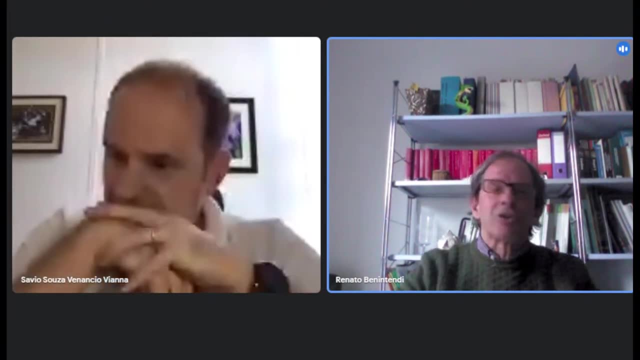 You now have to consider the Pelletier effect, the corrosion, just the, for example, the electrochemical behavior of material When you are just using, for example, gaskets or bowls and you discover that you have to consider, that you have to maximize. 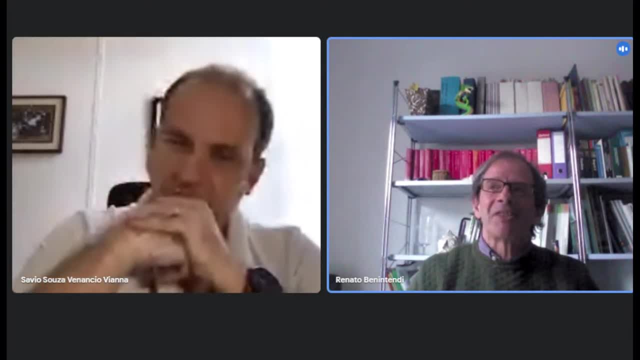 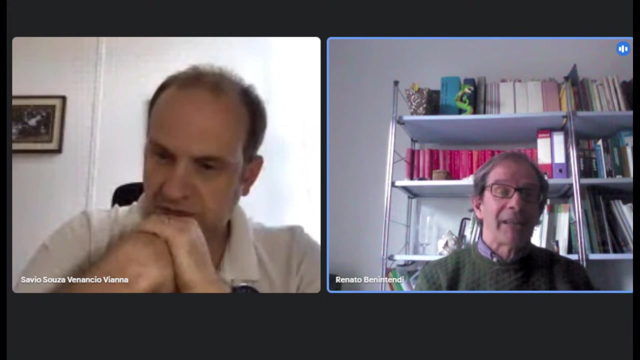 So this has resulted in overflowing a lot of new research. So I would say regulation, specifically European regulation. Why? Because from 2000, European regulation started with the new. there was a new approach, So we had Cerezo directive, Machinery directive, the Depression Equipment directive, CLP, Classification, Labeling, Packaging, and you have ATEX. 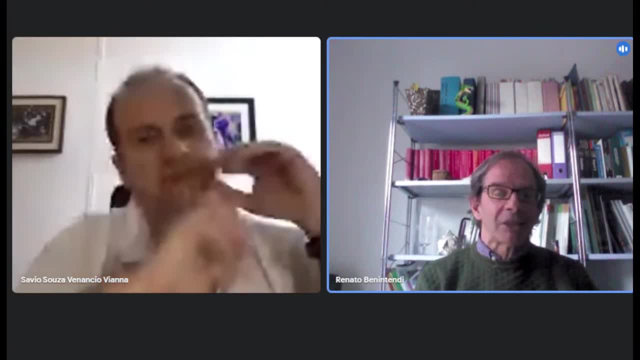 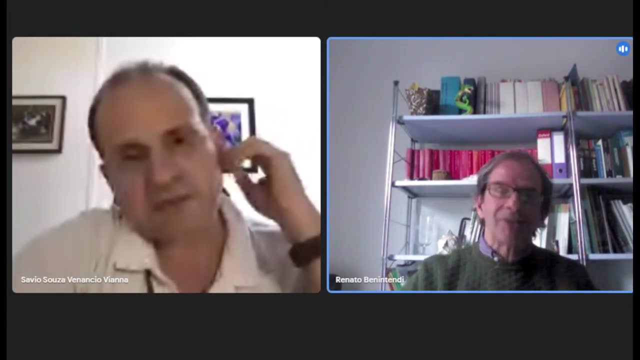 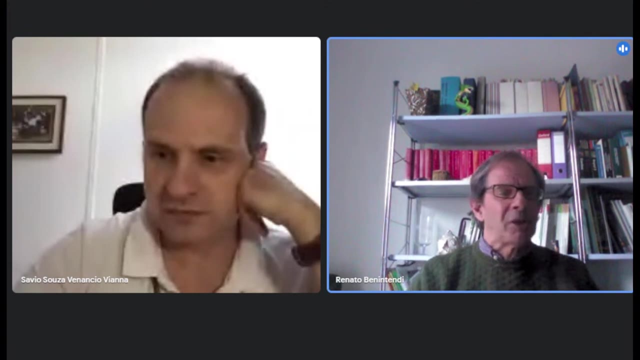 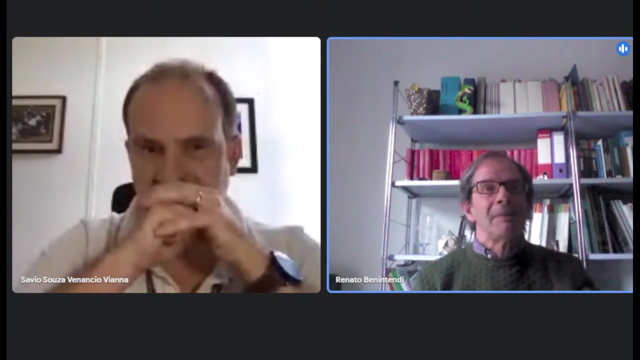 You have rich regulation. Now The material safety data sheet is no longer four-page, three-page, one-page, half-page must be 20 pages because otherwise the Helsinki European Chemical Agency doesn't know to register your chemical. And so this was terrible, because when the rich regulation was implemented, the QSAR, that is essentially the computational toxicity approach- 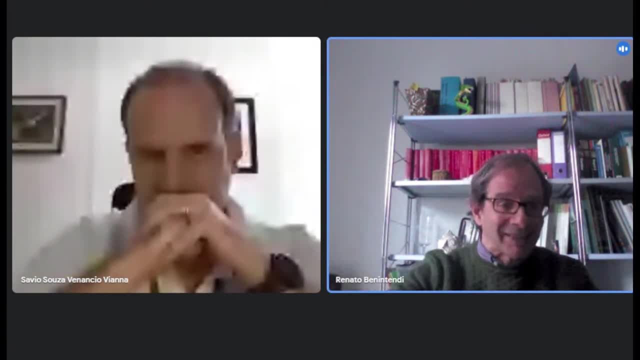 that can replace the in vitro animal test allowed the company not to be involved in an absolutely cost-ineffective research for toxicity. But there was a new rule, So I think that the future of process safety will be comply with the new rules that you have seen- the carbon capture and storage. 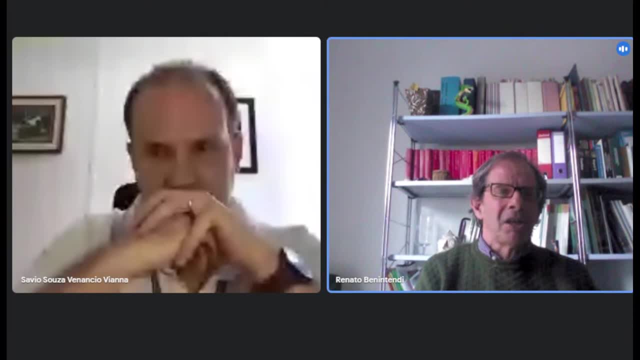 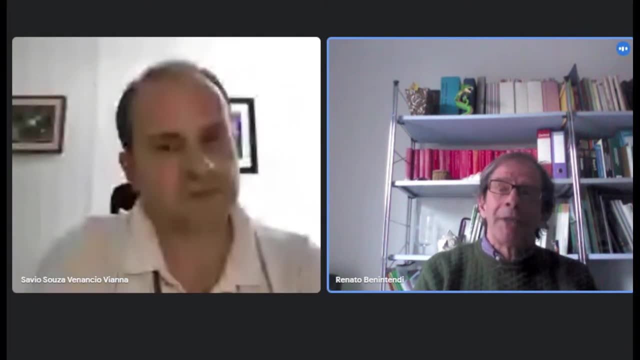 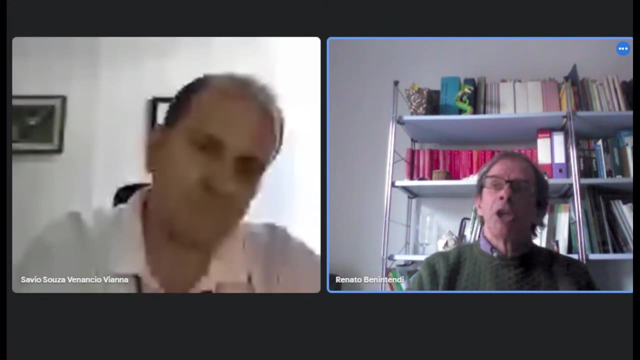 There was 12 million pounds research in China, By 12 million And, what is more, considering that, in reality, the process, safety requirements are more and more demanding, you are forced, in order to comply, just to think in a different way, just in order to comply with the most stringent, stringent rule. 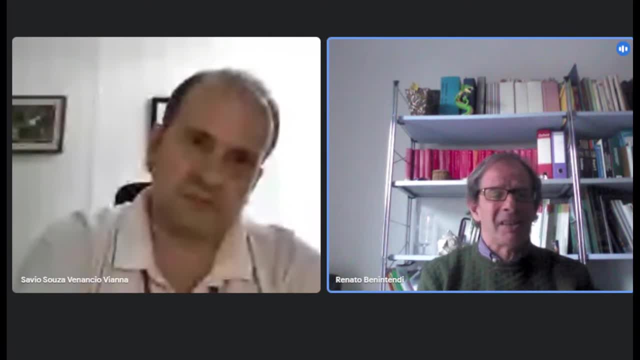 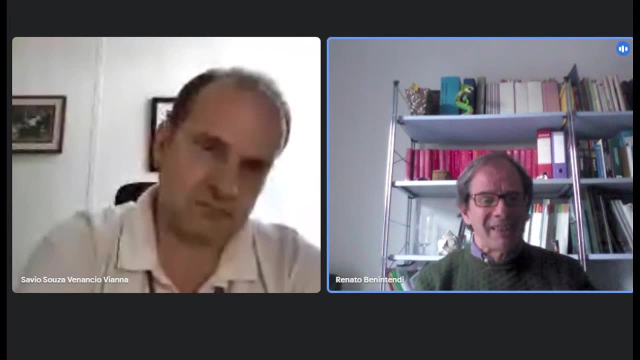 For example, now, now in Europe, we have 10 to minus six per year, So in terms of the acceptable risk. So this means that probably, if you apply the process engineering as it is, You probably are never- never, in my analysis, you are never- in the position to comply with the rules. 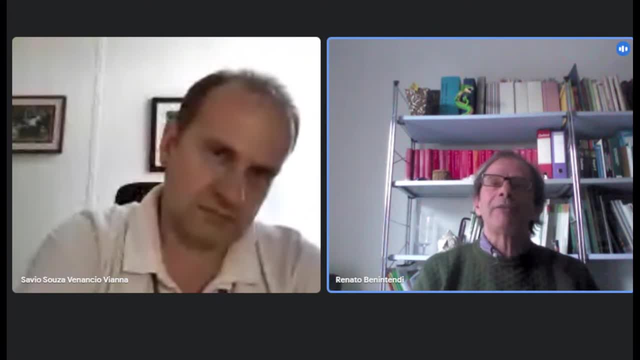 So it means that, in a way or in another way, you have to go to the literature, you have to study, you have to probably just to create a new model, And you have to think in terms of novelty of technology in order to comply. 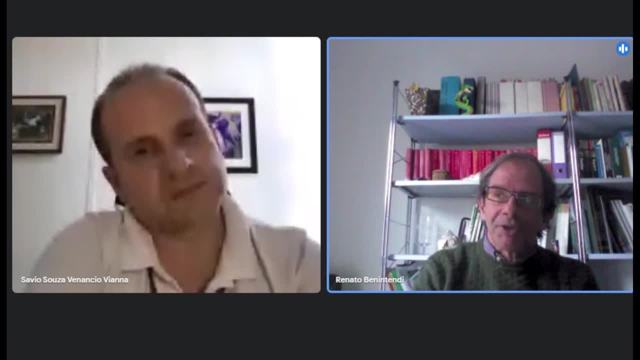 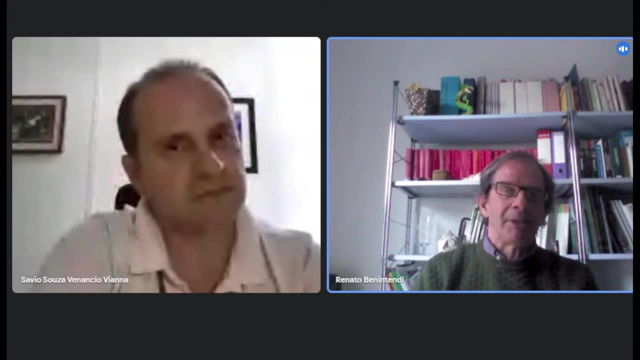 And this is not happening only in Europe. You consider that a very important point. Outside Europe, Now in Middle East, the European regulation is becoming the standard, even if it is not mandatory, but it's becoming the standard. So it's completely trivial that you are not in Europe because the Arabic and the Middle East people say: no, we want that. 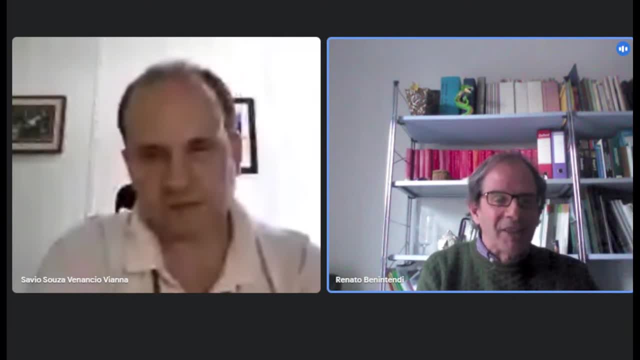 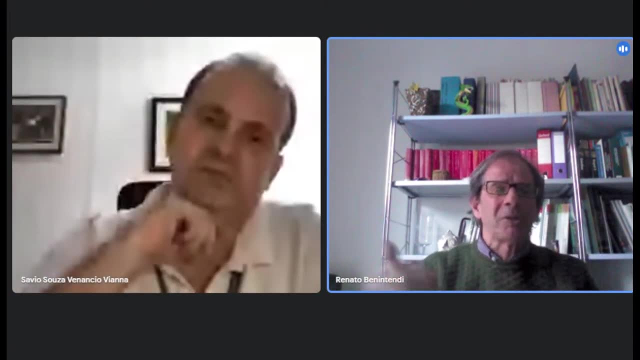 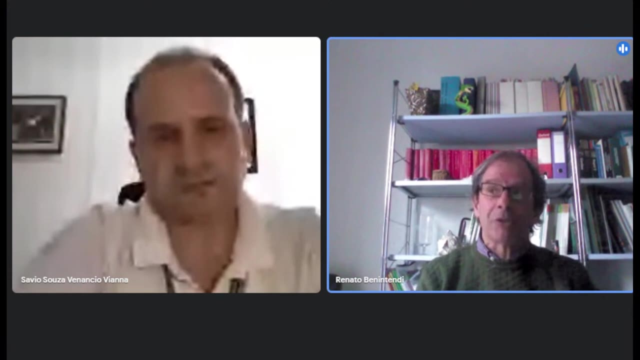 Dust explosion was not in the US. in the US the dust explosion was not exactly included as just a process, safety and regulatory item. In Middle East now dust explosion must be considered And They are using a European regulation, So I would say regulation, new technologies coming from the application and new techniques. 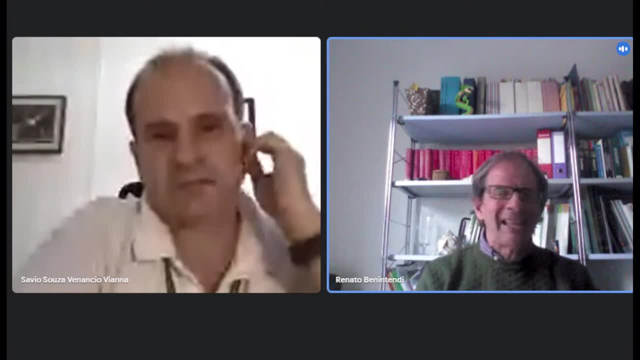 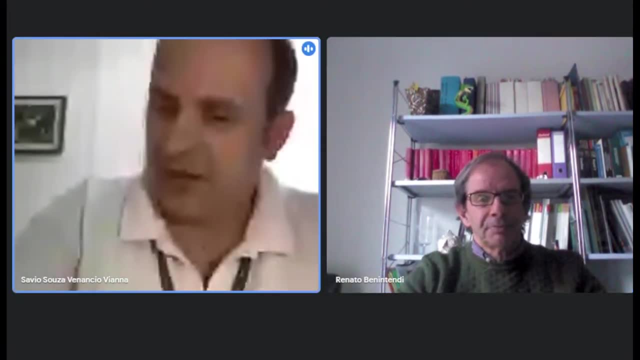 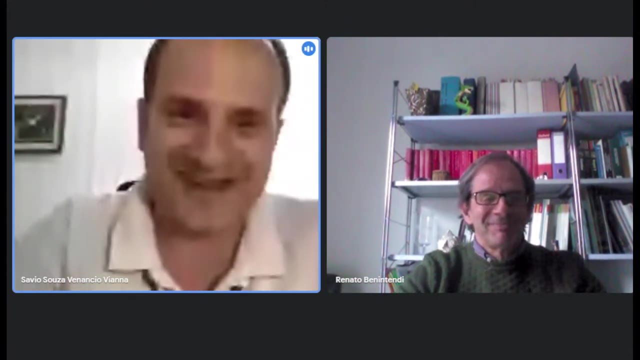 This is producing a completely huge separate research program for process safety engineers. Yeah, yeah, I agree, Renato. it was really a pleasure to have you here. I would love to spend the whole afternoon with you. Yeah, Although it's evening in the UK.